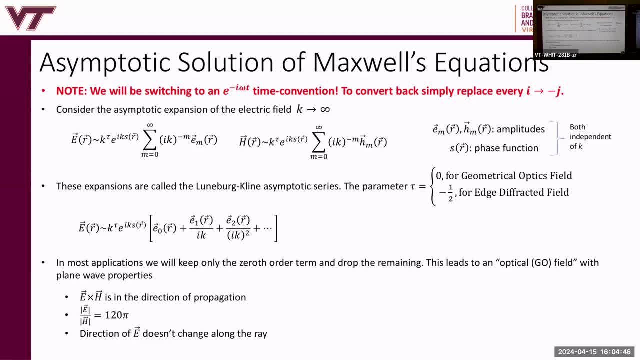 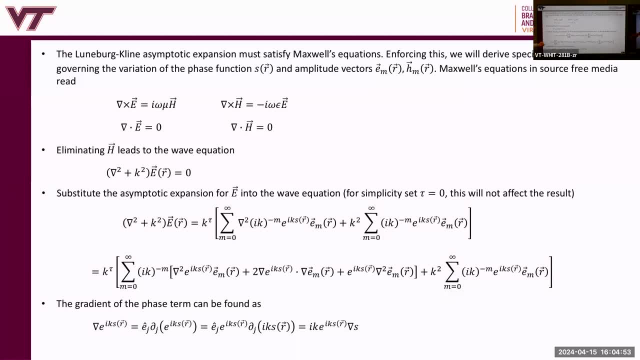 It's an expansion in terms of inverse powers of K right, And we noted Maxwell's equations in the E to the minus I, omega T time convention look like this: We derived the wave equation We substituted in our Lüneburg-Klein expansion into the wave equation and turned the 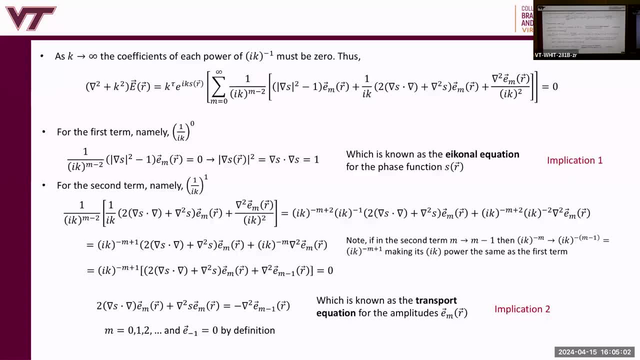 crank, And after doing that we ended up with four implications. The first one that failed out of all, that is called the Eikunnel equation. The Eikunnel equation comes from the wave equation with the asymptotic series expansion substituted in and equating the. what you're supposed to do is equate each power of 1 over IK right, So to the zeroth power. you get the Eikunnel equation. The magnitude of the gradient of S squared is equal to 1.. And the transport equation. 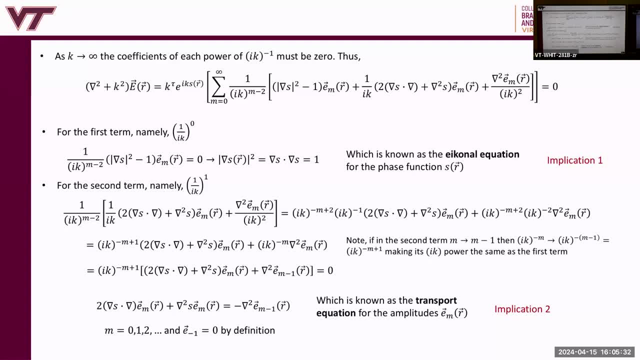 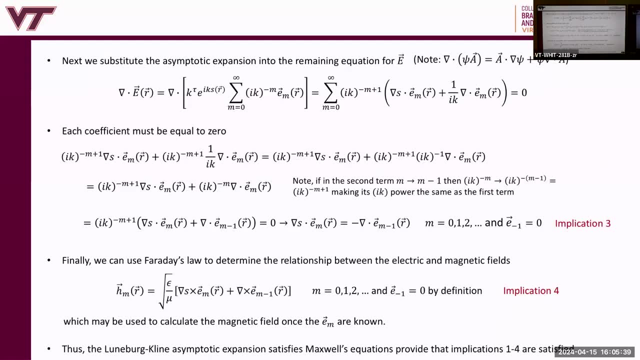 which came out of that. we're going to solve this one today. This one governs the propagation of the amplitudes, And the next equation that came out of that was this one here, which is sort of Gauss's law, right. 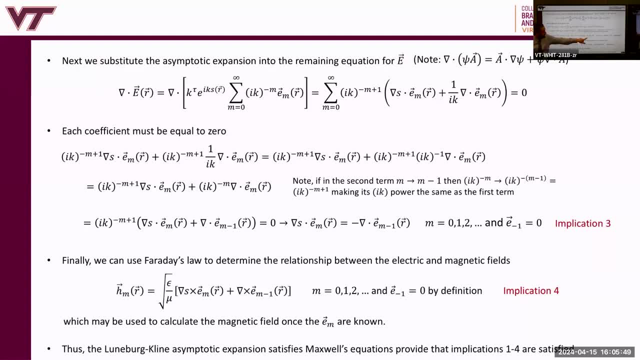 We substituted in the expansion into Gauss's law and we got this third consequence. And here, finally, we substituted in the Lüneburg-Klein expansion for the electric field into Faraday's law and we got this kinetic amplitudes relationship that relates the amplitudes of the magnetic field in terms of the amplitudes of the electric field in the expansion right. 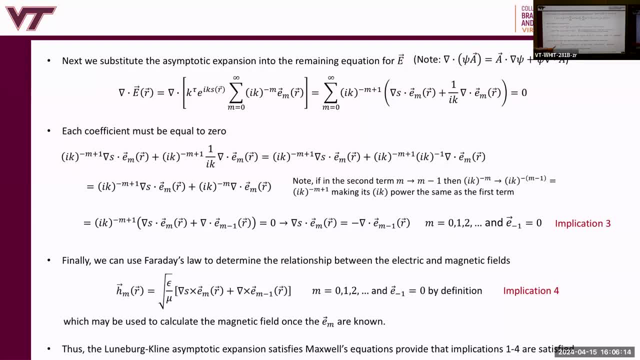 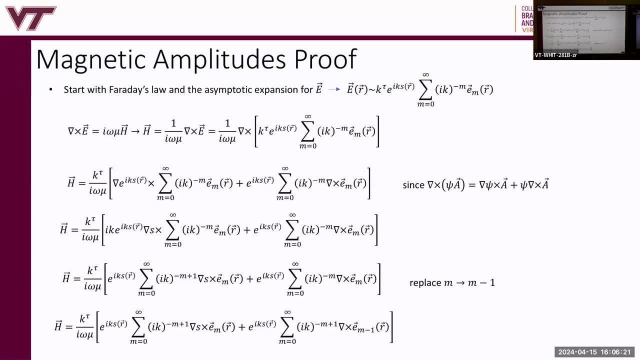 So last time I said that we would dig into this more to see how we got this expression, and that's what I've added to the slides. So here we start with Faraday's law. right, We start with the asymptotic expansion for E and we substitute that into Faraday's law. So in Faraday's law we rearrange it so that it's H equal to 1 over. 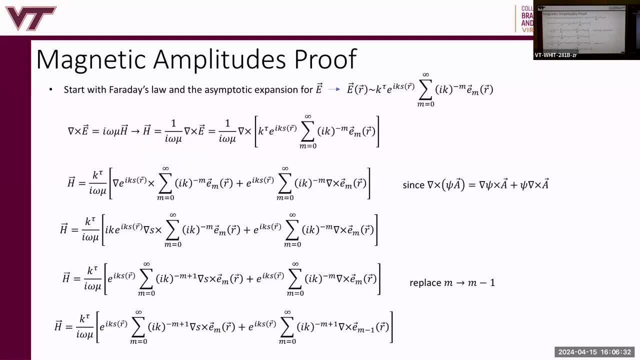 E right. So in Faraday's law we rearrange it so that it's H equal to 1 over O right. i, omega, mu times a curl of e and we substitute in for e the lunenberg clan expansion asymptotic. 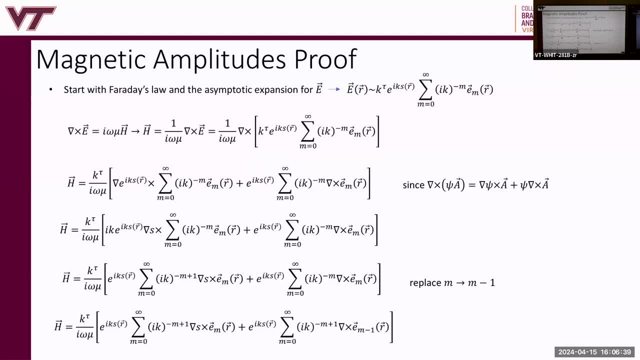 series. right, all right. next we distribute this curl operator. it's actually the curl of a product, so the curl of a scalar times a vector is equal to the gradient to the scalar cross, with a plus psi times the curl of a right. all right, so, all right, so, so that becomes the gradient, so the curl. 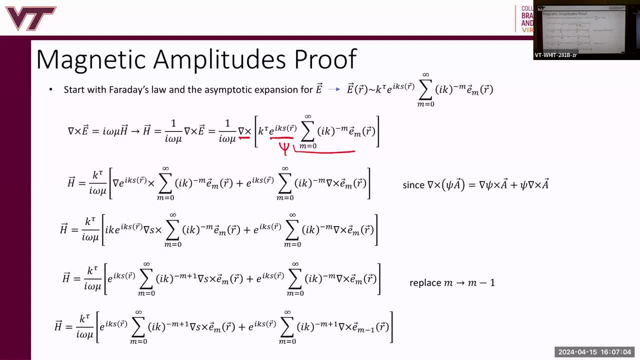 of this is the scalar psi and this whole thing you can treat as the vector a. so that means we get the gradient of psi is here crossed with a, which is this whole thing, this expansion, plus uh sai, which is e to the iks times, a curl of. sigh times the curl of глав to the k of a, plus the relative error ofṭ Church of this49 parentheses. here we get the gradient of ψ, which is the scar of uh, Va and mu limit to the 2 and n ofering each, well as the 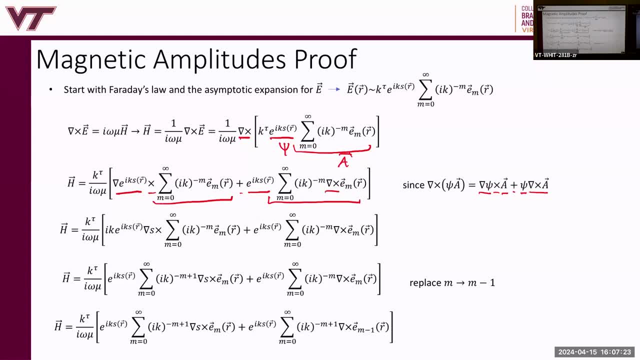 a, which is this, but the curl operator we bring into the summation. all right, good, okay now. what we do is we substitute in what we derived for the gradient of e to the i k s. we did that last lecture that came out to i k e to the i k s times, the gradient of s. right, okay now. and this term is: 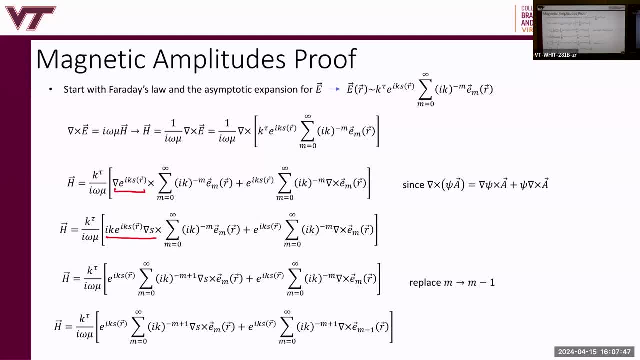 left the same. the next thing we do is, uh, we move this i k into this summation, so m minus m becomes minus m plus one. and we move this gradient of s crossed with inside the summation, because gradient of s does not depend on m. all right now. what we do is we replace, so we want this: i k minus m plus. 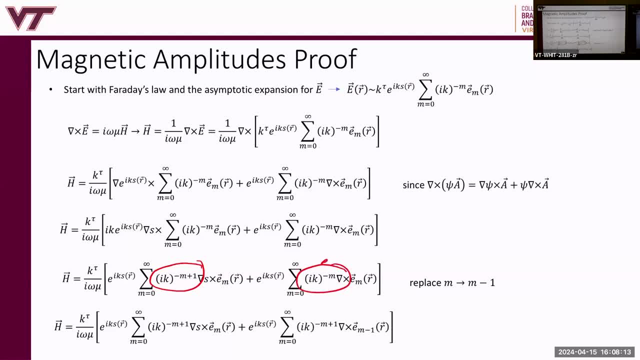 one to be the same as this one, or rather, we want this one to be the same as this one. so what we're going to do is replace m with m minus one in this term, and we get this, but we had to replace this m with m minus one. all right, now this summation starts the same. 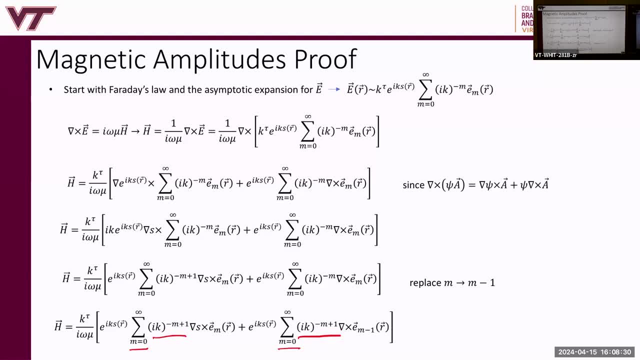 index. they have this same kind of power of the, you know the, uh, the, the polynomial that we're taking with the expansion. with respect, this is kind of like x in a power series. these are all coefficients, right? so this is the series is, in terms of inverse powers of k, all right, so we can. 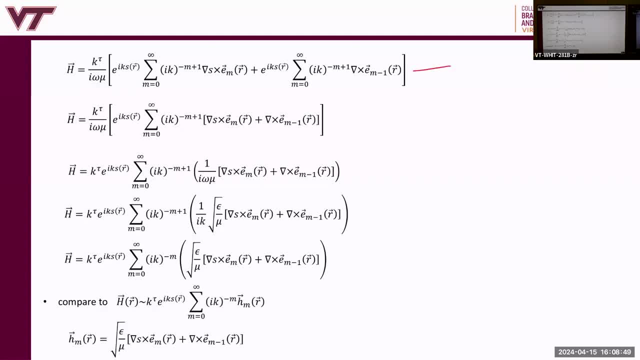 combine those two summations. so that's what we do here. i've repeated this, this calculation, from the last last slide there and uh, now we can combine everything. one summation, one ik to the m plus one, or minus m plus one, and then we have the curl of s cross, or sorry, the gradient of s cross, with e. 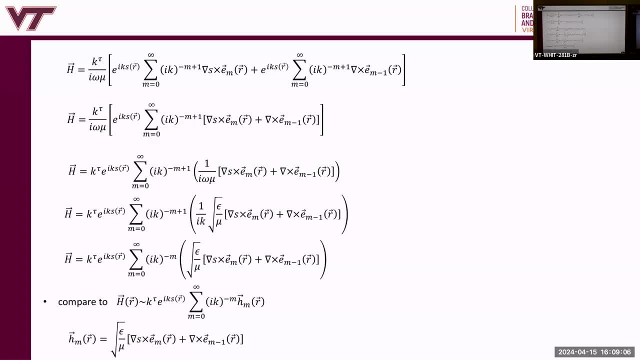 plus the curl of em, minus one. all right, good, so we factor out this: e to the iks. there's a cap or a k to the tau, k to the tau there, and we bring in this, this, uh, i omega mu. we bring it in to this part here. all right, all right, i one over, i omega. 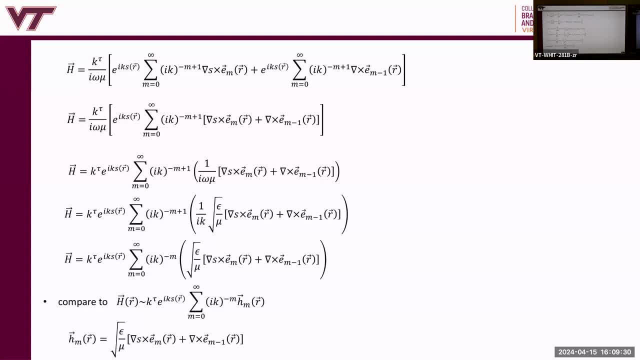 mu is one over k times eta. so let's, let's calculate that. so one divided by i, omega mu equals to one divided by uh i. so the easier way to do it actually is: say one over i k times eta, which is one over i, omega square root, mu, epsilon. multiplied by the square root of mu over epsilon, this becomes one. 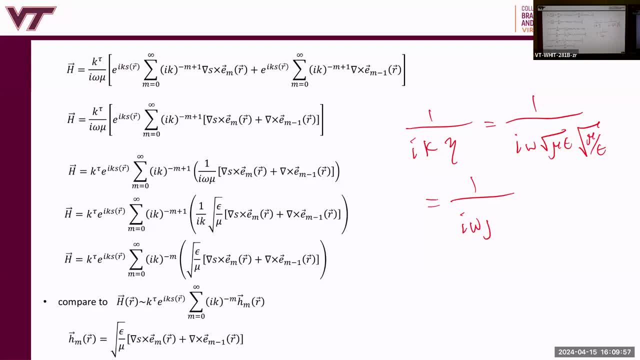 over i, omega and mu. right, so one over i, omega, mu is one over ik, eta. and then what we do is we leave the one over ik there and we write one over eta as the square root of mu, over i k times eta, root of epsilon divided by mu. all right, okay. so this one over ik is ik to the minus one we combine. 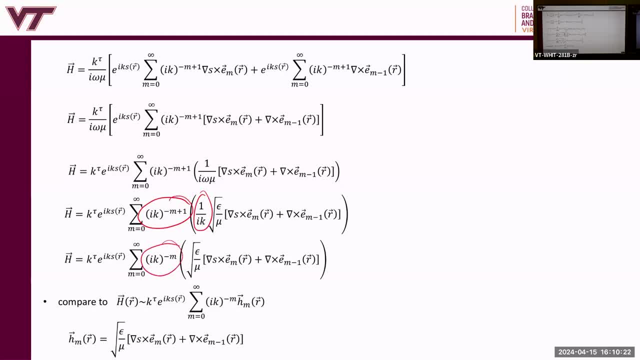 it with this: ik to the minus m plus one to get ik to the minus m. now what we do is we compare this form that we got from faraday's law to the expansion for the h field in terms of the klein expansion, and what we do is we say h is equal to this by comparison. all right, 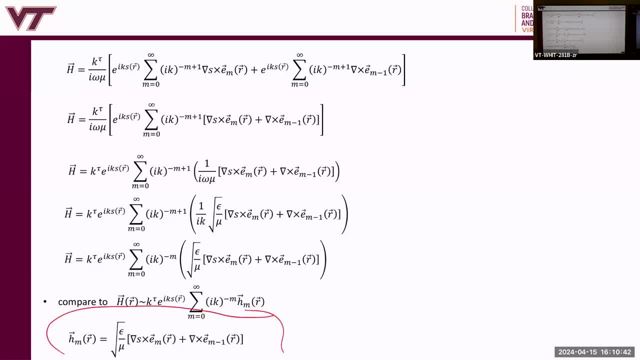 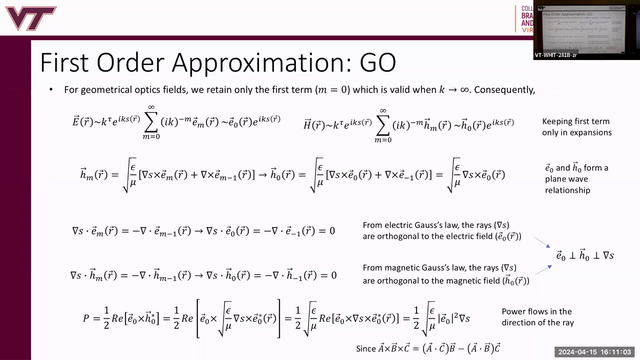 and that's what we get here. yeah, all right, great. so that's how we get the magnetic coefficients. once we have the coefficients for the electric field, all right, great, all right. then we said, uh, we looked at first order approximation, so m equal to zero and that 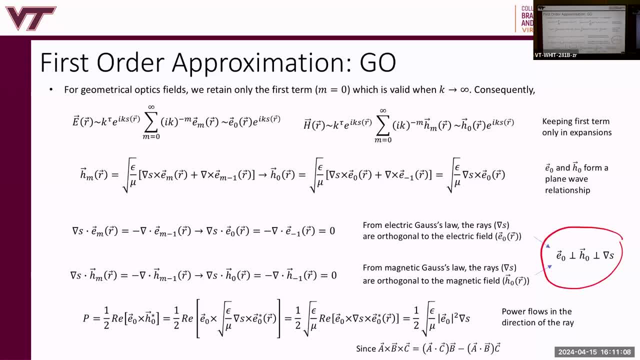 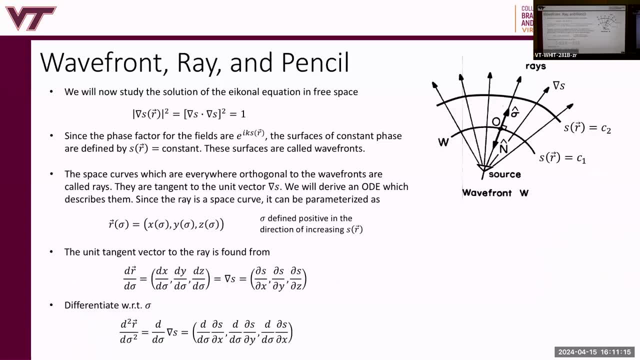 gave us plane wave fields and we found that e and h are orthogonal to the gradient of s, which is the direction of propagation, and that power flows in the direction of the gradient of s. all right, then we went into wavefront ray and pencil coordinates. so then we started to look. 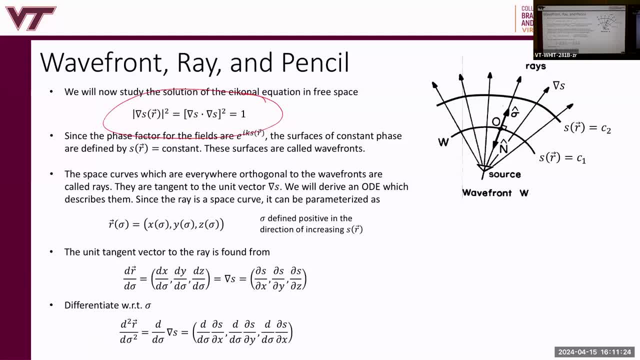 at the solution of the eikonal equation and from there we were able to define, so the ray we can parameterize. with this kind of parameterization we take a derivative of. with respect to sigma, we get the gradient of s right because, dr d, sigma is the tangent to the ray and we said that the rays are orthogonal to the wave fronts. 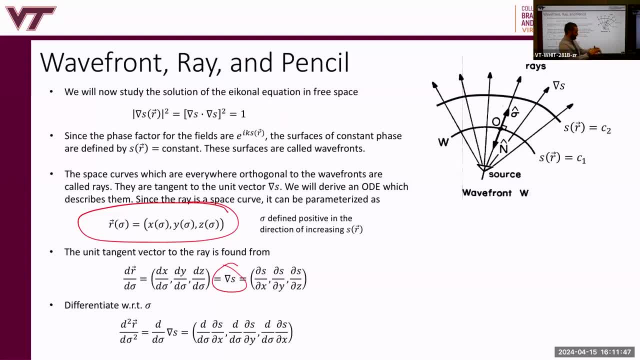 and that the wave fronts act as equiphase surfaces and the gradient of those equiphase surfaces has to be orthogonal to the equiphase surfaces. so it's in the direction of the rays right. all right. so the gradient of s is equal to dr d sigma. 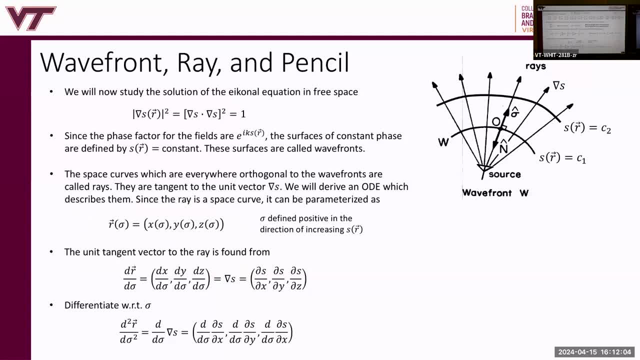 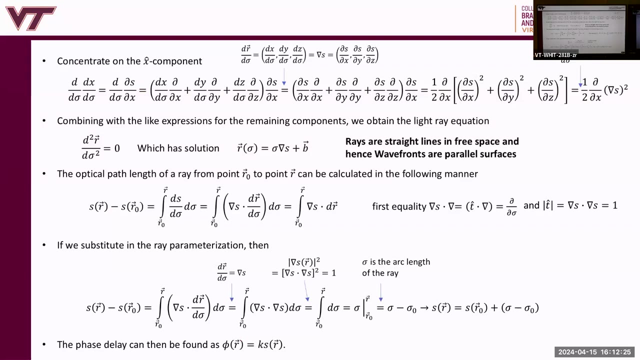 which is also equal to the tangent to the ray. all right, so we, we did, uh, we then um made this relationship here. so then we differentiated again, so we ended up with this expression here. oh okay, so here here we. then we went to this derivation. i looked at this a little bit more. 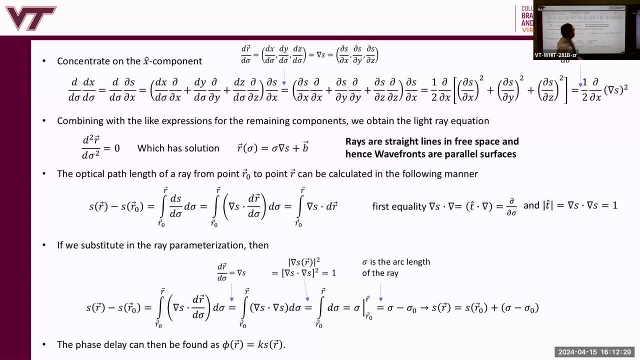 and i know we had some confusion on how we went this step to that step. i think i'm still looking at that, but i think we use this result here as a matter of fact somehow, because we didn't use that result yet anyway. uh, when you solve it, what you get is, uh, this expression here. 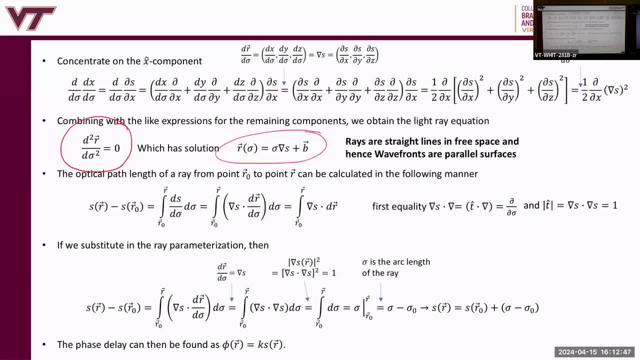 and what that says is that the rays have to be straight lines, right? so the solution to the eikonal equation says that the rays are straight lines in free space. all right, that's important, okay. and then here we also have the equation that says that the rays are: 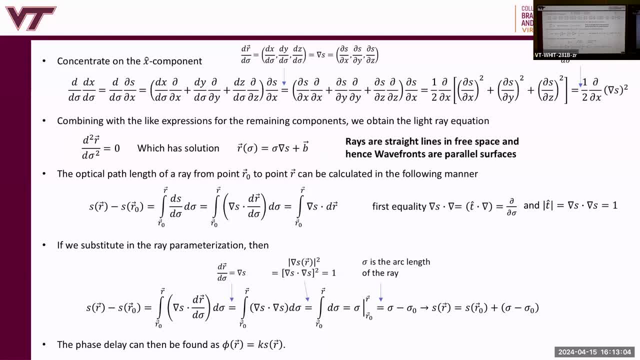 straight lines in free space, right? we also had some- uh, we had some confusion, some questions on how we got this expression here. well, if we look at the gradient of s dotted with the gradient, what does that mean? we can write that as t hat dotted with the gradient, because the gradient of s is equal to a unit vector in the. 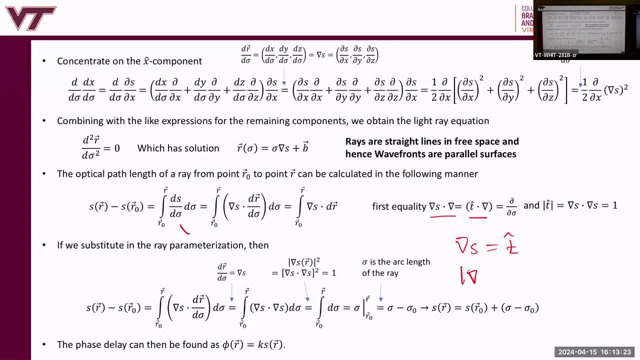 direction of the tangent of the ray. why is that? because the magnitude of gradient of s squared has to equal to one. so that means the gradient of s dotted with the gradient of thegen, gradient of s, equals to one. we know the gradient of s is tangent to the ray, so we can call that t. 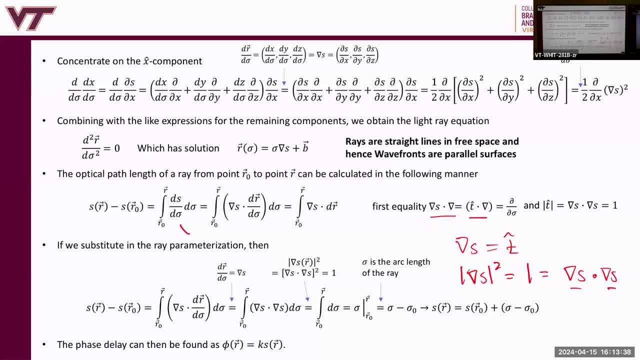 hat. so these, these themselves have to be unit vectors. so the gradient of s, we can say, has a magnitude of one and is a unit vector in the direction of the tangent to the ray. all right, so what that means is the gradient of s dotted with the gradient can be t dotted with the gradient. 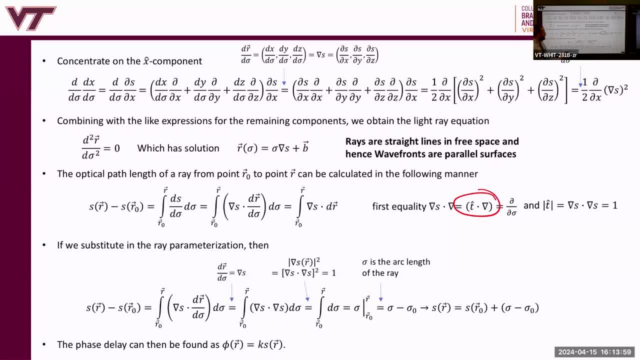 what is t dotted with the gradient? i have a gradient of some. it's an operator, first off. so is this gradient of s dot with the gradient right? it's an operator it has. it doesn't tell you what function you're applying this, this uh vector calculus or this differential operator, to right. 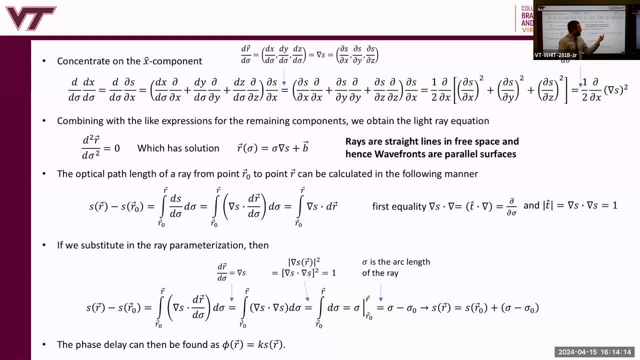 but uh, this is also an operator, the gradient, right. so we're taking the gradient of some function wherever we apply this operator to scalar function. and when we uh take the dot product with t hat, what does that mean for this gradient operator and the direction of it's? like directional derivative. it's very, very good, it's a directional. 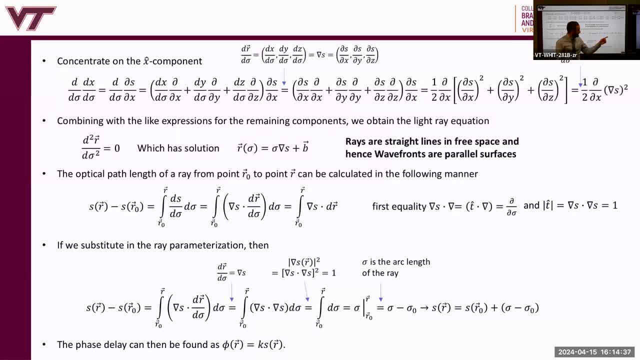 derivative in the direction of the unit vector t right. so it's a derivative of the direction of the ray which is d by d sigma or partial by partial sigma fuel. all right, these are these little identities that you need to know when you're we're doing these derivations, so that 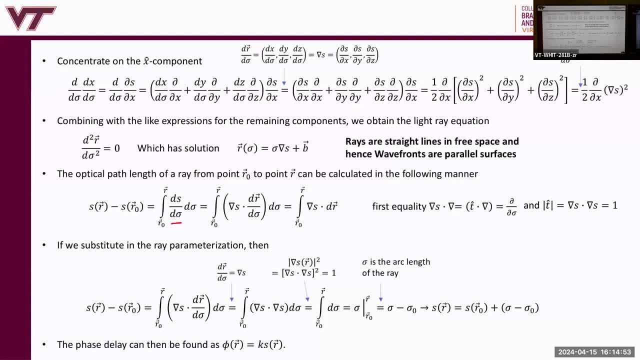 means that the uh ds by d sigma here is nothing but uh. so now we're going to do this derivative, now we're applying this d by d sigma, which is this, to the scalar function s. all right, and what that means is we're taking the tangential derivative or the directional. 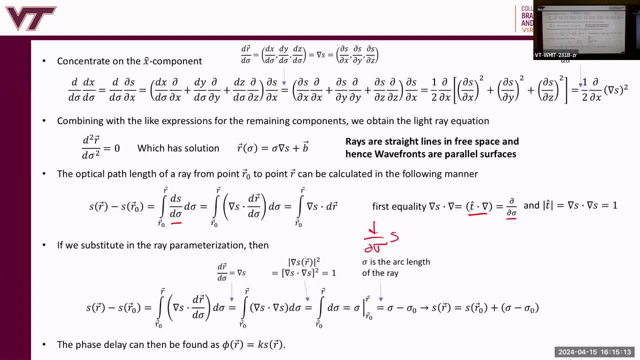 derivative in the of the wavefront surface in the direction of the ray, which is nothing but the tangent vector to the ray. right, we're integrating the tangent to the ray to calculate the arc length. all right, so we just said that we can replace partial or d by d sigma, here with the gradient of s, dotted with the gradient of s. 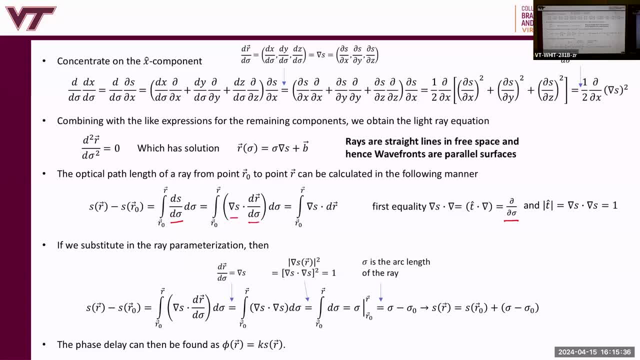 basically, right, the gradient of s dotted with uh, because dr d sigma is the gradient of s. all right, yeah, there's a lot here. right, there are a lot of derivations, but you guys will need the final results. we need to understand the derivations, right? if you want to do anything with this theory and later on, right okay. 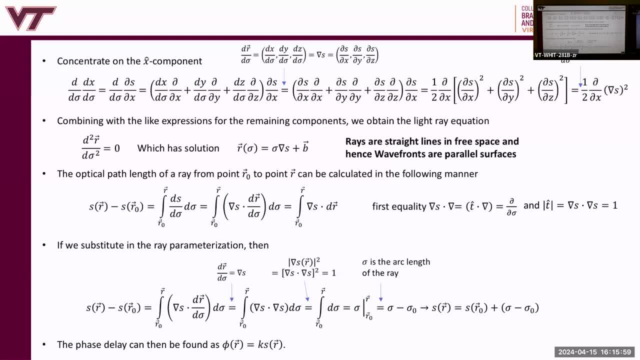 so great, so you cancel these d sigmas and what we find is that we can find the phase delay along two points along a ray. so the difference between the optical path length at some point r naught and that at r, by integrating from r naught to r this quantity, the gradient of s dotted with dr d sigma. 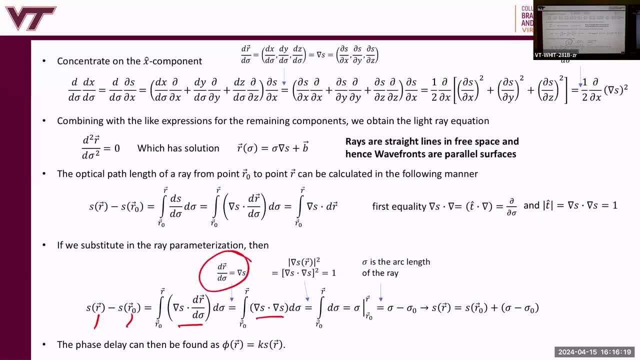 but we know that dr d sigma is the gradient of s. so the gradient of s dotted with the gradient of s, and we know by the eichmann equation that this is just equal to one. so we just get the integration of the arc length of the ray, right, you just integrate, we're not integrating any. 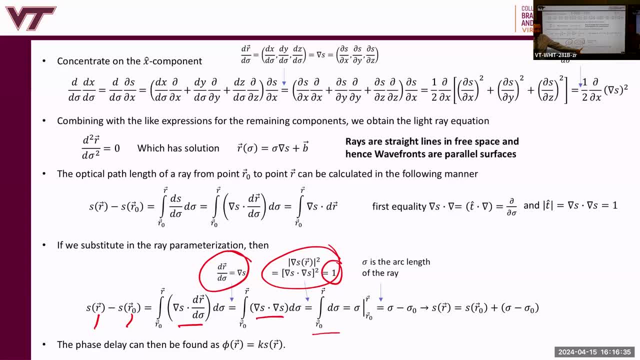 function along that line, integral, right, we're just integrating. you know how, if you integrate uh in spherical coordinates, if you integrate from zero to pi and then from zero to two pi and you just integrate ds, you're not integrating any function over those, those limits, just you're. 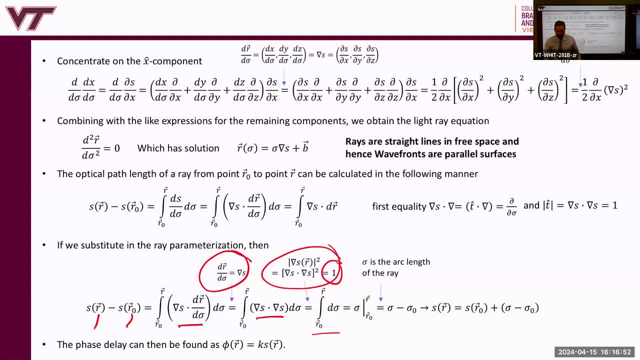 evaluating basically the function one for those limits. you're calculating the surface area, right? so this is the integrating the arc length, all right now you might ask: well, why do you have to do all of these? you know these different relations or gymnastics, to get to this result, which is kind of obvious. for this, 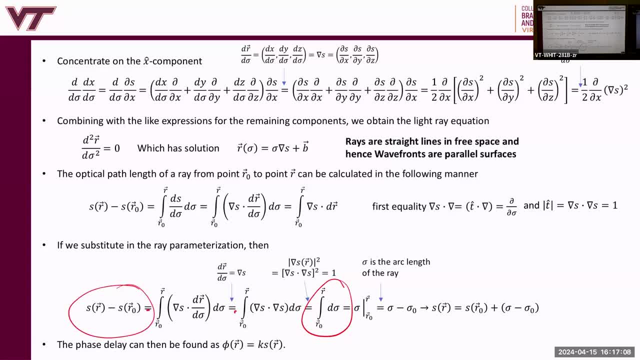 uh, but in in homogeneous media or media. that's not free space. even this, you have to follow these steps because it's not just this. you have to integrate the index of refraction along the ray. all right, so there's another scalar in homogeneous media, or in homogeneous media. then you have 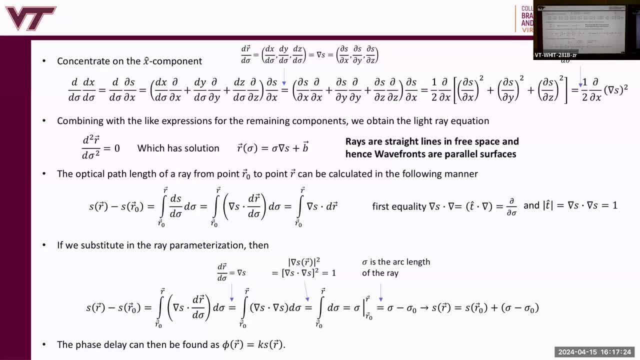 an integral that has a function, that's a function of the position in the medium or the arc length to the index of refraction. okay, so you get this following result right, and this is kind of obvious, right. so the optical path length at some point r is equal. 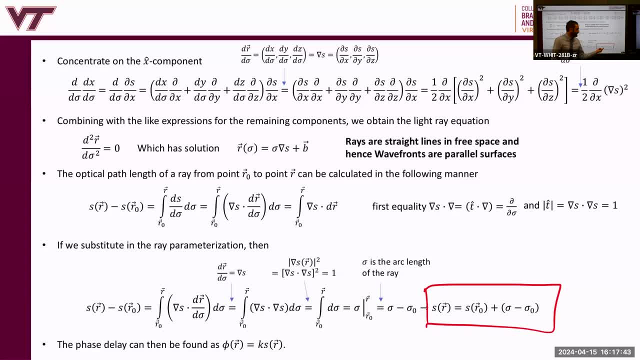 to the optical path length. at some point, r naught plus the arc length from r naught to r- right, okay, that that's important because once you have the optical path length, you can calculate the phase delay along the ray, which is what you need to do when you trace rays. 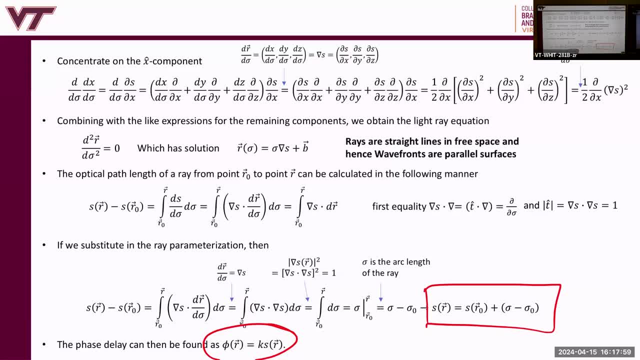 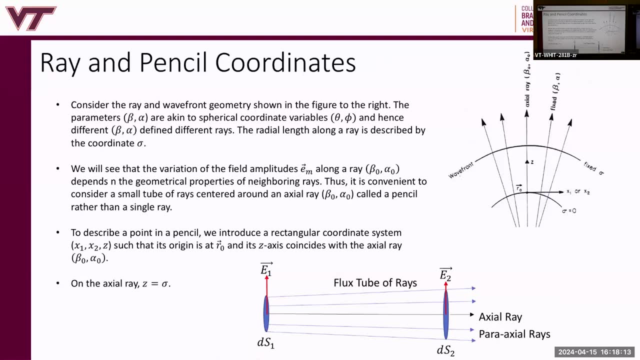 you need to know the amplitude change from point a to b and the phase change from point a to b and the polarization too, if it rotates. but in this, in the media that we're going to study, it does not all right. so you multiply by k, okay, so we solved the eikonel equation right when we 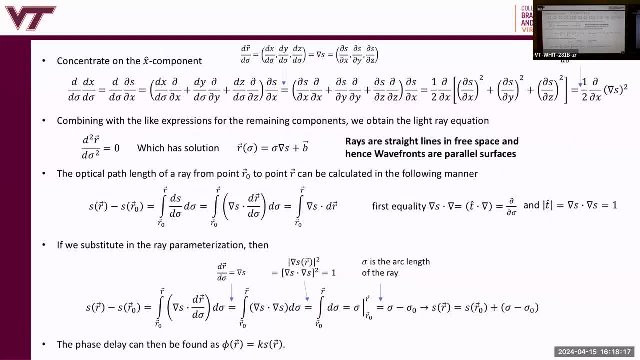 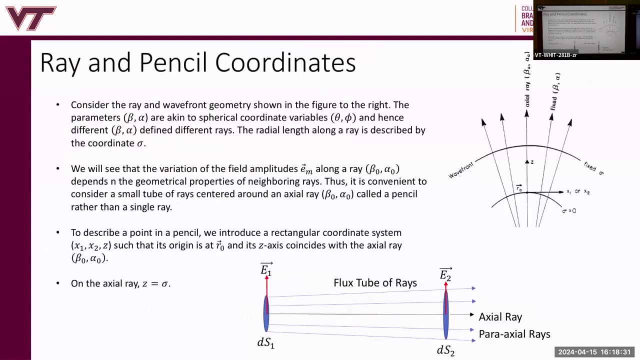 solve the eikonel equation. what did we get? we got this following differential equation: right, this is the solution to the eikonel equation, which shows that the rays are straight. okay, good, all right, now we'll solve the transport equation very shortly, so let's talk about ray and pencil. 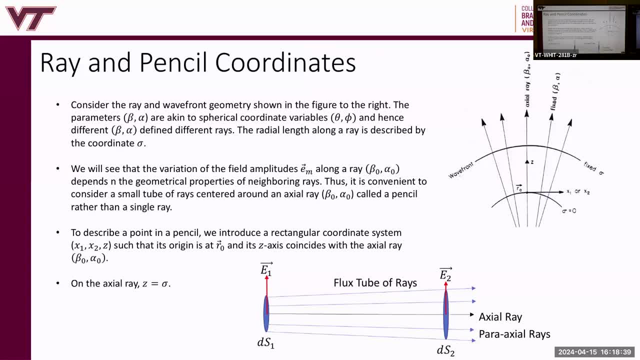 coordinates. consider the ray and wavefront geometry shown in the figure to the right. so we have wavefronts here. here's a wavefront. here's a wavefront, and this one's, at sigma, equals to zero, and this is at some fixed sigma. all right, the parameter is beta and alpha, so there. 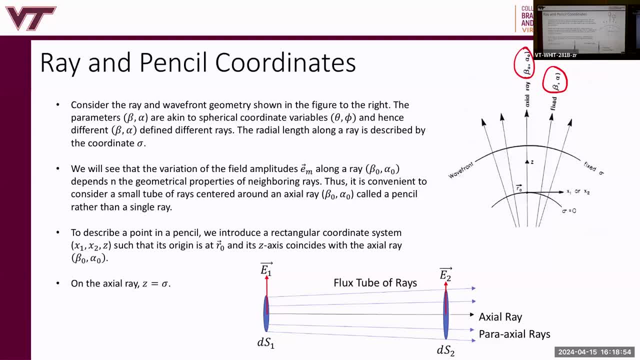 are two parameters here, beta and alpha, and there's a beta naught and alpha naught. beta and alpha are like the spherical coordinate variables, so what they do is a particular beta and alpha put you on a particular ray right. think of beta as theta and alpha as phi. all right, 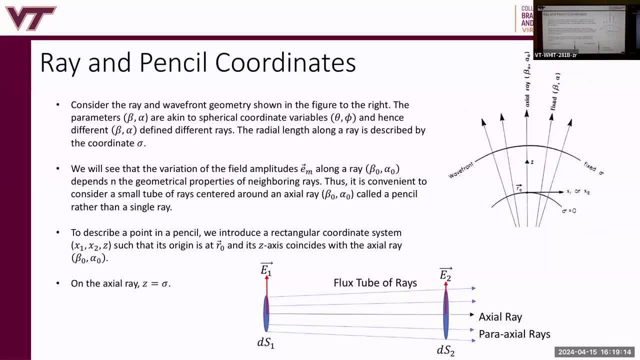 okay, they're akin to the spherical coordinates and for different beta and alpha, define different rays. we're not going to use this alpha beta coordinate system, this ray fixed coordinate system, very often here, but we will in diffraction, when we get to diffraction, all right, the radial length along a ray is described by the coordinate sigma. so a different beta and alpha. 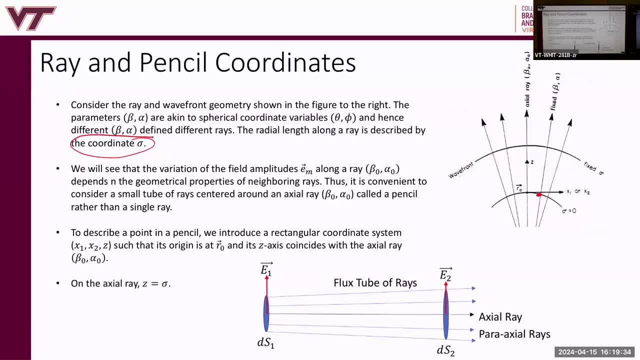 puts you on a different ray. so okay, think of it like this: theta is, let's say, in this particular figure. we could say that: so the z-axis is there right? here's the z-axis. here's a point r naught right, this point here and these directions. here is either x1 or x2, which could be the principal. 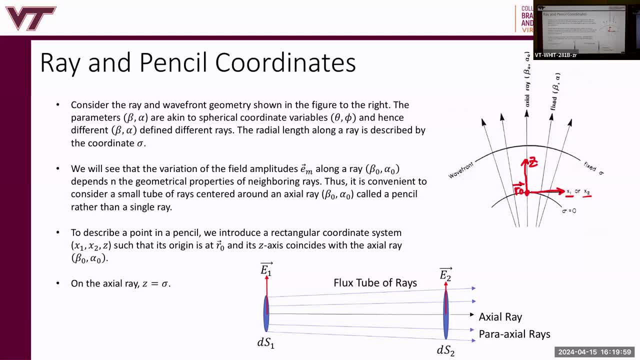 directions right, all right and okay. so if this is the z-axis, then this direction is the angle beta and it should be akin to theta. right, theta is the angle measure from the z-axis. phi puts us in and out of the board right, so at? phi equals to zero. for example, we could be: 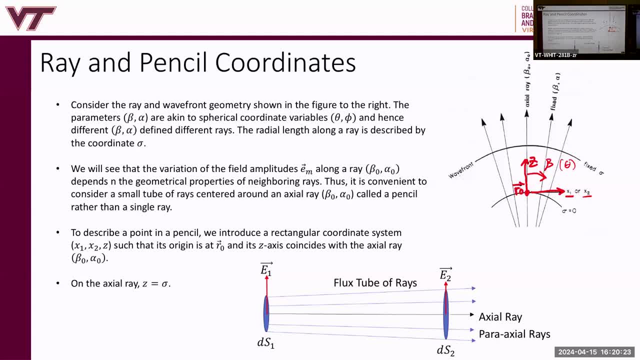 um, if this axis were x1 and the plane of the board is z and x1, then phi would be zero in this plane, right, okay, so you can imagine how different data and phi put you on different rays, right okay. and along the, along the z direction. 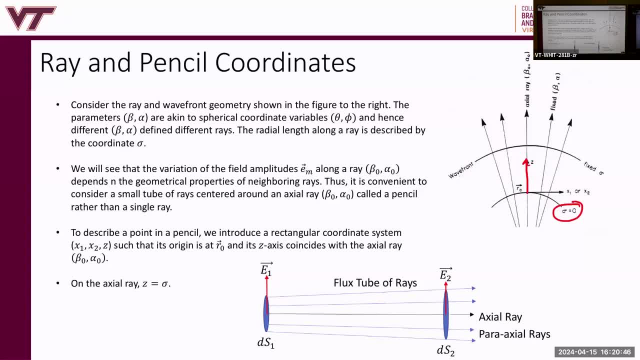 along a given ray. we measure the arc length in terms of the radial length of the ray is sigma, all right, okay, all right, we will see that the variation of the field amplitudes the ems along a ray there. okay, so there are different rays here? there are. there's one ray which is 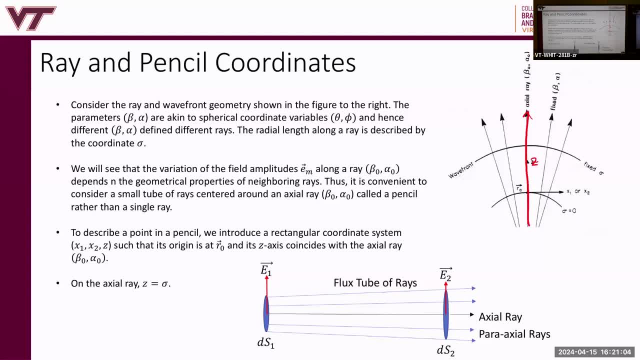 called the axial ray, the axial rays in the z direction, and it has beta naught, alpha naught as its ray coordinates, all right. all the other rays are called paraxial rays and they have different beta and alpha, all right. so we will see that the variation, the field, amplitude, the 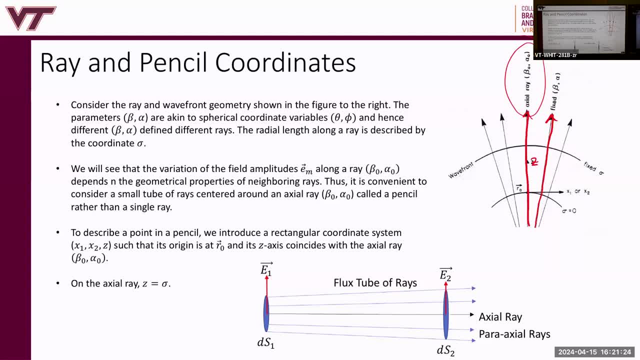 long array or an axial rate depends on the geometrical properties of neighboring rays. so we can't determine the amplitude by uh by uh, considering only a single ray right, we need to use a few neighboring rays. we call all those neighboring rays a flux tube of rays. so you have some axial ray here and you have a number of paraxial rays. 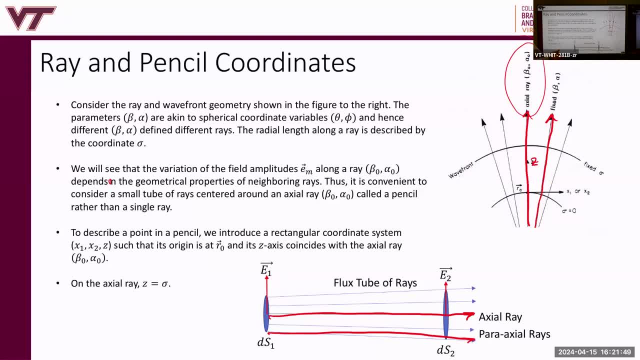 that surround that axial ray and create a tube of rays. all right, so you know. one time i always think of this thing is whenever i'm taking a shower. we have the shower head that has, like, the little streams that come out of it. there's a bunch of holes in it and everything that comes out of it looks exactly like this. 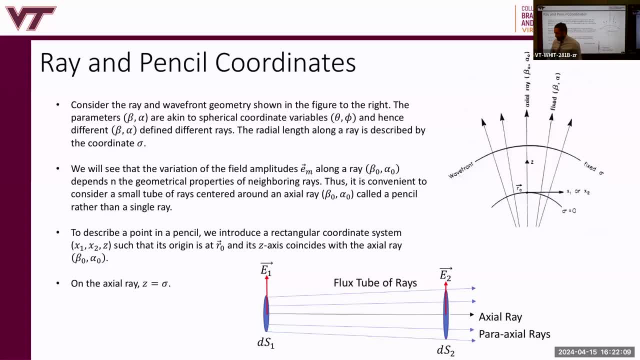 tube of rays. so there's a stream and then there are surrounding streams, and so you can kind of picture it like that, right? so, uh, a little tube of rays, all right. consider a small tube of rays centered around the axial ray. we call that a pencil. all right, so instead of a single ray now, 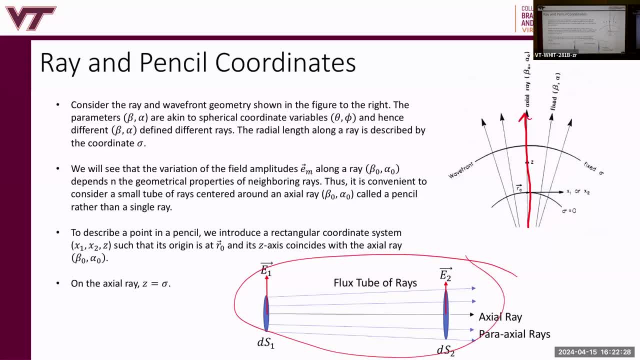 we consider a small tube of rays and we call those tube arrays a pencil, a ray pencil. okay, so describe a point. to describe a point in the pencil, we introduce a rectangular coordinate system, so x1, x2 and z. here's x1, x2 and z, such that its origin is at r, naught right here, and 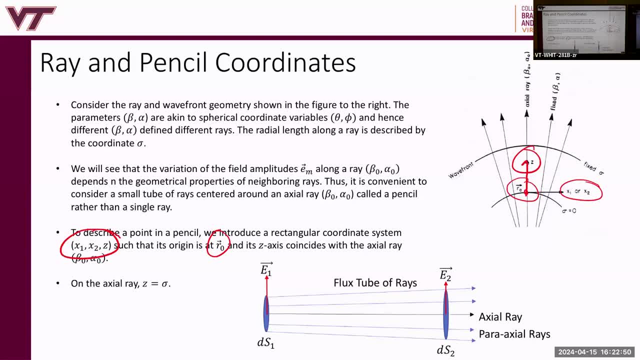 its z-axis coincides with the axial ray, which is described by beta naught, alpha, naught for the ray coordinates. okay, on the axial ray, z is akin to sigma. all right, of course, on the axial ray only. that's the key, all right. so let's start to add some differential geometry to this. yeah, 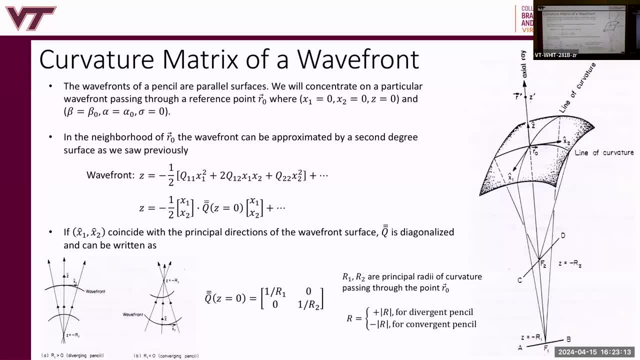 so the wavefront, the wavefronts of a pencil are parallel surfaces. why are they parallel surfaces? so you guys remember, it has to do the icon equation right. you know, they are orthogonal to the, the waveform, the rays are orthogonal to the wavefronts. and what do we? what do we know about? 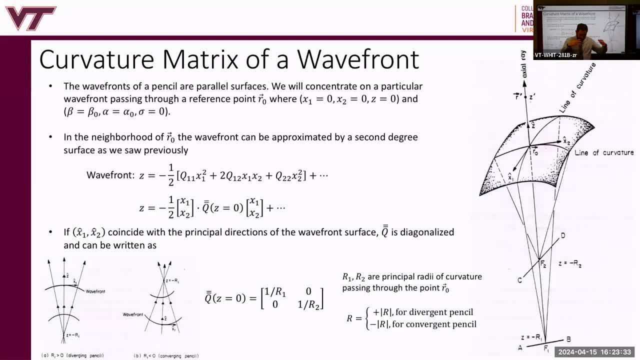 the rays. they're straight lines, so the wavefront surfaces have to be parallel, right? okay, good, so they're parallel surfaces. we will concentrate on a particular wavefront, passing through a reference point, r naught, where the coordinates, the pencil coordinates, x1, equal to zero, x2 equal to zero, and 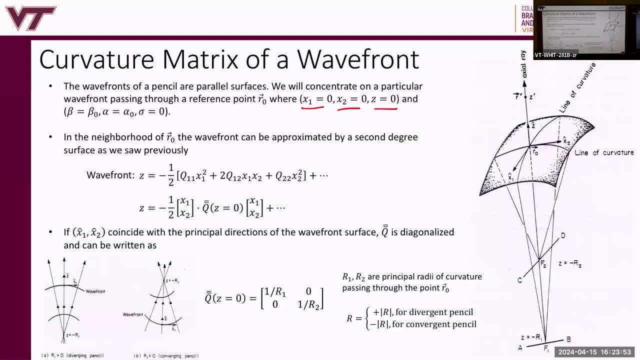 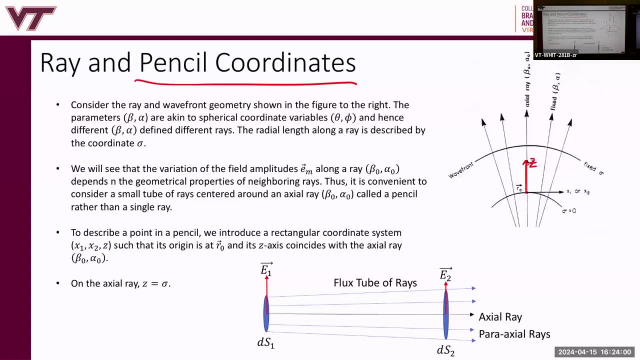 z equal to zero. remember, we're now working in these pencil coordinates. the pencil coordinates are uh, z and x1 and x2. x1 is we're talking about x2, okay, so in the pencil coordinates the point r naught here in the x1, x2, z coordinate system. 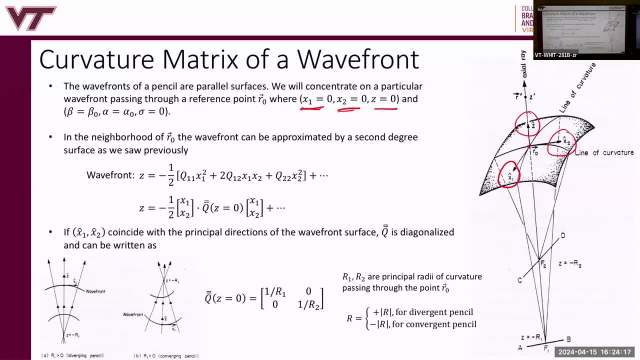 have x- naught one, or x1 equal to zero, x2 equal to zero and z equal to zero. okay, and we have beta equal to beta naught, alpha equal to alpha naught and sigma equal to zero. which one of these is the pencil coordinates? which one of these two is pencil coordinates? 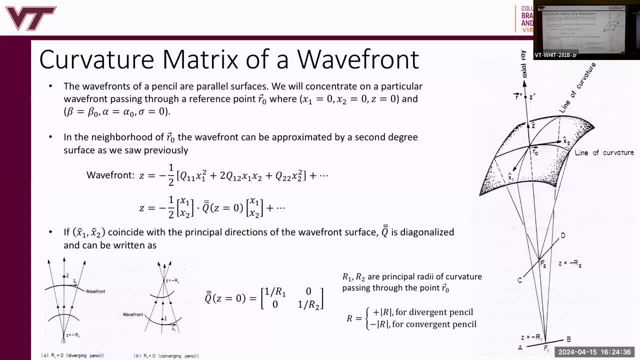 okay, so you have two coordinate sets here, right? x1, x2 and z. and then you have beta, alpha and sigma. which one of these is the pencil coordinates and which one is the ray coordinates? which one? which one is this pencil pencil coordinates? yeah, that's right. pencil coordinates are x1, x2 and z. 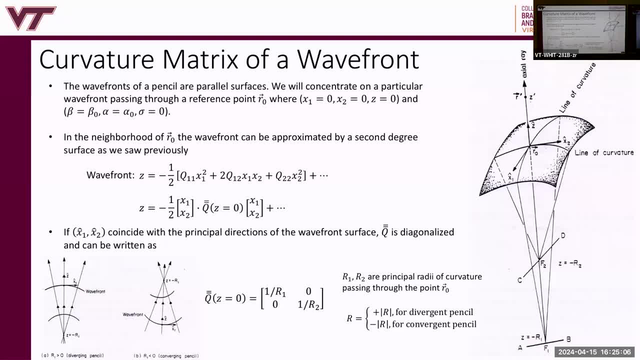 the ray coordinates are beta, alpha and sigma. okay, in the neighborhood of r naught. so in a small neighborhood about this point, r naught, the wavefront can be a proxy approximated by a second degree surface, as we saw previously. so this wavefront here, this wavefront here, 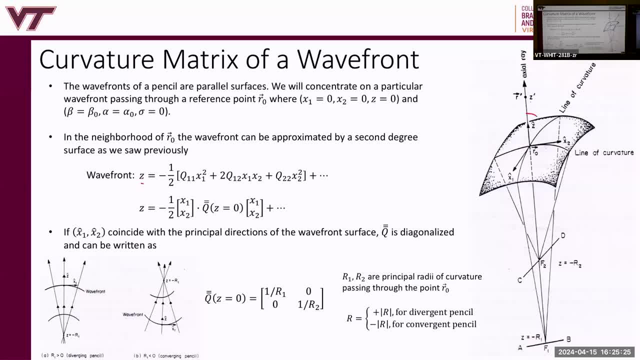 we can approximate that wavefront as z because it's in this coordinates, right. so z is the distance off of this x1, x2 plane, tangent plane to the wavefront at r naught, all right, so we're going to draw a surface. so we have some coordinates: x1, x2 and there's z. 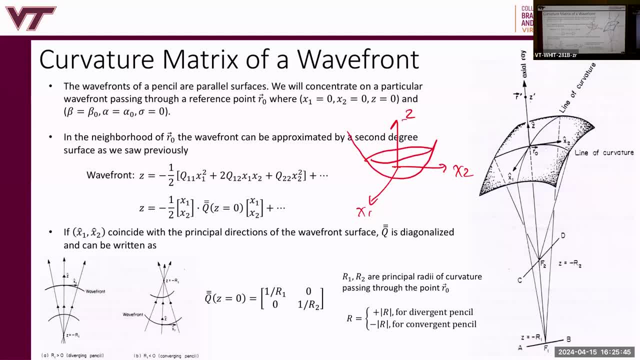 so we're going to draw some surface here, and this surface is described as: z equals to a function of x1 and x2 right. all right locally in the neighborhood of r naught. so z is equal to all right minus one half: q11 x1 squared plus 2q12 x1- x2 plus q22 x2 squared. 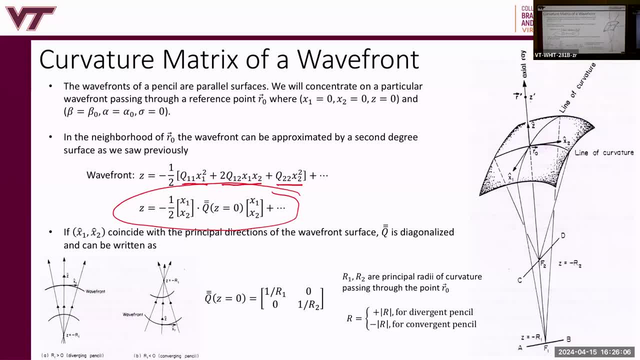 and in matrix notation. is this right? do you remember how we got that? it's been a couple of days, right. you remember how we got this? this is the approximation of a surface. oh, you know taylor series of equations. you know taylor series of equations- expansion: we kept only second order terms. 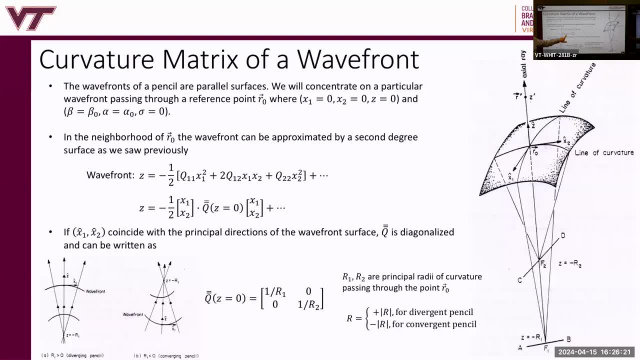 and we were able to derive that we can describe it in terms of the q matrix of the wavefronts as a surface right? why is it negative if you go back to our approximation of a surface? see if i can find that if you go back to the approximation of a surface here, 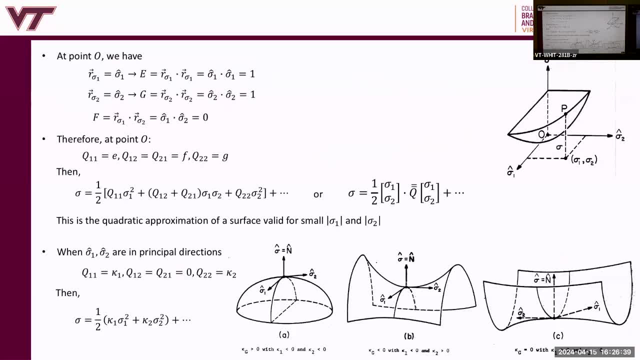 we said that we can describe a surface like this right, but it's not negative. and remember, here's now it's x1, x2, but this was sigma 1, sigma 2 and then sigma, and we described the surface sigma, the height off of the sigma 1, sigma 2 plane, using the q matrix, which describes the curvatures of 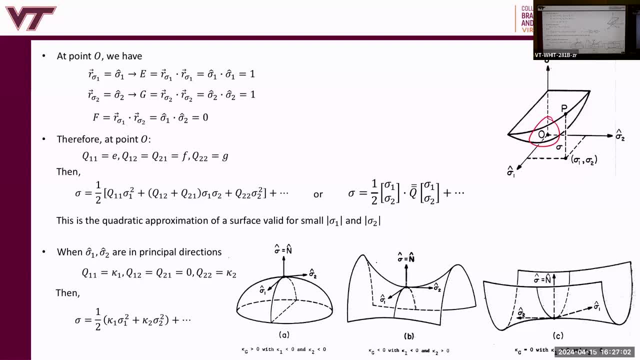 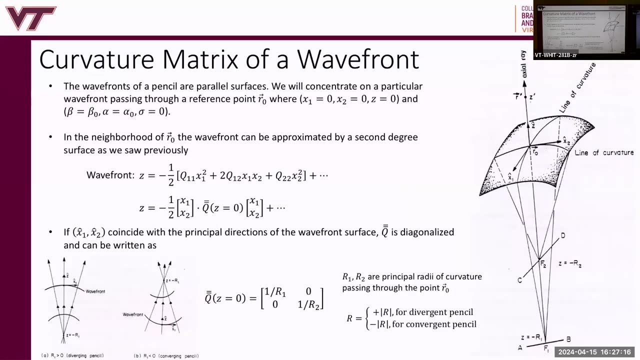 this surface locally about the point at the origin. but this one's positive, right? so why then see if i can get back to the side we're at? uh, why is this one negative? because it's not convex or very good, it's curving away from the coordinate system, right? 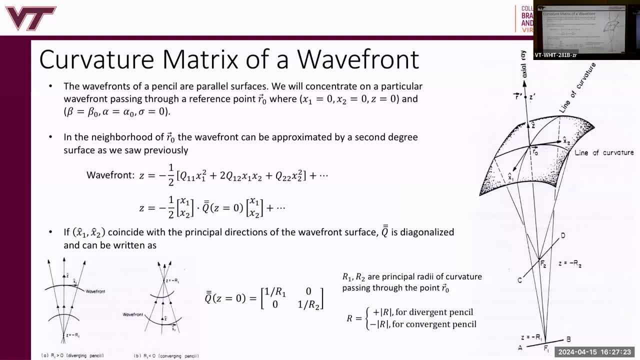 so it's negative. all right, all right. so so you start with the q matrix at z, equal to zero at this point of this surface right and uh. from that q matrix you're able to multiply by x1, x2, the displacement along these axis, axes x1 and x2, and you can calculate. 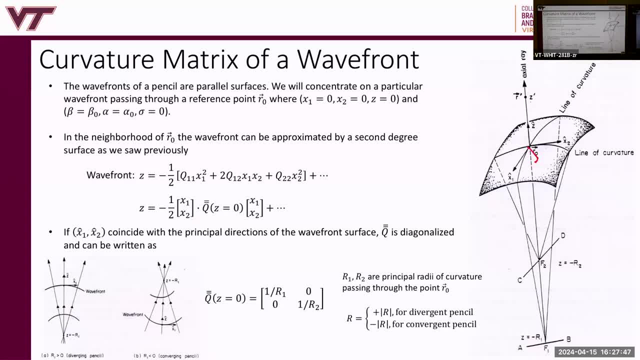 the height, depending on how far you move, what point you pick in this tangent plane as as x1 and x2, and then from here you can go up and find the height. i guess it's going down and in this particular situation, right, all right, good, so that should be cool. what this? this is a very 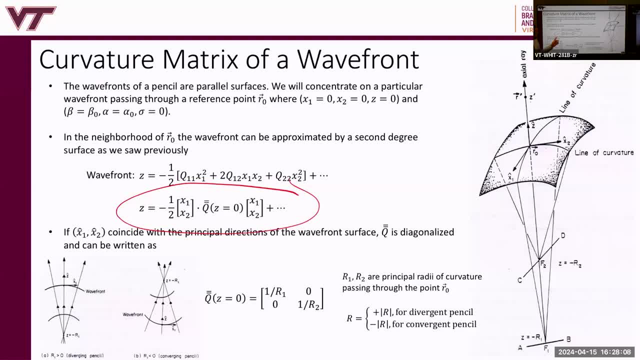 interesting function, right, or an interesting uh equation. what this says is: i can approximate. if i know the q matrix of the wavefront surface at the point r naught, then i can describe this entire surface locally around that point r naught using the q matrix at. 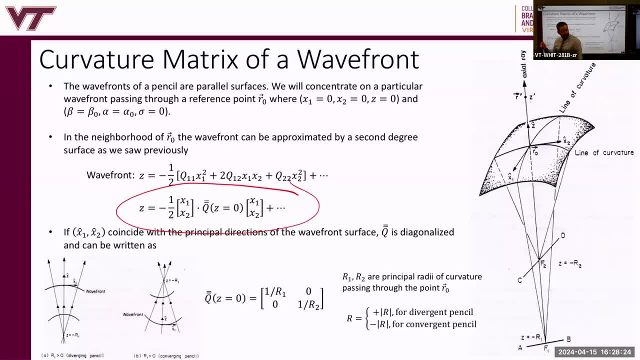 the origin with this expression. right, very cool, all right. so if x1 and x2 coincide with the principal directions, what do we know about the q matrix? i guess i wrote it already: it's diagonalized, right. the principal directions are eigenvectors of q, so then they diagonalize it, all right, good. 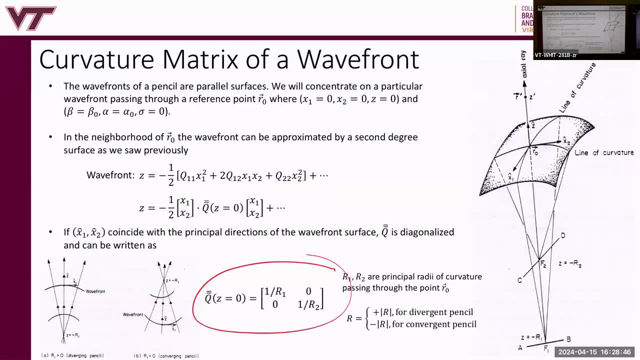 so if that's true, then i can describe this entire surface locally around that point r naught using the q matrix. i guess i wrote it already. it's diagonalized right. so if that's true, then the matrix is diagonal and we have one over r1 and one over r2. r1 and r2 are the principal. 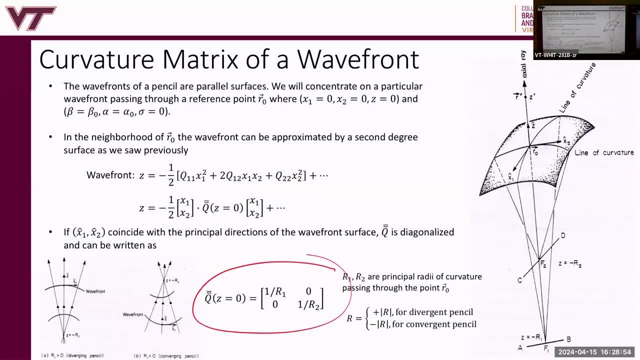 radii of curvature, passing to the point r naught, and in this figure, where are they? so here is a line of curvature along x2. now, it's a principal direction. for example, right in this figure, it is a principal direction. so what is the radius of curvature if i take this curvature? so what i do? 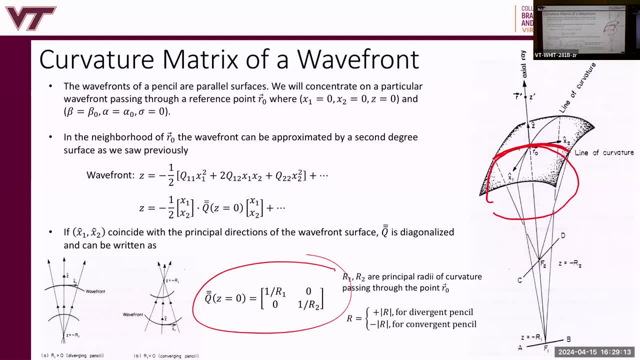 is: i fit a circle, okay, the circle is way bigger than that, all right. but you fit a circle to this line, right, and you find the radius of that and that radius, if you, here's the radius of that circle and that's also a radius of that circle. so this, at z equal to minus r2, for example, is the radius of curvature. 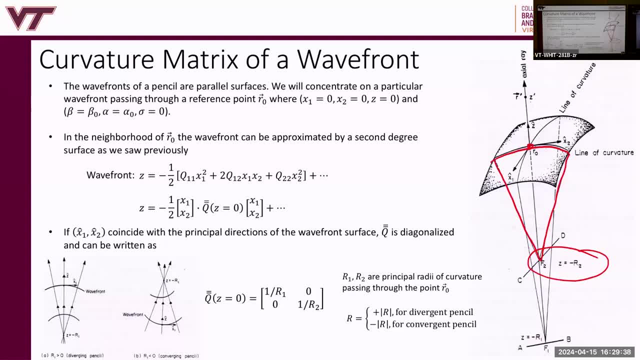 z equal to minus r2, because it's the origin of z. right here's z. that's the radius r2, and then r1, because along the x2, r1 is this line and this one has a different curvature. it focuses over here, at z equal to minus r1. all right, the radii of curvature, one over the curvature. 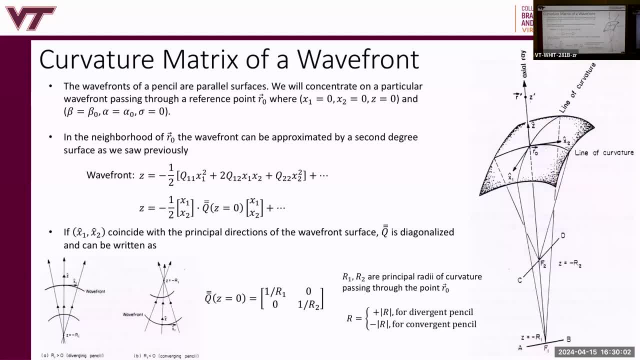 okay, one is the maximum and the other is the minimum. yes, very, very good, yes. so this, this curvature here, the curvature here is either max or min, and this one is the opposite, max or min, and one over those curvatures gives you these radii right. so that is the like: surface approximation, basically like: 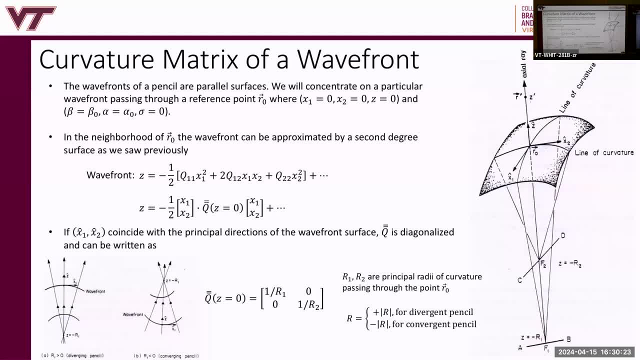 a piece of an ellipsoid. a piece of an ellipsoid. i don't know if this wavefront surface is always ellipsoidal, i wouldn't. i would say no, um, maybe locally. maybe, because it's described by euler's equation, right? so you interpolate from kappa 1 to kappa 2 using cosine squared and sine squared. 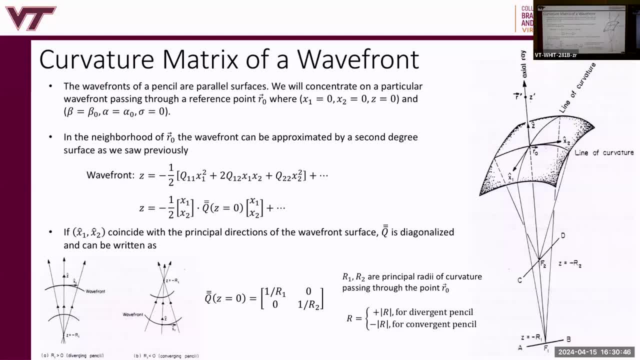 so it definitely has that kind of shape whenever you're in the principal coordinate system. so maybe, yeah, what was that? at least locally? maybe because you approximate the function using a quadratic equation. good point, that's right. we approximate the surface using quadratic form here, keeping only the second order, or second degree or degree, two terms, and therefore probably is ellipsoidal. 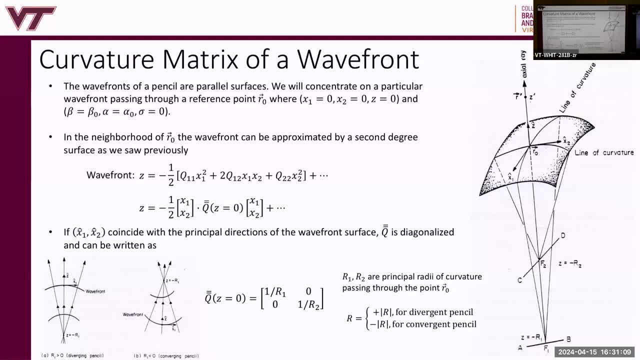 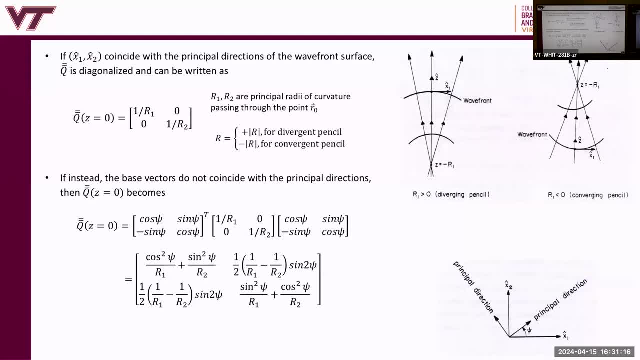 right, great, all right, so, uh. so it looks like i copied this here again. all right, so i copied this here again for principal directions, right? so there's a notation here. r is positive for diverging pencils, so here's a diverging pencil, it's diverging, right. so that means this: r is uh, plus r, so we define as plus r. 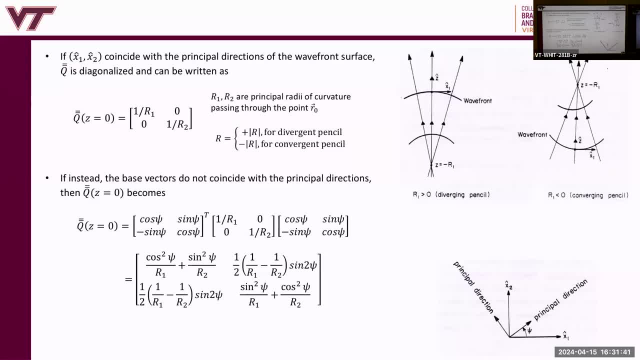 for diverging pencils. that's interesting. okay, it's a positive. oh it's probably because, remember, our normal to this surface always points back toward the source. and then here's our normal here and the curve is diverging. so we know that the normal to the normal section curve. 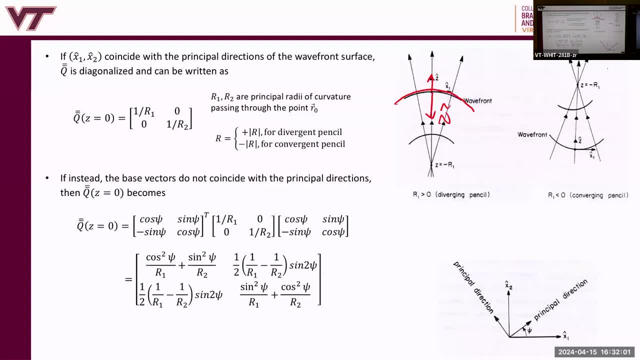 the actual space curve normal is also in this direction, right normal of the curve. so since these two are in the same direction, the dot product give you one, and therefore the curvature of the surface there is positive for diverging, opposite for converging, pencils right. so here we. 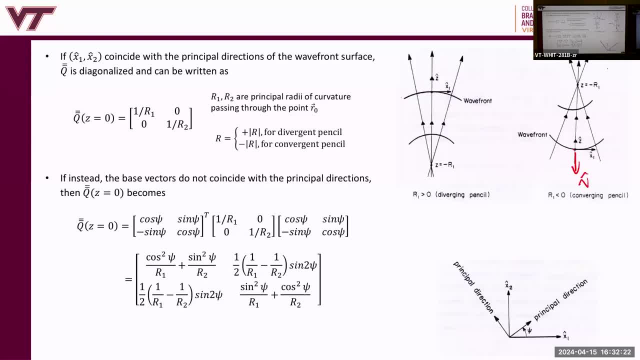 point back toward the source. but the normal, normal to the surface is that way, normal to the curve is that way and you get a minus sign from that because it's converging. yeah, okay. oh, if instead the basis vectors do not coincide with the principal direction, then the curvature matrix at z, equal to zero, can be written by rotating the curvature matrix at 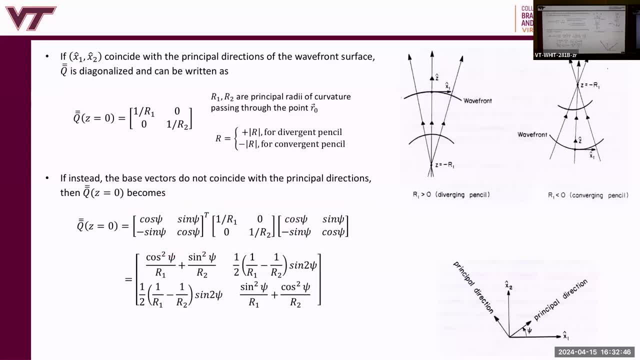 in the principal coordinates, into these new coordinates, right? so psi is the angle. so here's x1, here's x2. the principal directions, let's say, are in this direction, in that direction, right? so if the principal directions are this way, then you have to rotate by angle. psi, your 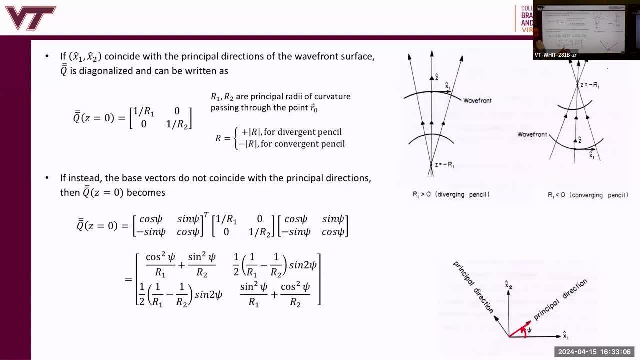 coordinates x1 and x2 coordinate system by angle psi to align it with the principal coordinates. so what you can do is take the curvature matrix in the principal coordinate system and rotate it the opposite direction by angle psi to bring it into the uh x1, x2 coordinate system. and that's what these matrices. 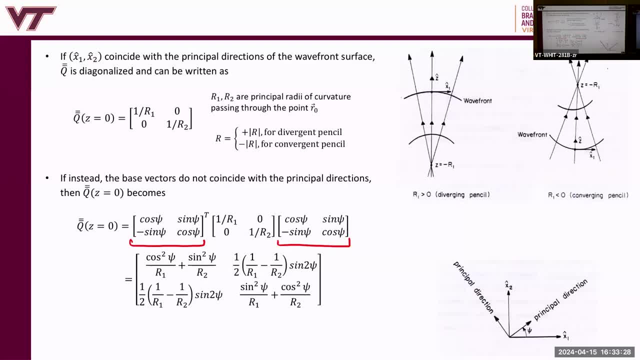 do they just rotate a coordinate system, right? all right, if you multiply all that out, you get this expression. so this works for any coordinate systems, right? good, so all this will become clear. you guys are going to do a homework problem where you your last homework is going to be. i haven't thought exactly what i'm going to make it, but 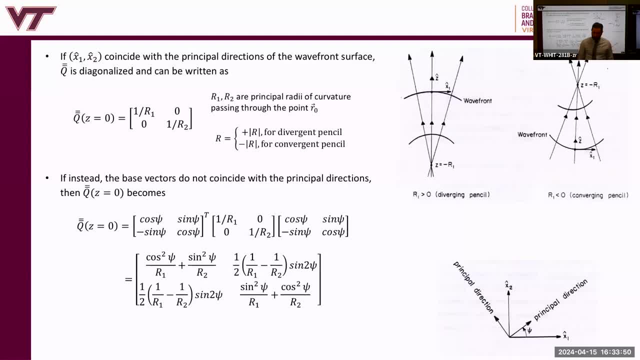 you're going to trace rays and solve, maybe, a hyperbola as a subreflector of a main reflector, dual reflector system, something like that. you're going to trace rays and you're going to reflect them off of surfaces, so you'll get a chance to really, uh, make use of all this. all right. 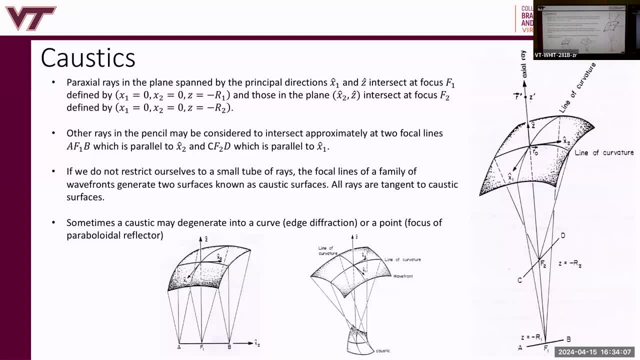 we can talk about caustic now, so all right. so paraxial rays in the plane span by the principal direction x1 and z intersect at focus f1. so okay, here's the axial ray, right? this is the axial ray and goes this way, right? 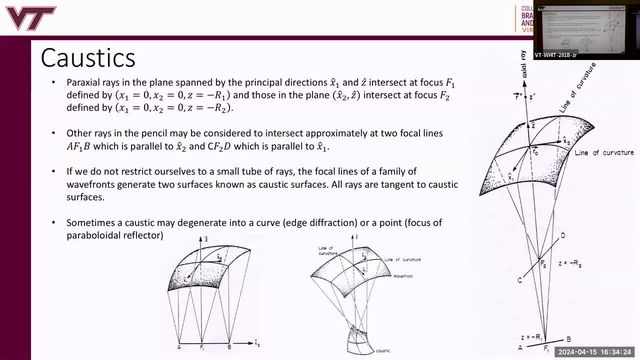 okay, so we have a number of para-axial rays, right? so a para-axial ray might go through the surface like this, right? so this might be a para-axial ray, and that para-axial ray and that para-axial ray. 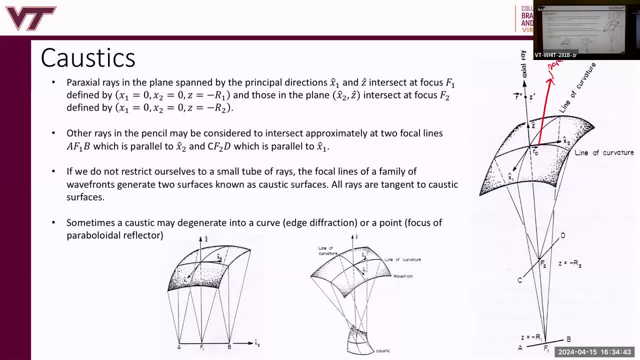 will also have a line of curvature, or radius of curvature rather, but what we find is that the uh focus, or the, you know where the lines of curvature converge, the radius of curvature converges, i guess. so here you can see as, along x2 direction, this line converges to point f2, and so 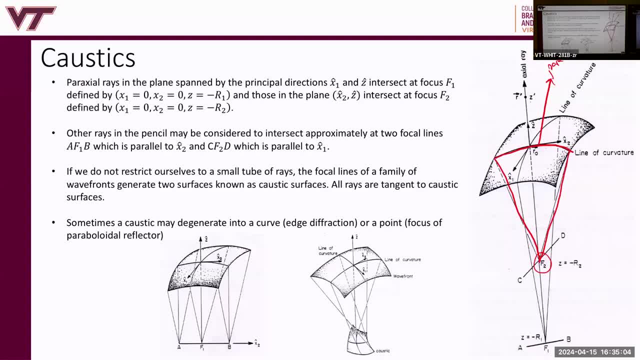 is this one focus right now. a paraxial ray here will converge somewhere over here, like that, and maybe over here like that. right, but all of the paraxial rays in that cut will converge or will, i guess, intersect along the line c to d. all right, so they make. they make a caustic line. 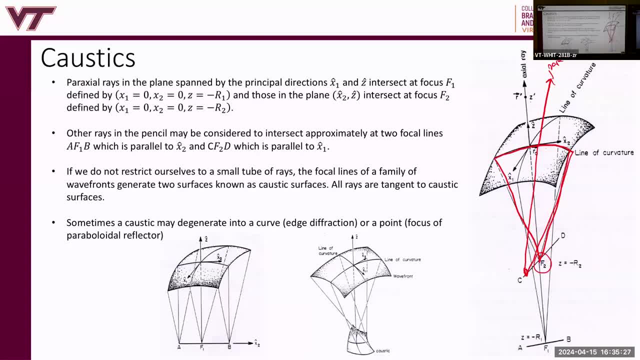 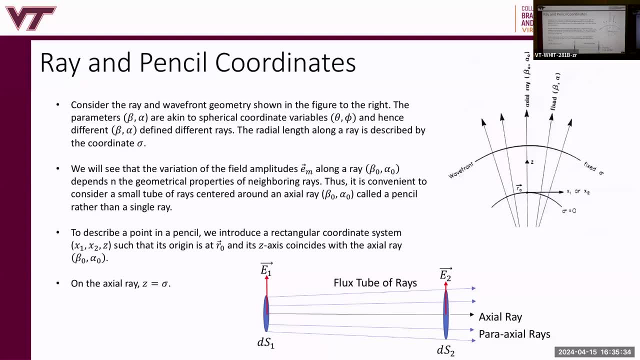 what is the meaning of paraxial? okay, good, so remember. uh, here, if we have an axial ray, we were talking about tracing axial rays when we solve the eichmann equation, but now we said that when we wanted to calculate the amplitude variation or transported amplitudes along the 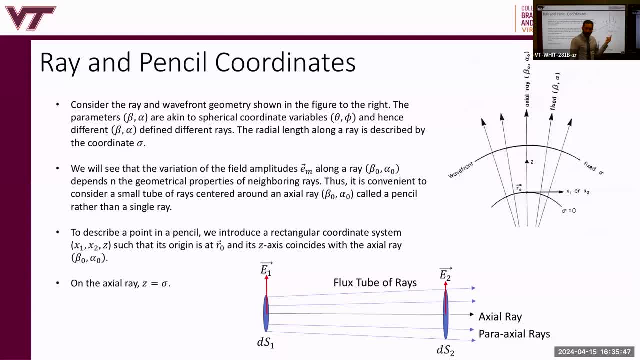 ray, we have to consider neighboring rays as well, and you'll see why we have to do that when we solve the transport equation. but having predicted that, then, instead of considering a single ray now we have to consider a single ray as the axial ray plus the paraxial. 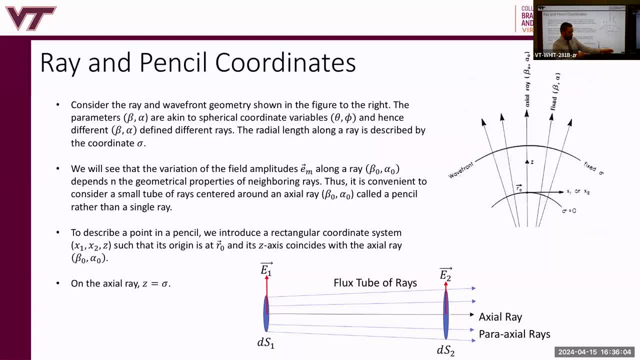 rays, a few rays. so here's my arm. let's say my arm is the axial ray and i have to consider some neighboring rays in a tube all around the axial ray. those are all called paraxial rays. that tube of rays has a cross-section and what we'll find is that the, the amplitude of the electric field. 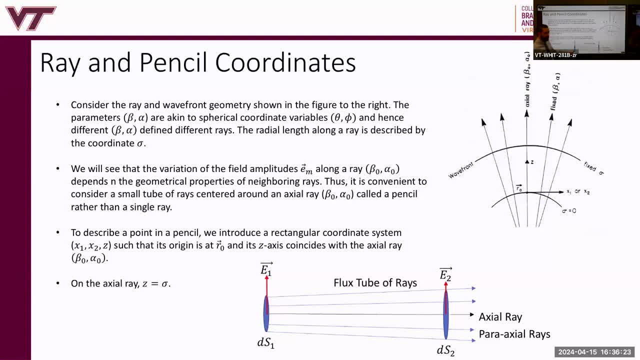 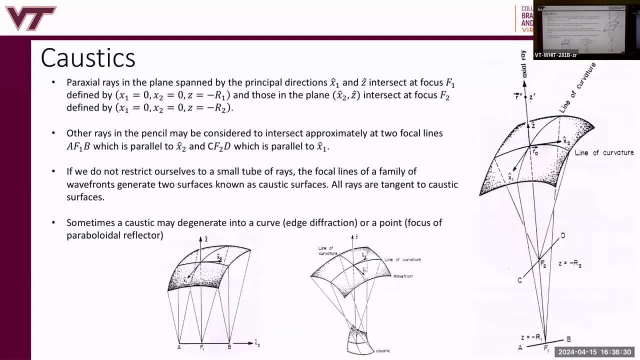 is related to the cross-sectional area of the tube of rays. all right, okay, good, so. so the paraxial rays don't come to the same focus, the same point, right? unless it's like a parabola reflector or something, then then the caustic is a point. 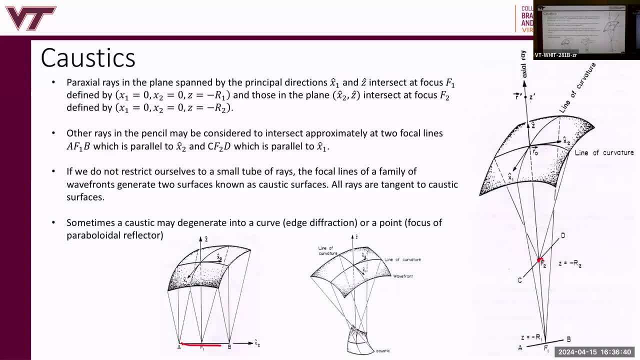 but uh, but rather they make they focus to a line. all right. so here's a surface. look at this surface. here is one line of curvature right through the x1 axis, right like this line of curvature here. it's here, right, that line of curvature. this says: 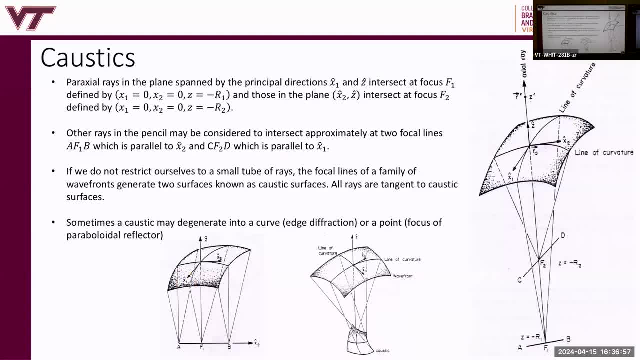 right here says x1. so this line of curvature here, which is aligned with the coordinate system, x2, x1, z, right that one focuses to the point f1, as we noted over here. uh, we're talking about x1 now, so it's this one, f1, all right. however, the next, the paraxial ray, let's say this ray that goes to this: 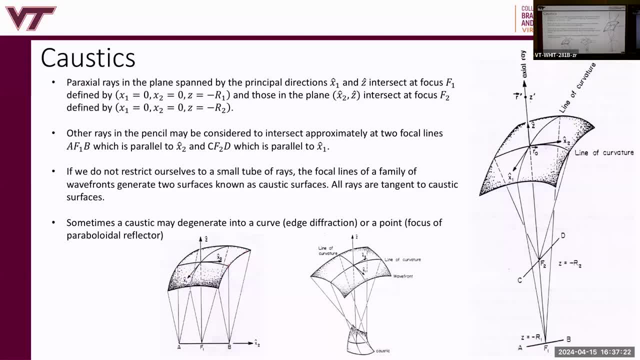 point that paraxial ray. this paraxial ray has this line of curvature in the same direction, parallel to x1, and it focuses over here at a different point along this af1b line. and then this paraxial ray has this line of curvature. 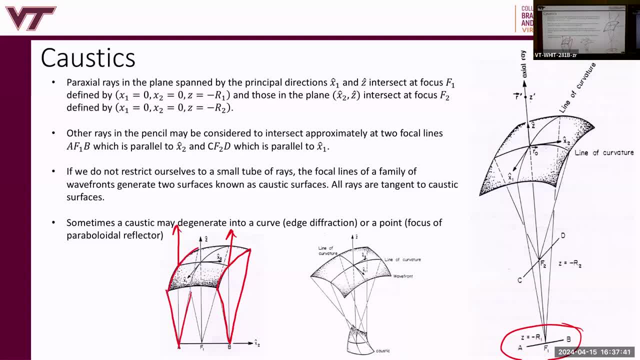 which focuses over here at point a. all right, so the point is the paraxial rays don't all focus to a point. they might focus to a line. if they do, it's called a caustic line, right? so you get a. uh, other rays in the pencil may be considered to intersect approximately at two focal lines. 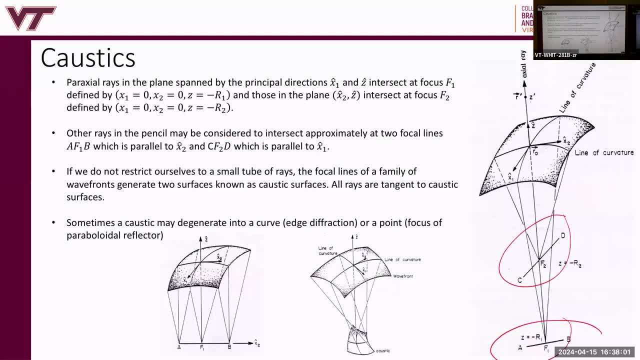 so you get these two lines all right, and that in that case they are called caustic lines, all right. okay, if we don't restrict ourselves to a small tube of rays, the focal lines of a family of wavefronts, so a bunch of different wave fronts now, uh, generate two surfaces known as caustic surfaces. 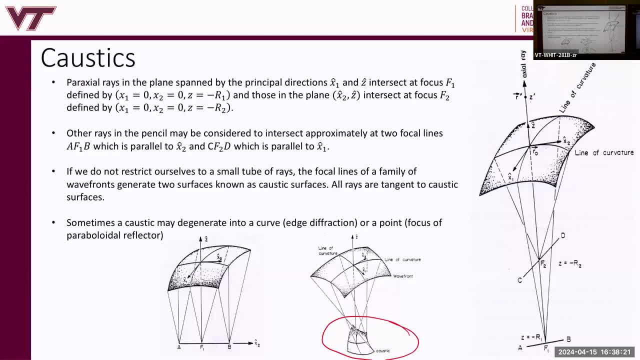 so you could get a whole surface if we, you know, think about more than just these parallel lines here. but we start considering, you know, more of these- and neighboring wave fronts, right parallel wave fronts. they might all intersect at a caustic surface. all rays are always tangent to caustic. 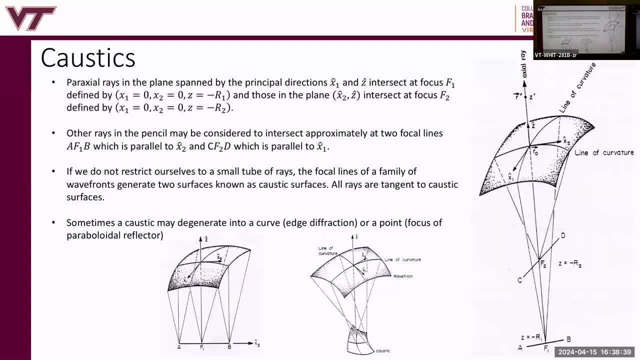 surfaces. that's how you define these caustics, all right, all right. so sometimes a caustic may degenerate into a curve, in the case of edge diffraction, or a point like the focus of a parabola paraboloidal reflector. yeah, all right, don't worry about caustics for now. 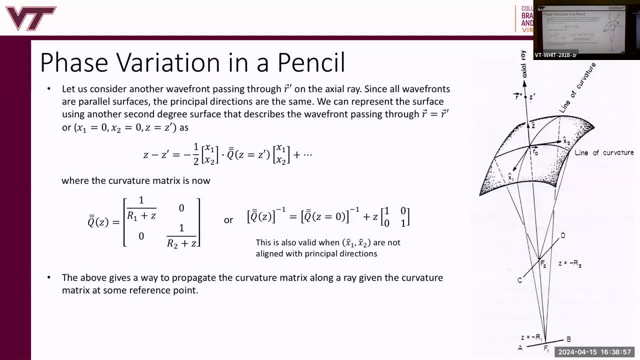 all right. so let's let's see how we can calculate the phase variation of pencil. we figured out how to calculate the phase variation along an axial ray right. all we had to do there was multiply k by the optical path length that we calculated from point r naught to r. right now, that's for. 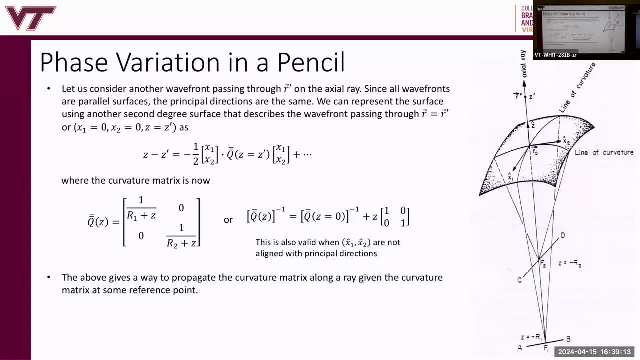 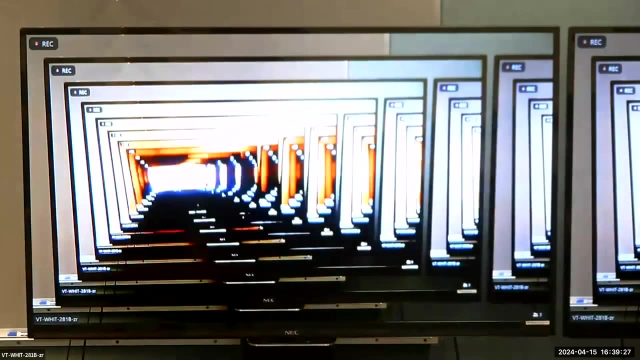 the axial ray only. how can we also measure the phase variation in the pencil, which is the axial ray plus the pair axial rays? so let us consider another wavefront passing through our oh no, no, through r naught or r prime, rather so through r prime on the axial ray. all right, there's another. 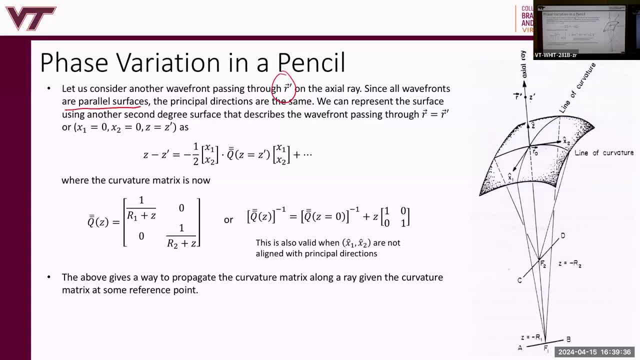 surface. now, since all wavefronts are parallel surfaces, the principal directions are the same. all right, so we're in the principal directions for this particular wavefront. we're considering another wavefront here. that's at point, you know. uh, this point here would be maybe a 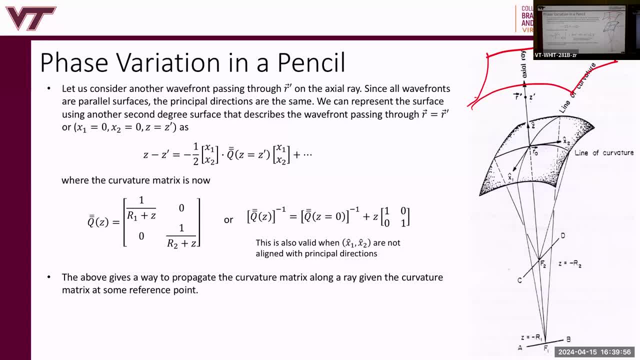 should probably draw it here right. uh, here this point. here is r prime. the principal directions here: in the same direction as the previous wavefront, because the wave fronts are parallel surfaces. all right, we can represent this surface using another second degree surface that describes the wavefront passing through r equal to r prime, or x 1 is still 0, x 2 is 0. 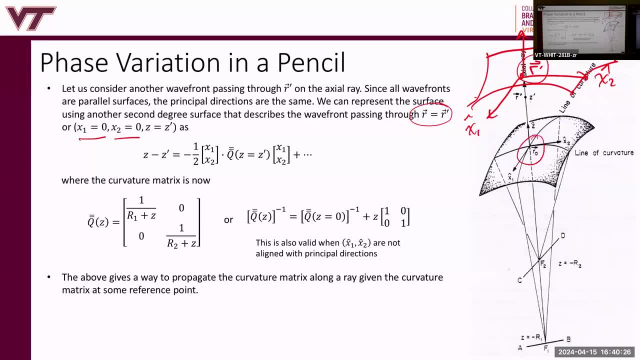 so r prime here and r naught in this coordinate system. here the x 1 x 2, z has r prime is related to r naught, as x 1 equal to 0, x 2 equal to 0 and z equal to z prime right. 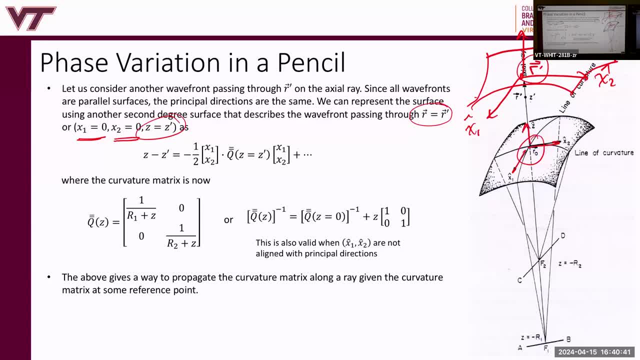 yeah, okay, so we know how to propagate a curvature matrix. right, we've done that. the curvature matrix that you propagate here is q at point z. so here is q at point z equal to zero. this would be: q at z equals to zero. we want to propagate it up to this wavefront here. 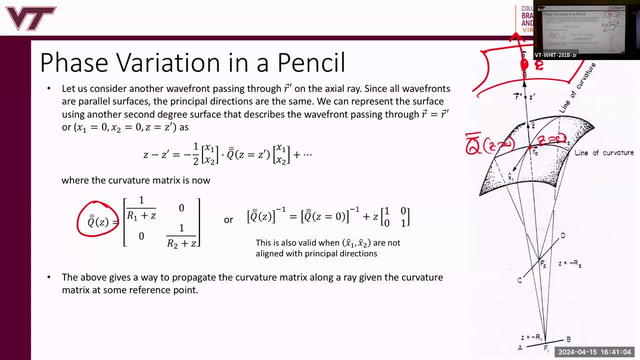 at r as z. so okay, uh gosh, at uh, z equals to z prime. so q at z equals to z prime for this surface. about this point: here: uh can be calculated in terms of the curvature matrix on the original surface. how do we do that? first, we expand this surface up here, so there's a this: 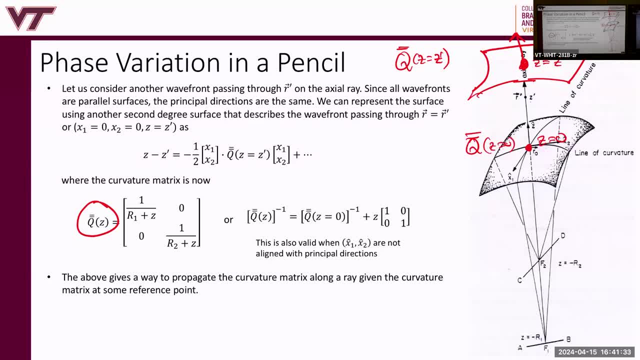 wave front, here the, the uh. the wave front at z equal to z prime is expanded like this: z minus z prime is equal to minus one half. you know the second order approximation for service, except now we're using the q matrix. it's equal to z prime, right, and we have to do all of. 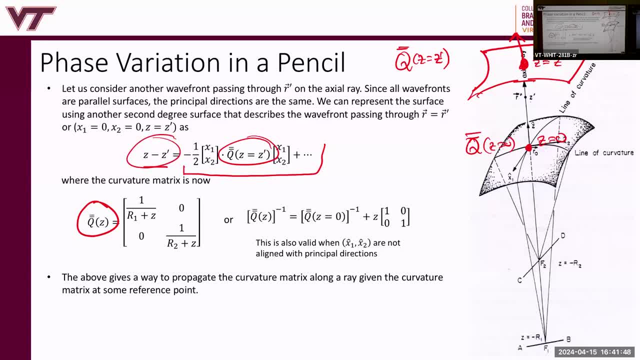 that at z minus z, prime has to be the new origin. all right, to propagate a q matrix to a point z, if we're in the principal coordinate system, all we have to do is add the new radii of curvature. so think about it like this: here's the wave front at z equals to or z equals to z prime. 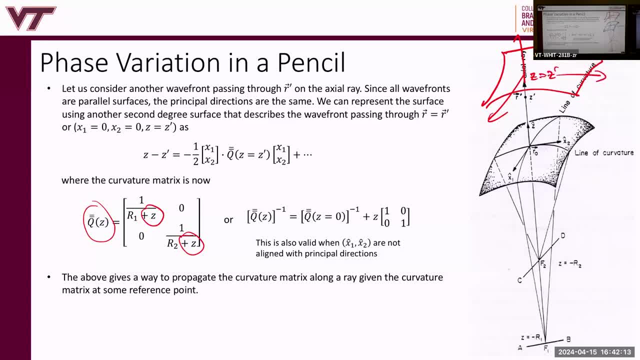 this has the same principal directions. right, the radius of curvature is going to be the new radius of curvature. the radius of curvature is going to be the new radius of curvature, to be larger because it's an expanding wavefront, for example. right so, but the curvatures are the 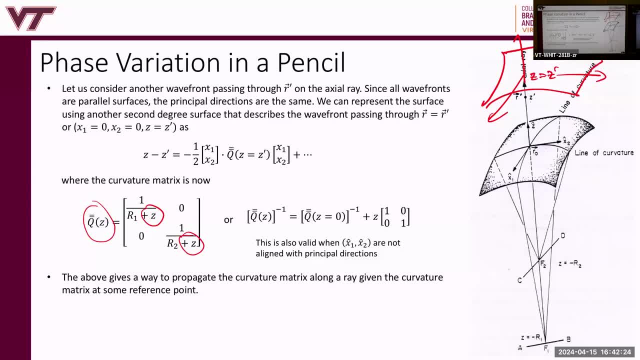 same. no, the curvature is not the same. the directions, the principal directions, are the same. so here we're going to get a line of curvature like that and it's going to focus to the same point, and here we're going to get another line of curvature and it's going way down here, right. 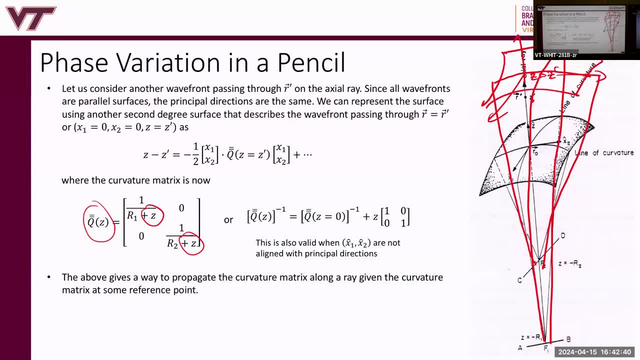 it's expanding from the same point to the same origin, basically. so we just have to add this distance, z, to the radii. okay, z prime is infinitely, infinitely close to z, or not? or z prime is what now is infinitely very close to z, or not? uh, it doesn't have to be not infinitesimal, right? yeah? 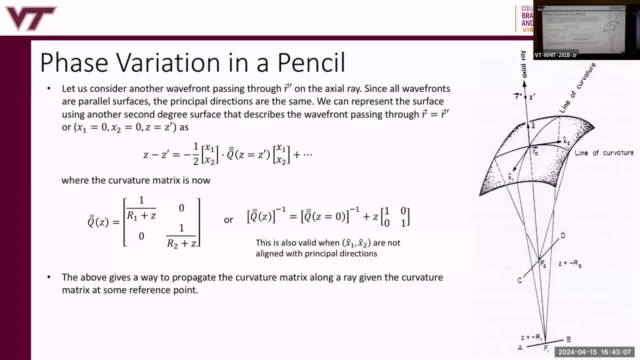 okay, so we can also write this in terms of. we can write q of z in terms of q at z, naught by saying that since, remember, q itself has curvatures, so the inverse of q, if it's a diagonal matrix, has radii of curvatures, because to invert a diagonal matrix you just invert all the entries. 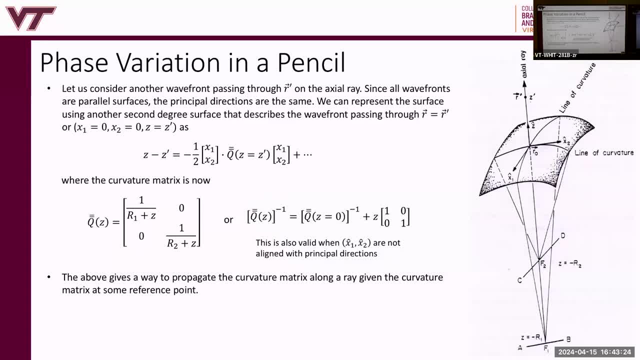 the diagonal entries of that matrix. all right, so we can say q, that's equal to zero, inverse, plus z as a diagonal matrix. same thing as this, and this comes from geometry, right. so the above gives a way to propagate the curvature matrix along array. given the curvature matrix at 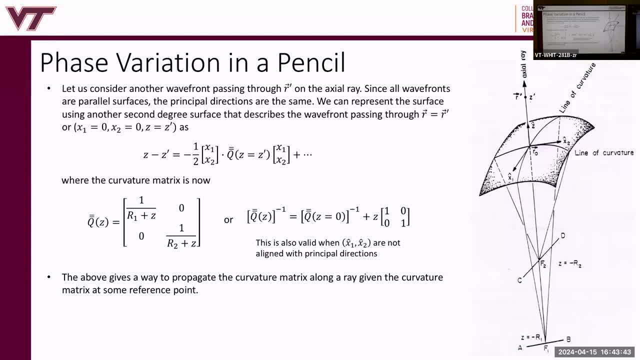 some reference point, very important for tracing rays. all right, i'm gonna do that a lot. you're going to start with a fee, but that Hubadываем just made that. i'm just saying this because- and we should also pinky some it to to shape the curve it. we can have some picked out, we can do some fine processing, we can. 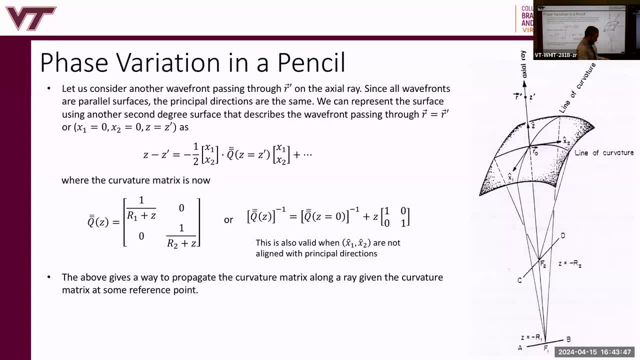 going to start with a feed or a known source And you're going to start with, maybe, a spherical phase front, So you know what the radial curvature are at some point along the ray, And then you'll want to find some other point where you have a surface that you're going to intersect. 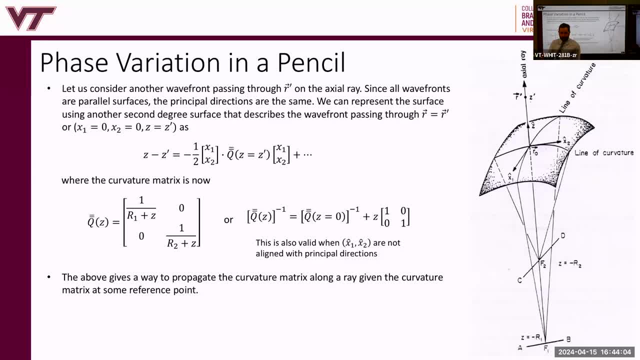 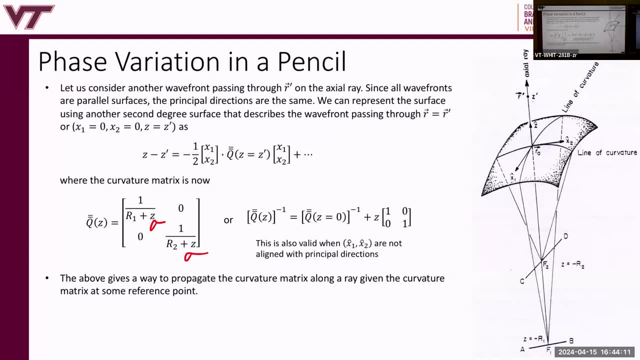 So you just add the axial distance, So this z is the axial distance. So remember, OK, so sigma is probably better. I think we do that on the next slide. Sigma is probably better, But we're talking about axial ray here. 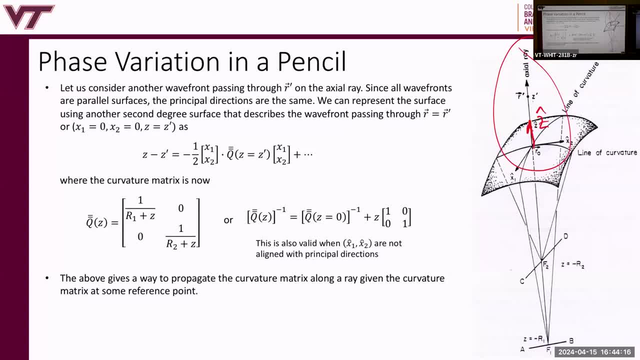 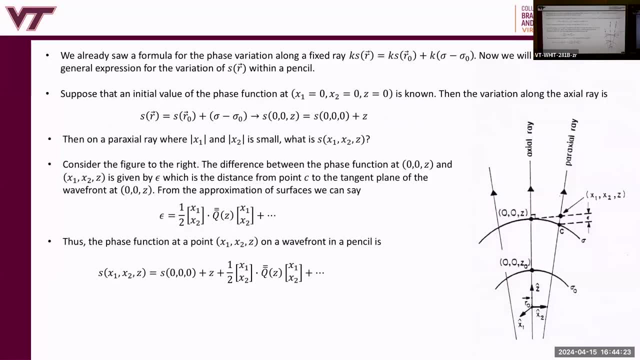 And the axial ray is aligned with the z-axis here, right, So we can say z, but it's probably better to say sigma, All right, so OK, so we already saw what are we trying to do. We're trying to calculate the phase. 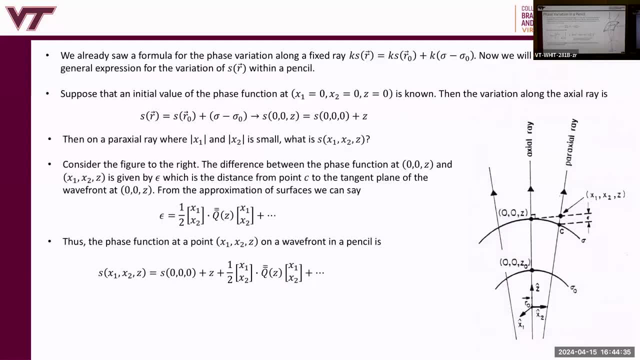 at neighboring points of the axial ray within the pencil. So we already saw a formula for the phase variation along a fixed ray, which is we derived this right? We derived this By integrating the arc length along a ray and using the Eichmann equation and solving the Eichmann 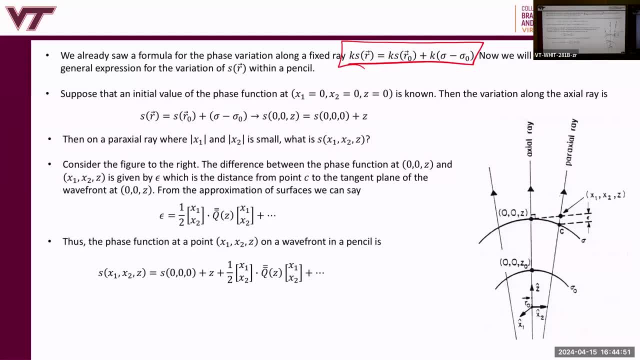 equation which showed the rays are straight And we found that the phase at r relative to r0 is given simply by the phase at r0 plus the optical path length multiplied by k, which gives you the phase along the ray from point r0 to r right. 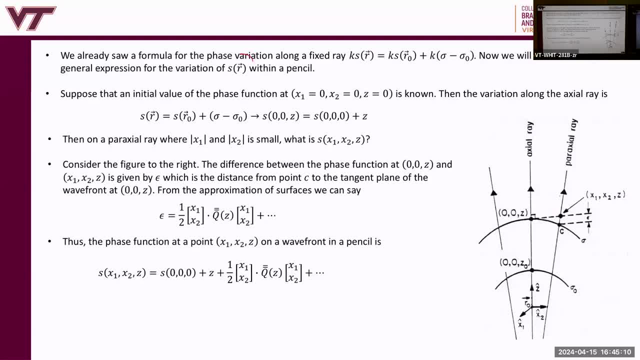 OK, now we will drive a more general expression for the variation of s within a pencil. So suppose that at an initial value of the phase function at the origin, x1 equal to 0, x2 equal to 0,, 0 equal to 0 is known. all right. 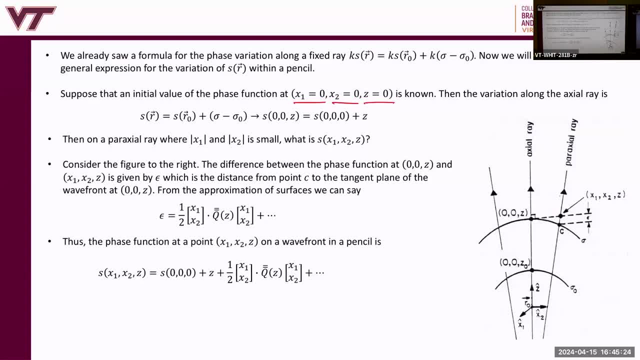 The phase function is s here. OK, then the variation along the axial ray is this: Does this make sense? We're talking about axial rays, So we already saw this formula for a ray, And if we're going to call that ray an axial ray, 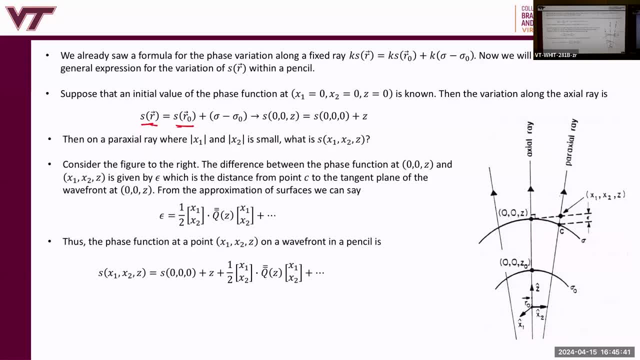 then s is equal to s at r0.. s at r is equal to s at r0.. Plus sigma, minus sigma 0 for a ray right. And in our coordinate system here, in our pencil coordinate system here, we have x1,, x2, and z. 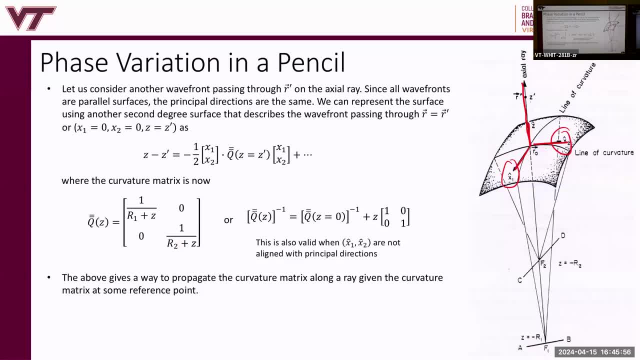 We're talking about the axial ray, Then x1 is equal to 0,. x2 is equal to 0, right, So we can say that that is s at 0, 0, z, x1, x2, z. 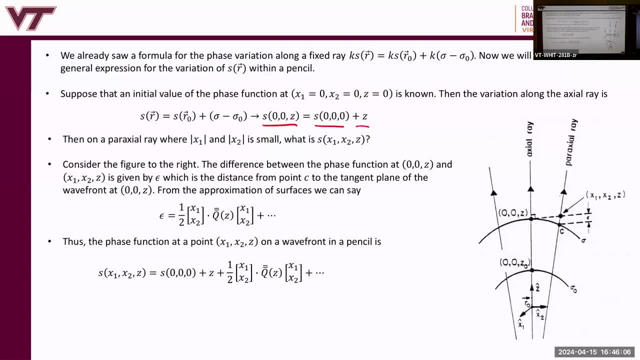 So 0, 0, z is equal to s at 0, 0, 0 plus z. yeah, All right, good, So now consider the figure to the right here. So this figure, This figure, The difference between the phase function at this point: 0, 0, z. 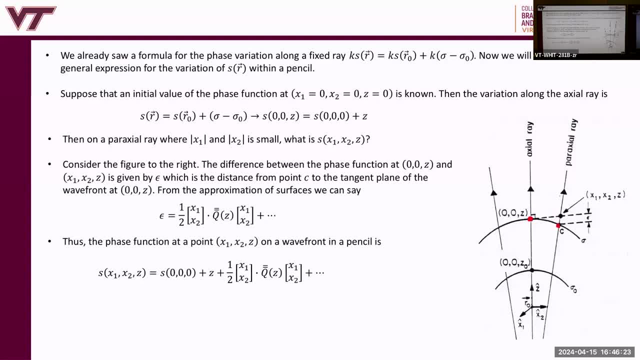 and some neighboring paraxial ray is where the sigma intersect. at the point c is this value epsilon? So because we've moved in the tangent plane to this point, we've moved in the tangent plane to this point, which is x1,, x2, and same z right. 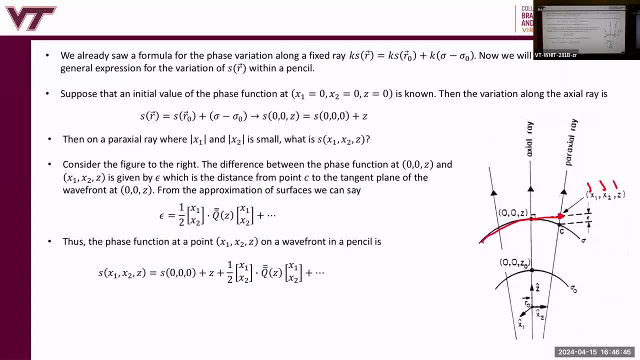 Because we moved to that point. the surface has moved, The wavefront has moved away And the wavefront tells us the phase right, The length from one along the ray, rather right. So the difference between this point in the tangent plane, 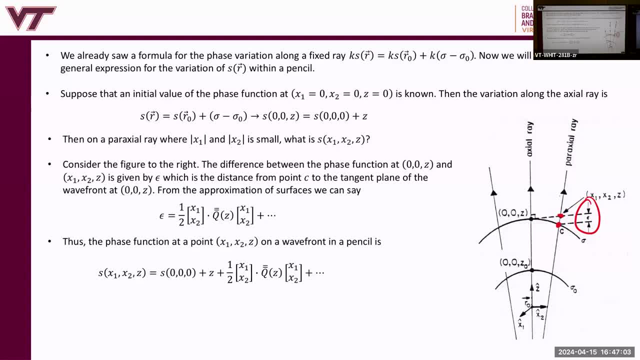 and the actual surface we call sigma. What is that? That's nothing but the height of a function that we measure from respect to the tangent plane coordinates. So we can just expand that in terms of a second degree approximation, right? So So we say: epsilon here is nothing but our second degree. 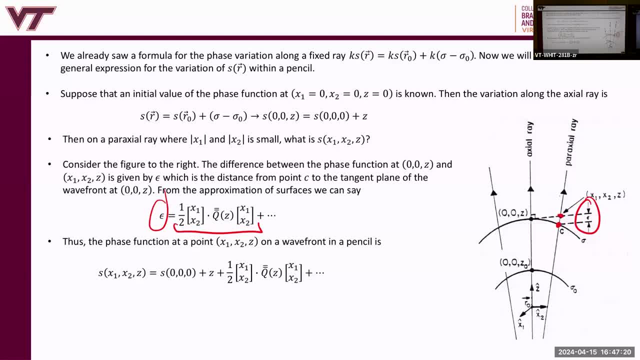 approximation right: q at z. Very good, So now we can use the same concept, The phase function, at s equal to x1,, x2, and z, rather than at s equal to 0, 0, z is s at 0, 0, 0 plus the z. 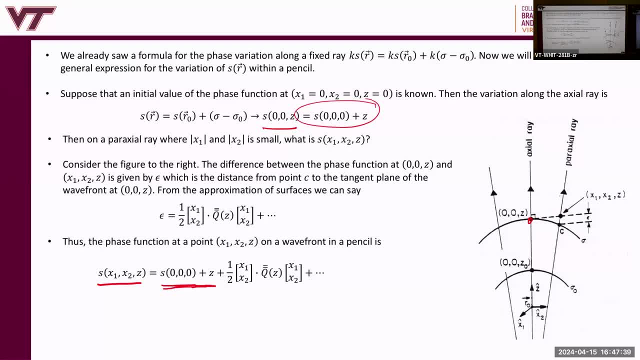 right. This brings you to the axial ray at this point here. And if the wavefront were planar, then that would be the phase everywhere. And all x1, x2 coordinates, x1, x2 coordinates at sigma equal or z equal to 0, z equal to z. rather right. 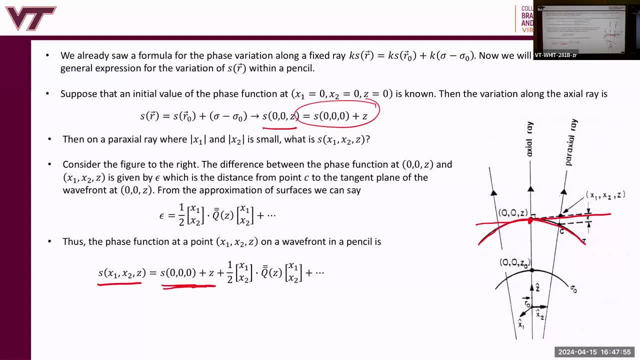 But because this is not a planar wavefront, there is a small phase deviation because of this point c not being in the tangent plane, right, It's epsilon, So we have to add that phase. So what happens when x1, x2 equals to 0?? 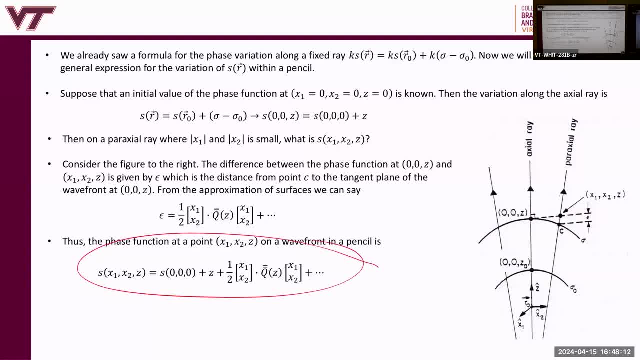 0. 0. 0. 0. This function right here. If x1 and x2 are equal to 0 in this function, what happens? What? Where On the No, So x1, x2 equal to 0 puts you here's. 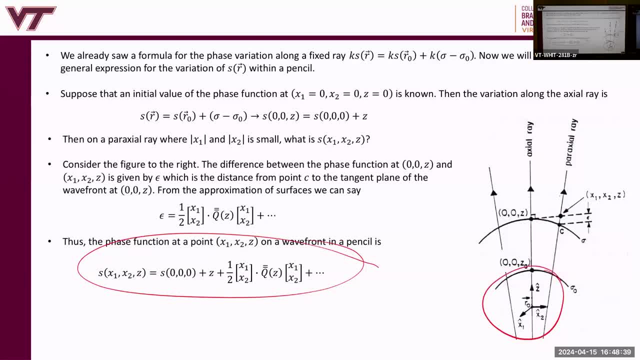 the x1, x2 coordinate system. right here, This is the coordinate system: x1, x2, right, Right. So X1 equal to zero, X2 equal to zero. put you on what ray? Axial ray. So if I plug in X1 and X2 equal to zero and zero here, this whole term goes to zero, Right? 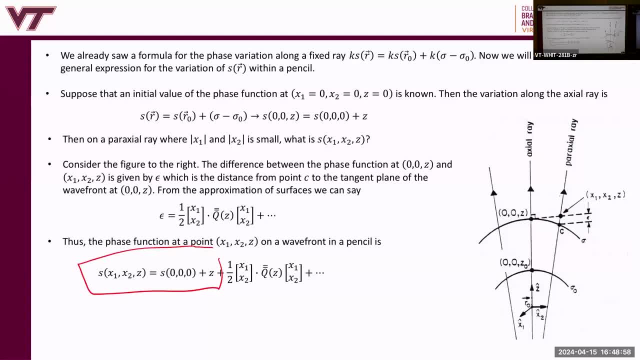 So that means I get the phase of the axial ray only if this were zero and this were zero, which makes sense, Right? So this other second degree approximation is a correction for the shape of the wavefront to different X1 and X2 in the tangent planes for the phase of the wavefront in those points, Right? 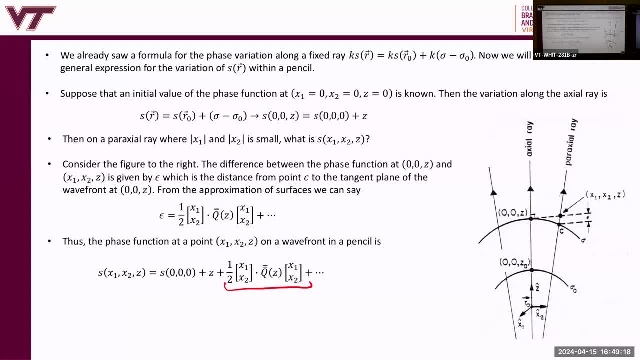 I think in this case it should be minus, right. Minus one over two, Yeah, I would agree. Why do we have it as positive? I agree with you. This should probably be minus. here I'll look back, But I think that should be minus. It makes sense. 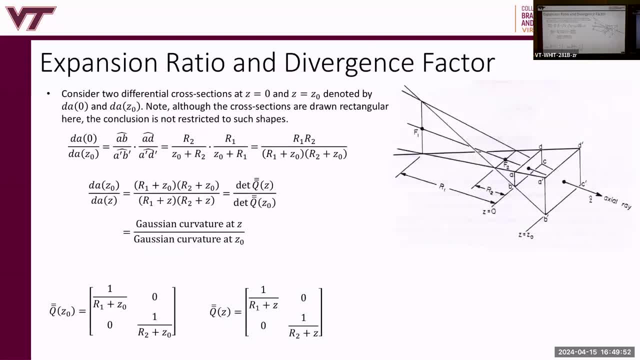 All right, Good, So let's start talking about amplitudes, Right? So once we get to the derivations of these, how to propagate or how to calculate the phase along the ray and how to calculate the amplitude electric field along the ray? 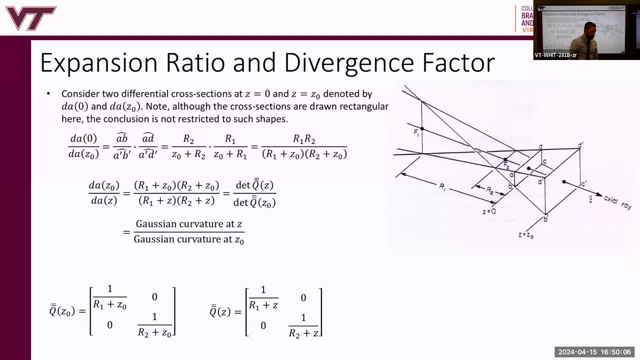 Then we're done, We just have to trace things. We then have to learn how to calculate reflected Q matrices. But after that we're done, All right, And then we get into diffraction from edges. OK, so consider two differential cross sections at Z equal to zero. So here's: Z equal to zero and Z equal to Z naught. 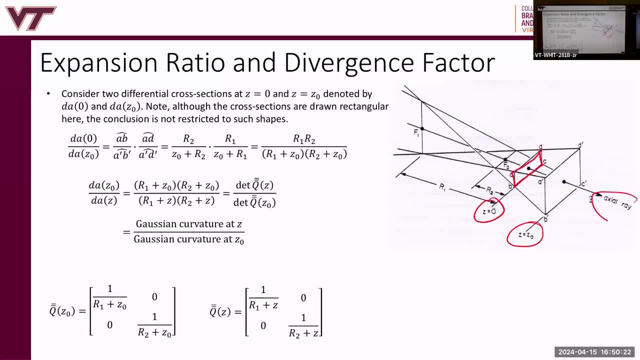 Here is a differential cross section of the axial ray and the surface carried by it. In this figure these cross sections are square or rectangular rather, but normally they're not. But the argument is not this argument. It works for any shape surface, All right. 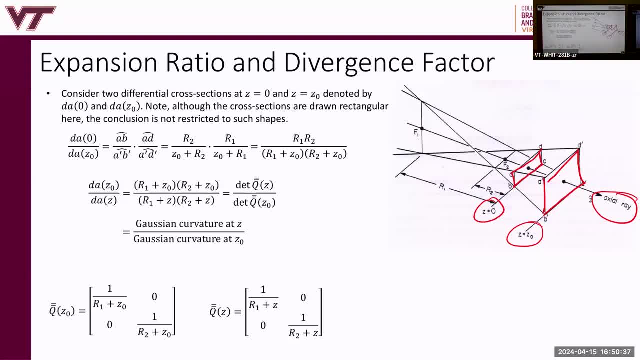 The result is general. So What is the ratio of this cross sectional area to this one? That's what we're trying to calculate, All right, So DA, which is the change or the differential cross section of area at Z equal to zero and Z equal to Z. 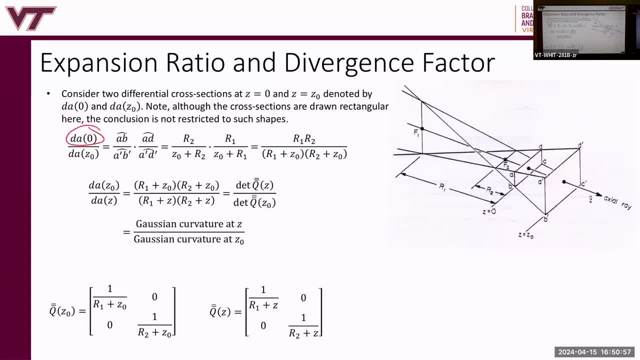 We can calculate that Well. DA at Z equals to zero, is nothing but A times D multiplied by A times B. Right, That's this. And then the other one is A prime times D prime divided by A prime B prime. 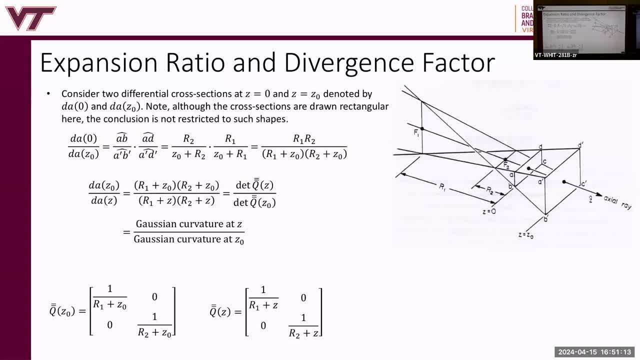 Or multiplied by A prime, B prime. OK, All right, So Let's see. Then we say that this is R2 over Z naught plus R2.. OK, let me see here R2.. R2 is there, So R2.. 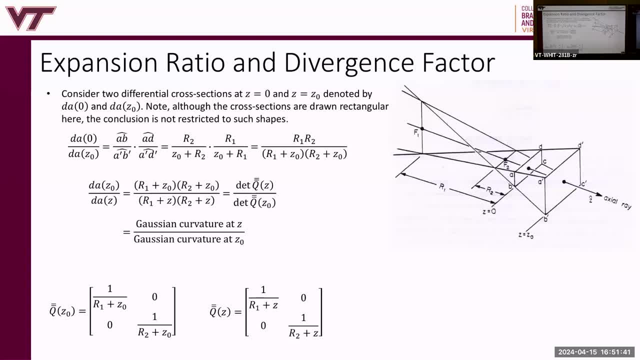 Multiplied by R1.. OK, In this sense, R2 and R1 are still radii, Right? So this radii describe the. if you multiply the two radii, it describes. So, OK, A B divided by A prime, B prime. What is that? 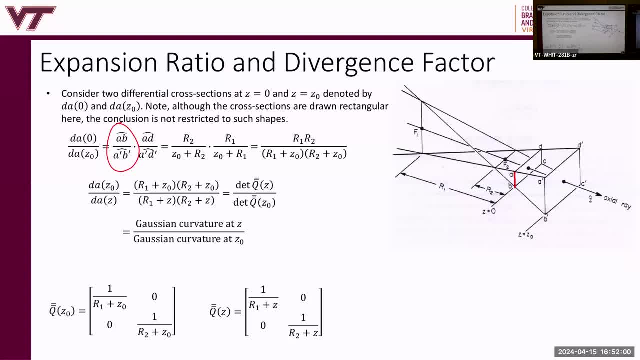 So A B is here, A B is here, And A prime B prime is here. Right, The difference between these two is equal to R2 divided by Z naught plus R2.. So here's R2.. Those, those are the same. 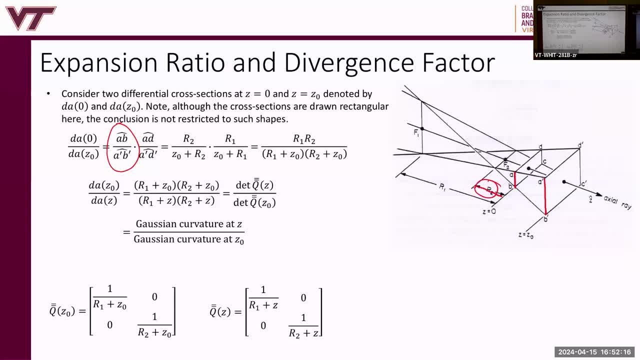 This would be due to the geometry. All right, So R2.. R2 is this distance, And if you add Z naught to R2, that gives you it's similar triangles, Right? So here you have these two triangles And here, Right? 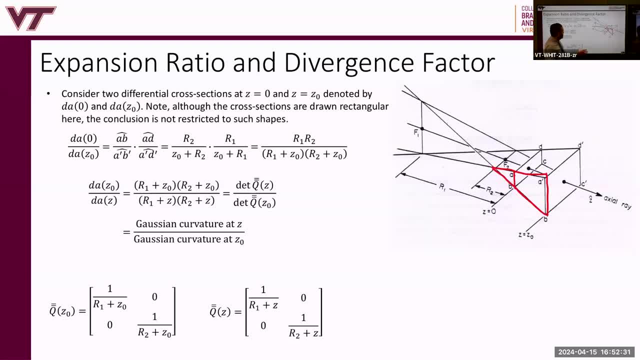 So it's similar triangles. If you ratio the ratio of, Let's see the ratio of A, B to A, prime, B, prime. So A, B this side to this side, the ratio of these two sides is the same as the ratio of this side to this whole side here. 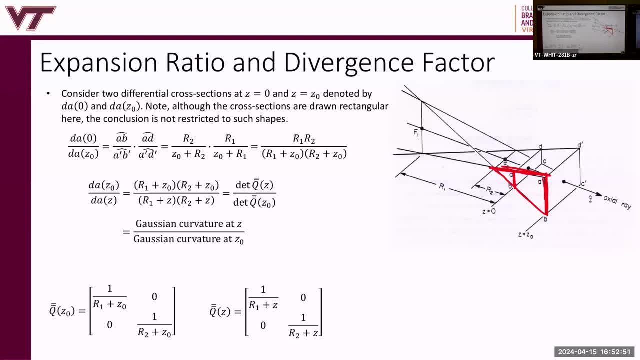 Right, So you can express that in terms of the radii of curvature, And you can do that for both. You get this expression here, And what we notice here is that if we do the same thing For- Yeah, this is correct, So we do the same thing now. 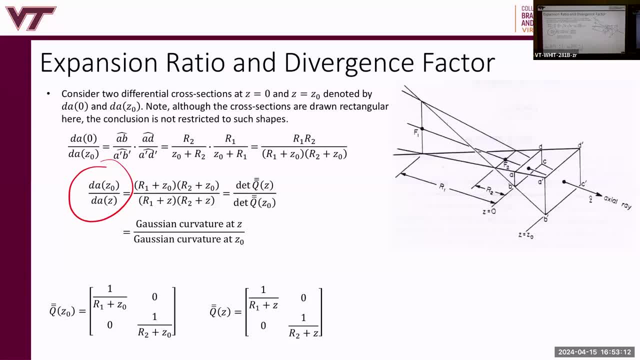 So, Oh, we invert it, All right. So invert the whole thing, You get this expression Right. And now we're going to say from a general Z naught to Z instead of zero to Z, instead of zero to Z naught. 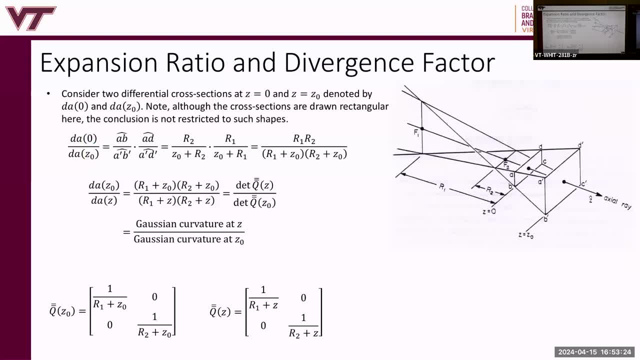 All right, Now what we notice, this, the numerator we notice, is the determinant of the Q matrix at Z Right. Let's go back. Oh, here, The Q matrix at Z naught. This is the Q matrix at Z naught. 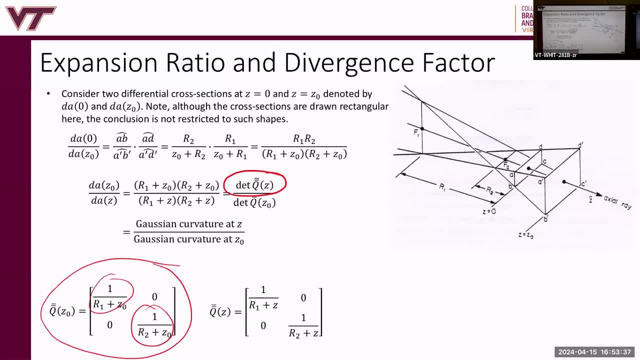 If you take the determinant of this, how do you calculate it? This times that minus zero, Right? So this is the determinant of Q at Z, And this one is the determinant that Q at some some point Z Z. Why is that? Oh, because, All right. 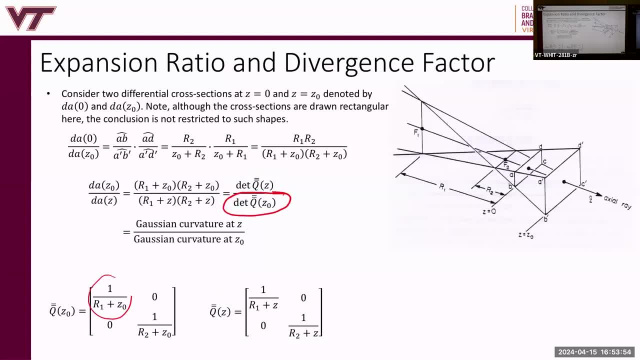 The determinant of Q at Z naught is one over R1 plus Z naught times one over R2 plus Z naught, And if you invert that, then you get this as the numerator. All right, OK. so what does that say? 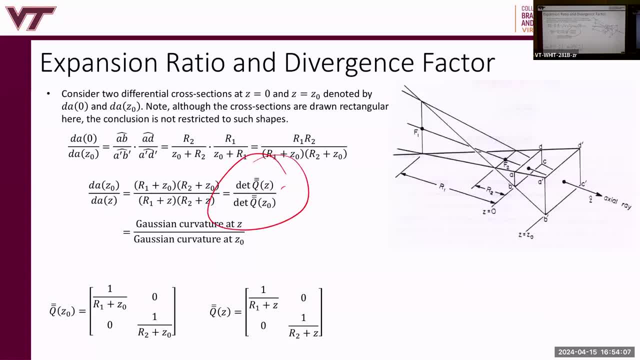 That says that the determinant to the Q matrices- if you ratio the determinant to Q matrices are two different points along a ray in a pencil, then that you can calculate the difference, the ratio of the cross-sectional area of the flux tubes. All right. 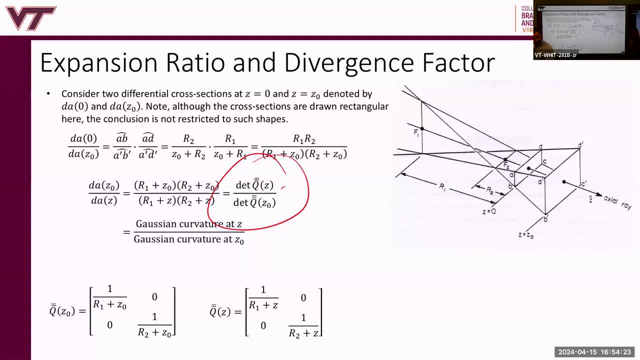 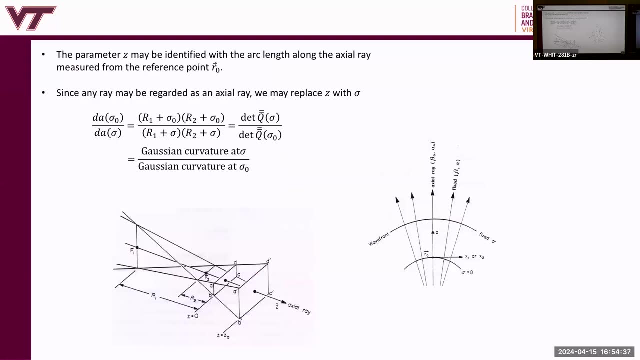 Based on geometrical principles. that's going to be related to the amplitude of the ray, Amplitude of the electric field carried by the ray. Sorry, Yeah, OK. So we can also do this as a function of sigma, right? So instead of saying Z and Z, naught, we can say sigma, because the parameter Z may be identified with the arc length along the ray. 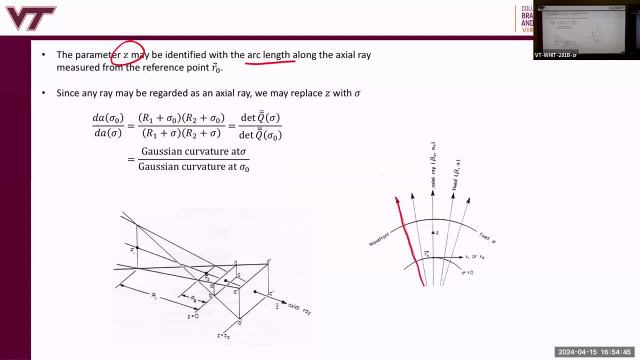 And any ray you can consider as an axial ray. I can say: this is the new axial ray and the tube of rays, the pair of axial rays would be around it. So we can say: and sigma is always the arc length parameter along an axial ray. 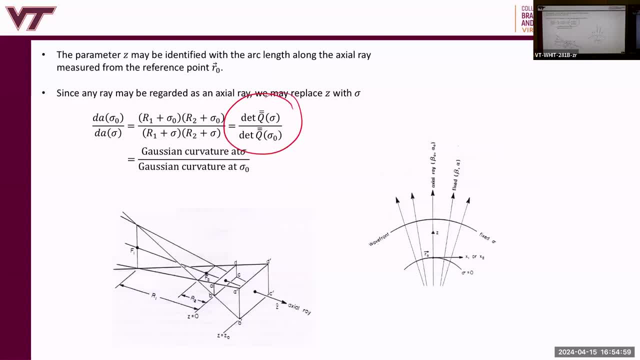 All right, Good. So this is our formula, which is the: what is the determinant of Q at sigma? This is the Gaussian curvature at sigma, The determinants related to the Gaussian curvature, Remember, It's the eigenvalues. So now we have, OK, so the Gaussian curvature at sigma and the Gaussian curvature at sigma naught. 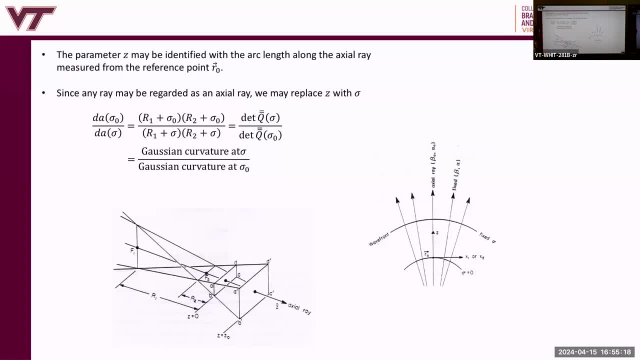 if you ratio those two, which you can calculate by calculating the determinants of the Q matrices, then this quantity will be related to the change in amplitude of the electric field carried by the ray. We call that the divergence factor. All right, So along a given ray, 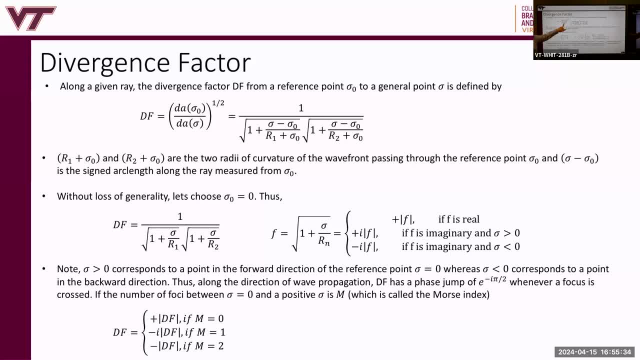 the divergence factor df from reference point sigma naught to a general point. sigma is defined as the square root And you'll see this why. Why is it the square root And how is this related to the amplitude? We'll get to that. 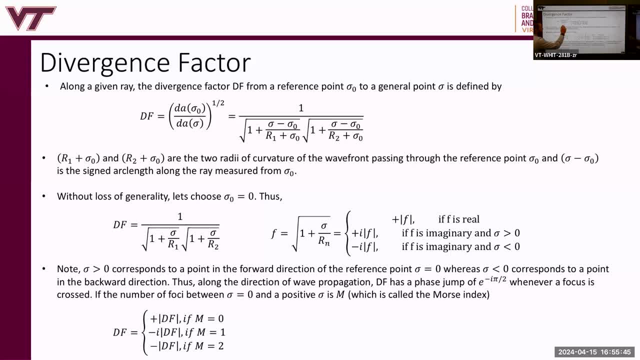 We're going to solve the transport equation. But dA at sigma, naught, divided by dA at sigma, square root of all of that, gives us the divergence factor. What we're going to find is the electric field. E at point sigma is equal to the divergence factor multiplied by. 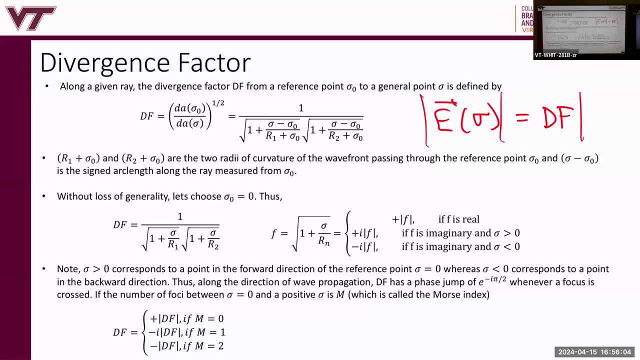 Oh, so the amplitude, sorry, By the E at sigma naught. So now we can trace rays, We know the shape of the rays, We know how to calculate the wavefront curvature, propagate the curvature matrix along a ray, And now we can calculate the divergence factor at different points along that ray by calculating the Gaussian curvature. 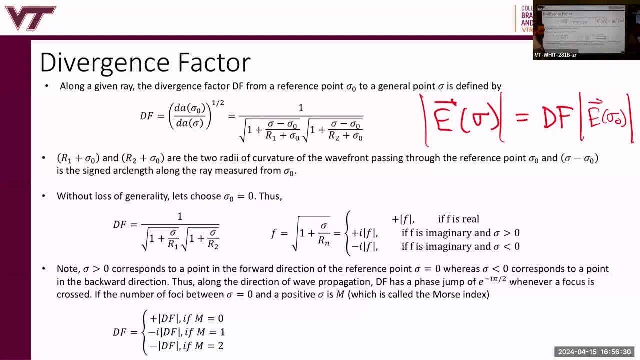 the determinants of the Q matrices at those two points. Right, So we can now calculate the phase and amplitude of the electric field carried by rays. Right, All right, Great. So let's say sigma naught is equal to zero, And what we'll find is the divergence factor looks like this: 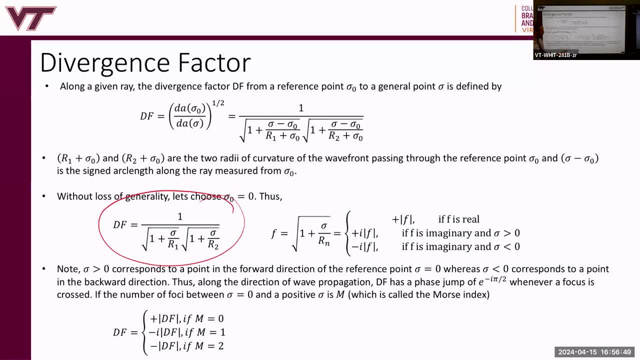 All right. So there's something interesting about these square roots, though, Right? So, depending on where sigma, sigma is measured, positive in the direction of wave propagation, Right? So Let's see So Okay, So All right. 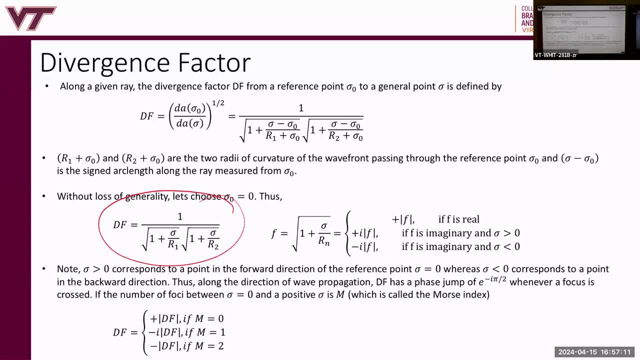 So All right, Okay, Without loss of generality. This function F can either be positive, imaginary minus imaginary or real. Right Depends on whether sigma is greater or less than zero, And And if F is, F becomes real valued. So there's a sign convention here. 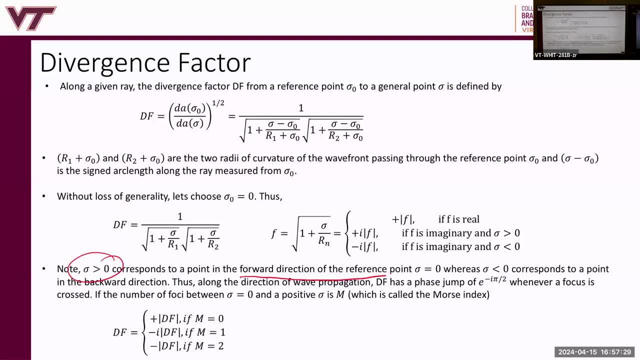 So remember, Sigma equal to zero corresponds to a point in the forward direction of the reference point. sigma equal to zero, Whereas sigma less than zero corresponds to a point in the backward direction. So positive sigma is in the direction of propagation. Thus, along the direction of wave propagation divergence factor has a jump of e to the minus. i pi over two whenever a focus is crossed. 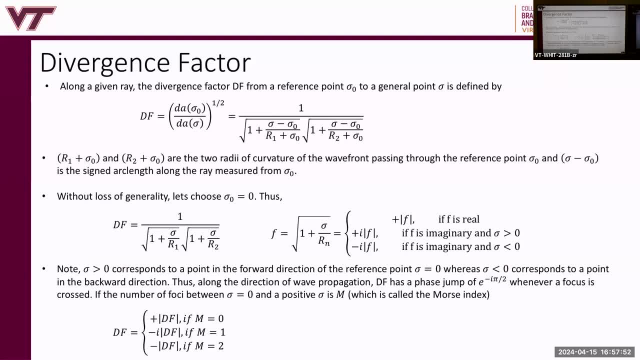 Let me see if I have a figure for that. Yeah, we'll do an example, All right, Okay, So. So let's say that Sigma is my variable right, And let's say I have a way front And I start to trace backward. 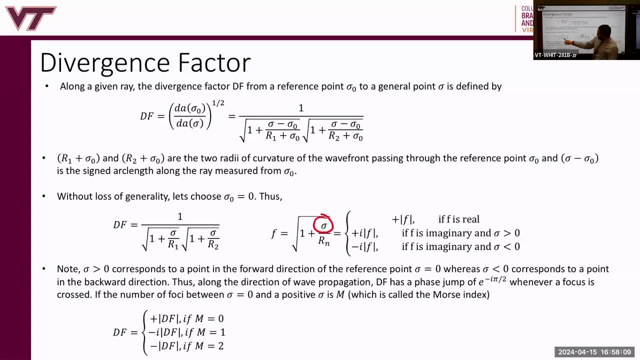 Until I get to signal equal to R one Right Or negative R one. even When Sigma is equal to minus R one, Then this thing becomes a square root of zero right And I can pick up a minus J If I go beyond that point. 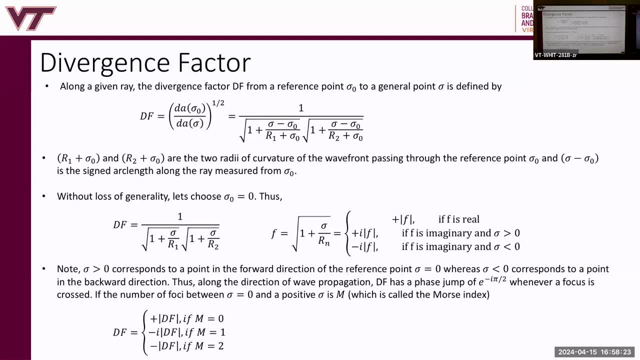 We'll look at examples right now of that. All right, That's the whole point of basically j. either minus i pi over two is a jump of j, uh, or minus j. whenever a focus is crossed, the total number of foci between sigma equal to zero and a positive sigma we call m. 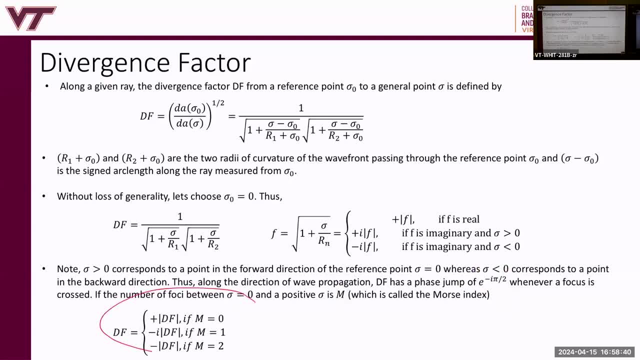 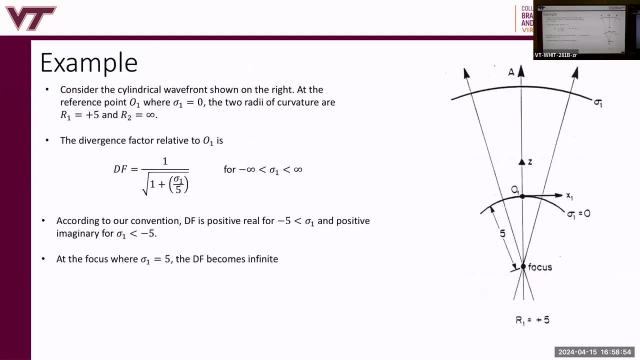 which is called the moore's index, and here are some rules for the sign of the divergence factor and it's um, whether it includes an i or you know i squared, or if you go to two. if you go to two foci, then you're going to pick up two i right, and you get minus. let's do an example. so consider: 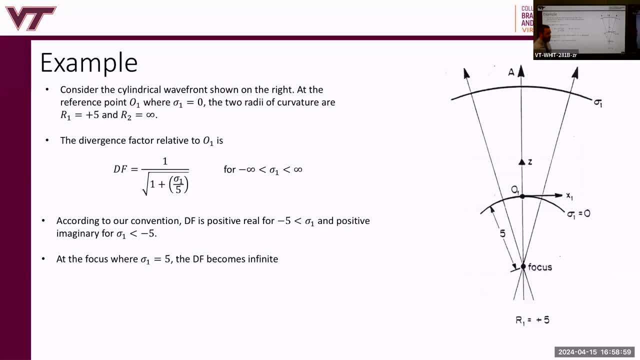 the cylindrical wavefront on the right. if i say cylindrical wavefront, what does that mean? how many? what are my two curvatures? one of them has to be what do you? one of them has to be zero, right, all right. so the one in and out of the board is zero, so you can extend this figure in and out. 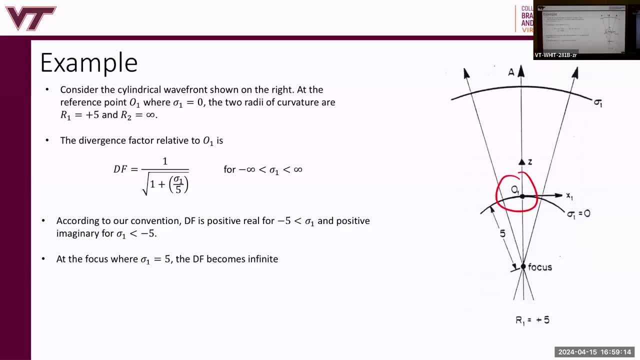 of the board indefinitely, at the reference point, oh one, where sigma one is equal to zero. so the two radial, i have curvature r plus five and infinity. so here's the focus, here's this wavefront passing through, uh, where sigma one, remember, sigma is along the direction of the axial ray. sigma one. 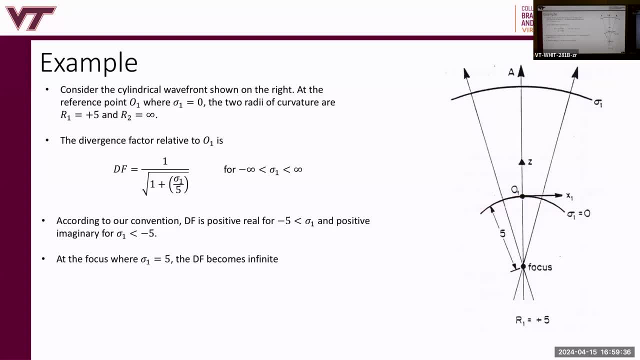 equals to zero at this reference point. that's the origin, and it has a radius of five. the radius of curvature here is five, right, okay, and the other one's infinity. the divergence factor relative to, oh, one is okay. divergence factor equals to one over the square root of one plus sigma one over five. where does 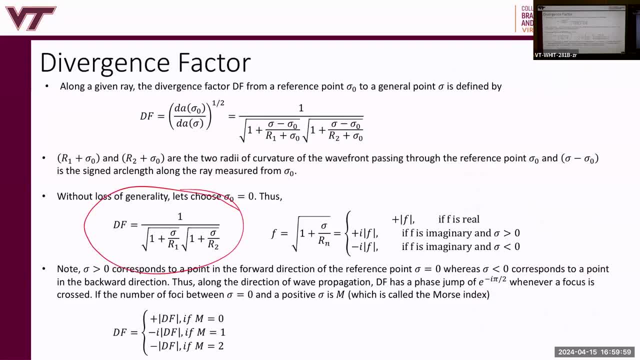 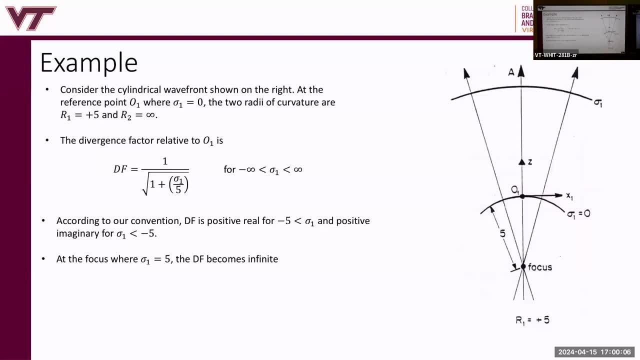 that come from. this is the formula for the divergence factor. why is the other one? why did we only have one square root in this? in this formula here, r2 is infinity. very good, so sigma divided by r1 means sigma divided by five, right, okay? and this is valid for all sigma ones going. 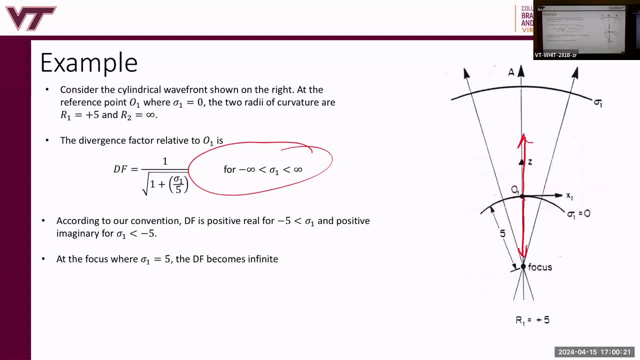 negative or positive, right, all right. so obviously, if i go to, according to the convention, if i go to sigma one less than minus five, so i go sigma one here, i get to my five minus five and then i keep going beyond. that means i go through the focus, right. if i go through the focus, then, uh, this becomes, say, minus six, for example. 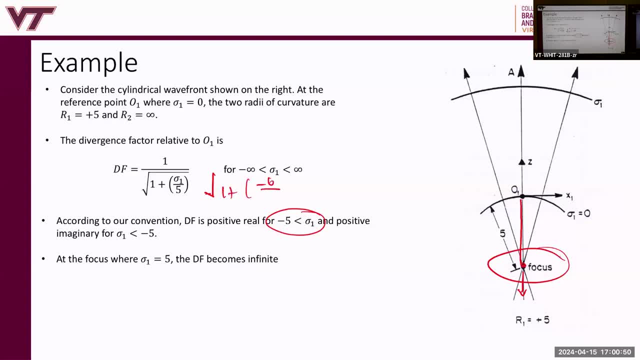 the square root of one plus minus six divided by five, and this you pick up a, i right. so this is going to become, i times, the square root of one. uh, so should be minus six fifths. so, okay, what is one plus minus six fifths minus one fifth? 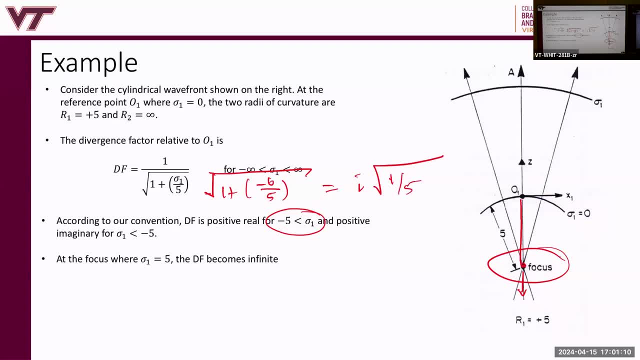 right. so one fifth, all right, good, and we say that that is a positive real for for those values. so, uh, oh, sigma, okay, so, okay, so all right. sorry, what i'm saying here is for, uh, sigma is greater than minus five, so it's more than this focus all. 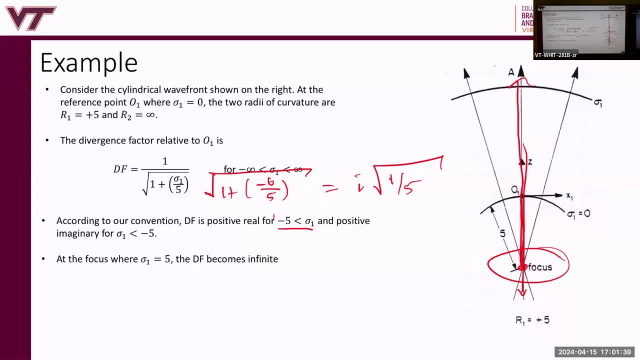 of this right from this focus upward, is my sigma one greater than minus five. we get positive, real, because we don't go through any false high. but uh, for sigma one less than minus five, which is this point and down. then we pick up a. we get positive imaginary, right, okay, good at the focus. for sigma one equals: 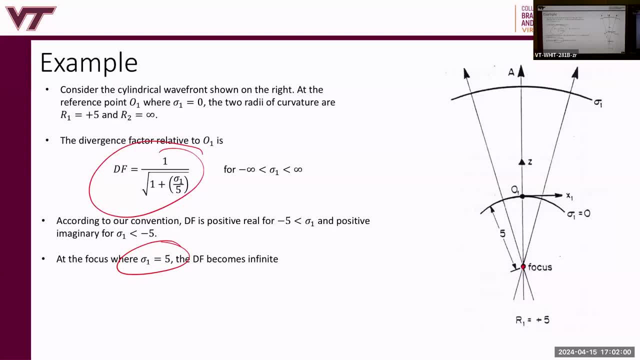 to five, the divergence factor becomes infinite because you divide by zero. and that's one of the limitations of geometrical optics: it predicts infinite amplitude at the false high you, so you can't use it for reflectors right the main beam direction of this, the far field. okay, so this? 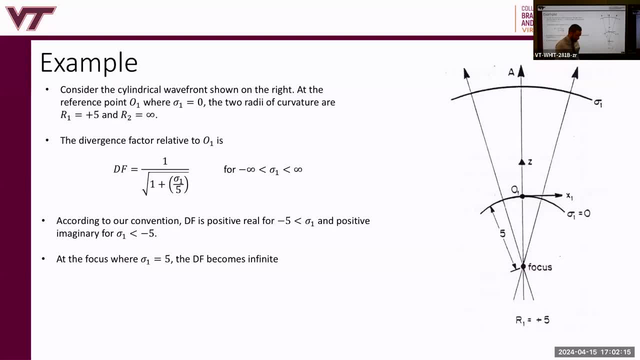 always. this is, uh, one thing that always bothered me when i was a student. so the far field is caustic, all right. so what does that mean? the far field in the direction of the main beam, for example? the far field means all rays intersect in the far field, right, but the rays that go to the far field? 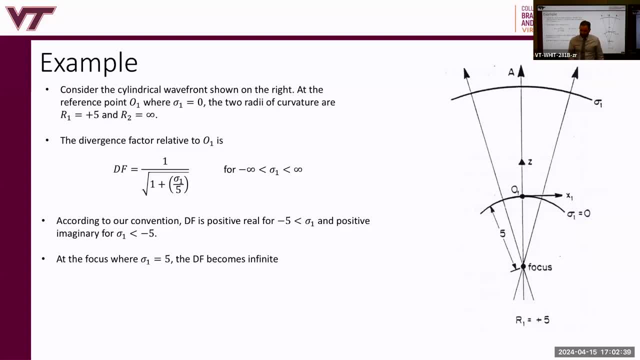 let's say, for example, the far field is the direction of the main beam. for example, the far field is the right direction of the main beam, that we're talking about, the pronног function. so that's a different thing. a ph και for a plane wave are parallel right, but somehow they intersect at. 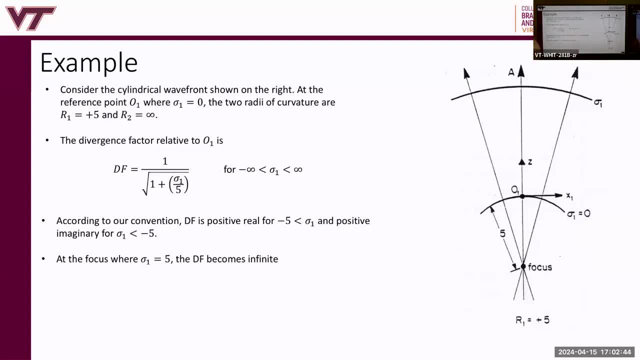 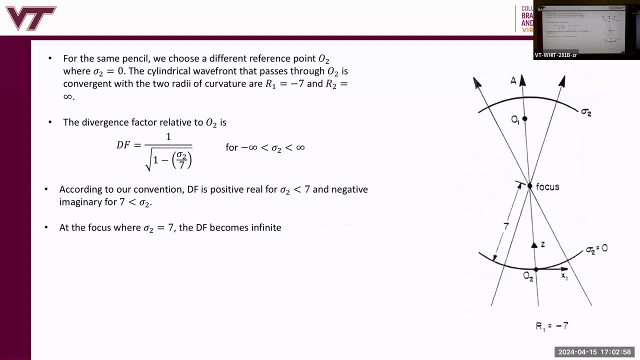 infinity. you can imagine them intersecting at infinity, because if i had a points source infinitely far away, then when i look at the rays near me they look parallel. you're so far away at the source, right? all right, anyway, the far field is caustic, right? yeah, i think it becomes negative. imaginary. uh, where is the denominator of it? and all right, i guess Sana is purely uniqueness, having think about it, not as much relative risen to the new one is son clockwise, but 얘는 to be scared of nuestra θmис dakos, and so on. alright, so we're gonna get off theраф. siempre跑. fried is dead. 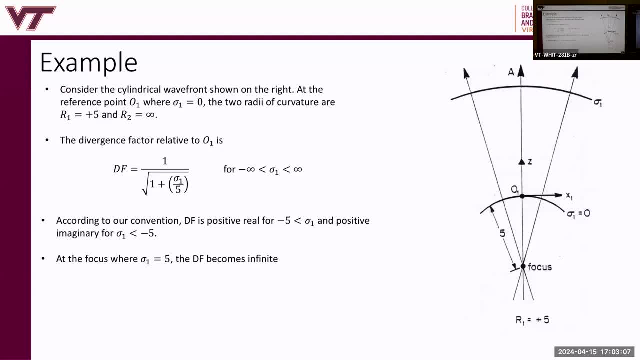 people need matter anyway. we can never change it right. we're out of time here. is this optimization? we're taking aotherapy? okay, by shapes. i don't know, tiziana, when we got here and had like two types of prayer: the denominator, so it's like minus i. okay, let's see what convention we picked here. so 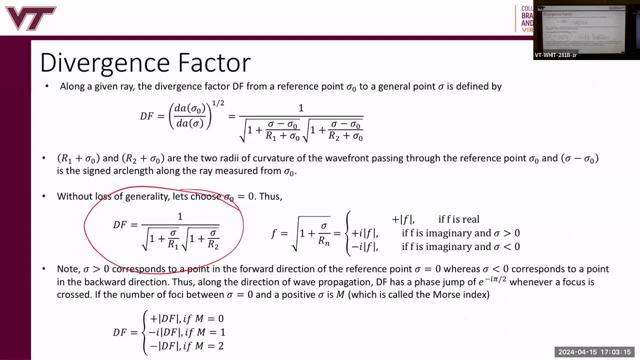 uh, one second, so if okay. so if sigma is less than zero, it's this case, right? if sigma is less than zero, then uh, it should be minus. i times that. but then the minus- i in the denominator becomes a plus. i uh, why is that? that's kind of weird, right? what's a convention? 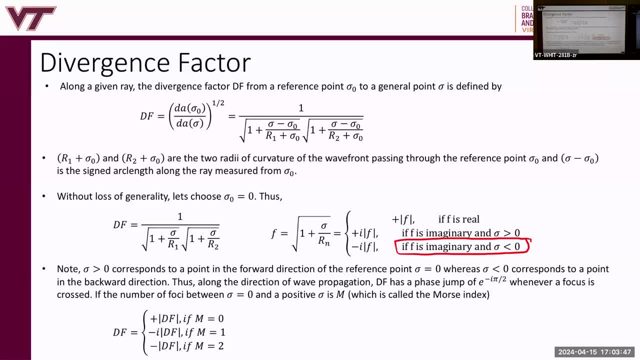 uh, wait, a minute. minus i, no, no, so okay. so one divided by the square root of one plus minus six over five. right, that becomes one, two, three divided by: i times the square root of one-fifth. yeah, this becomes minus. i times one over the square root of one-fifth, which is equal to minus. i times the magnitude of f. 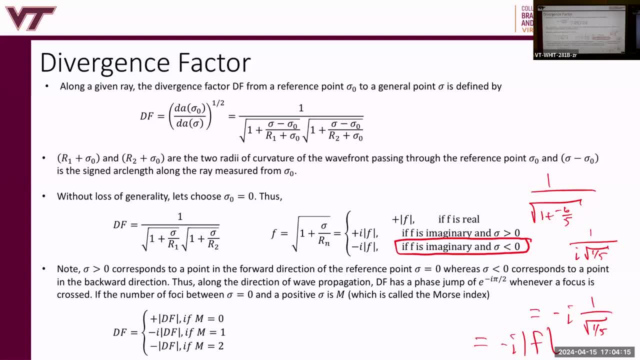 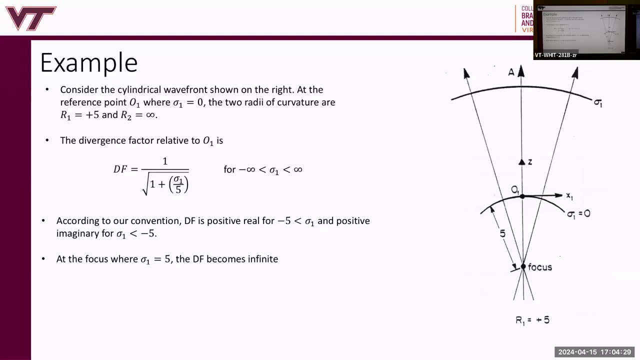 yeah, i mean minus, i right. so that makes sense, right, and on the other slide we said it was positive i, so i think positive, positive imagine is correct. so i got to go back and look at that. it must be something we're not understanding. it's a good point. sigma is less than it's negative. 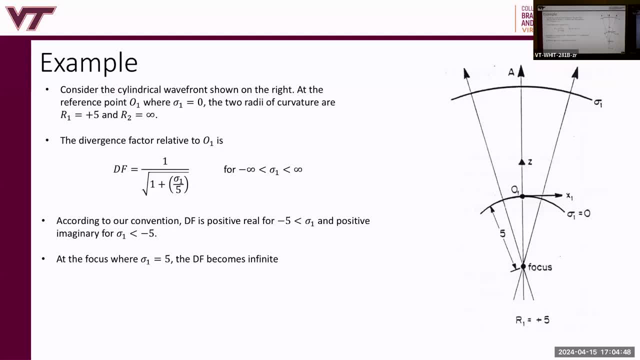 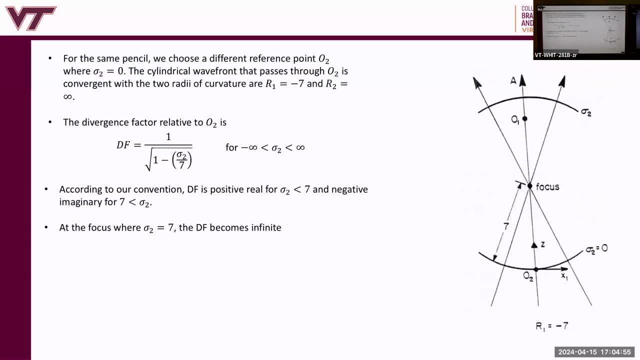 i'll have to look at that. yeah, i think maybe we pick up a minus sign for the convention. yeah, that could be that. yeah, all right, let's look at the same pencil. but we choose a new reference point, o2, so we're going to look at the original. so here's o1 original, here's the original focus. but now we're going to talk. 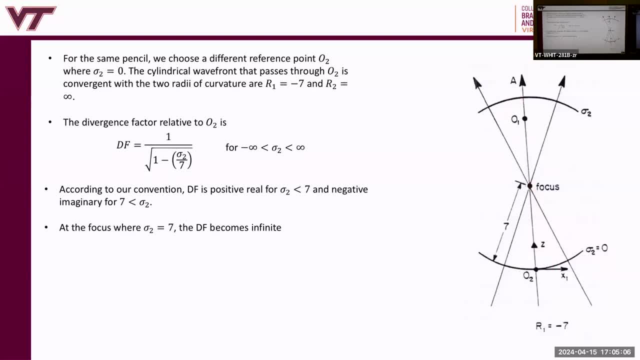 about o2, which is after the focus, right in the backward direction, where sigma 2 is now equal to zero, right. so this is the new reference point where, in this coordinate system, sigma 2 is equal to zero on that wavefront, the cylindrical wavefront that passes through o2 is convergent. 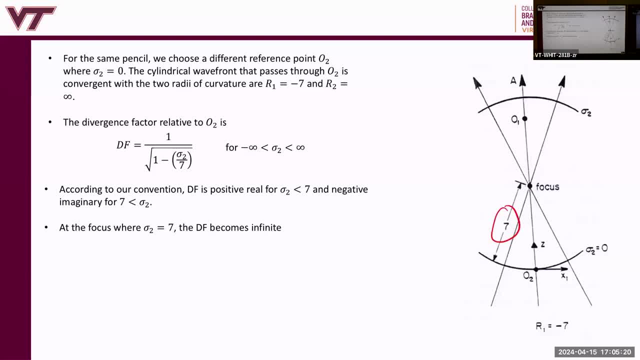 with the two radii at curvature, r1 equal to minus seven and r2 equal to infinite. so this wavefront is converging to the focus. after it diverges, right, okay, the divergence factor relative to o2. now is this expression here and according to our convention, 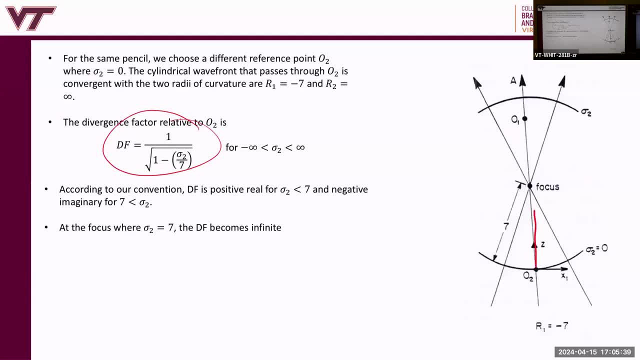 the divergence factor for positive sigma. so sigma less than minus or less than seven. so sigma is positive in this direction. but before we get to the focus, we're allowed z going from zero to seven. right, and that's positive, real. we haven't gone through a foci or focus and negative imaginary. 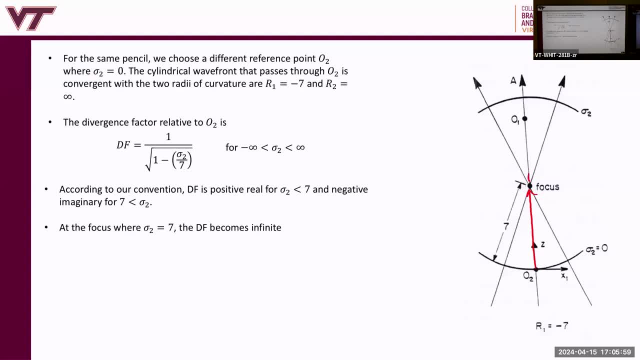 for when we go through the focus, we're allowed to get to the focus and that's positive, real. we're allowed to get to the focus, sigma two greater than seven. then we go through the focus, we pick up an eye right, so it's negative, imaginary, in this case by convention. all right, yeah, just just note. 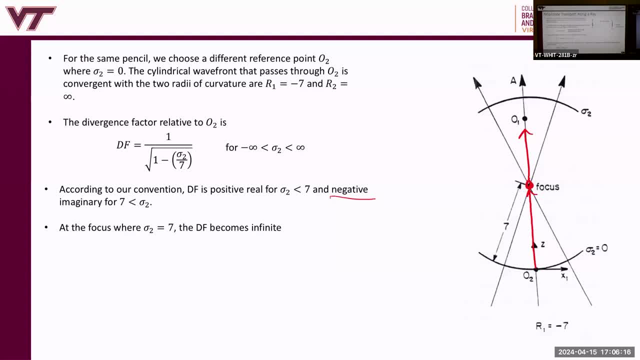 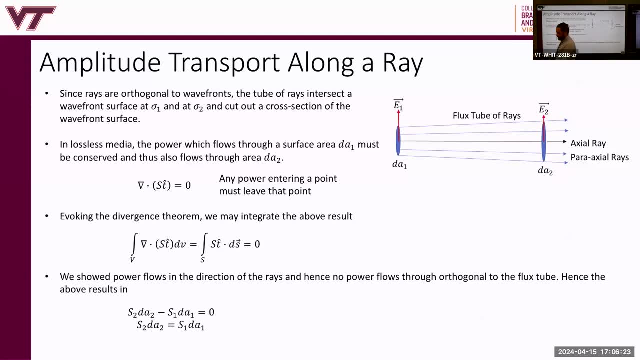 the convention. okay, good, so now, all right. good, so now we're going to rigorously solve the transport equation. all right, to show that the divergence factor multiplied by the electric field at some point on the ray is equal to the electric field at a new point. right, okay? so, uh, and this gets a little bit mathematical, but not too bad. so let's get into. 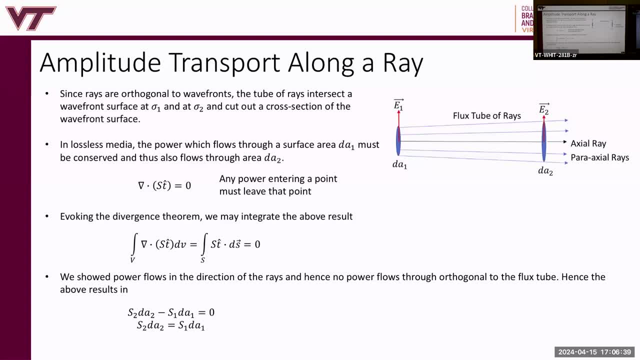 and we'll come back to this point next time too. right? so since rays are orthogonal to wavefronts, the tube of rays intersect wavefront surfaces at sigma one and sigma two and cut out cross section of the wavefront surfaces da1 and da2. all right, in lossless media, the power which flows. 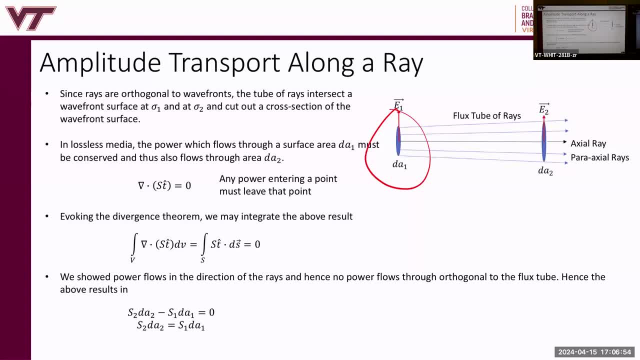 through the surface area, da1 must be conserved and thus also flows to da2 make sense. very good, so in other words, we can say that mathematically, as the divergence of s and the t hat is equal to zero, where s now capital, s is the power density. all right, so the divergence, the, 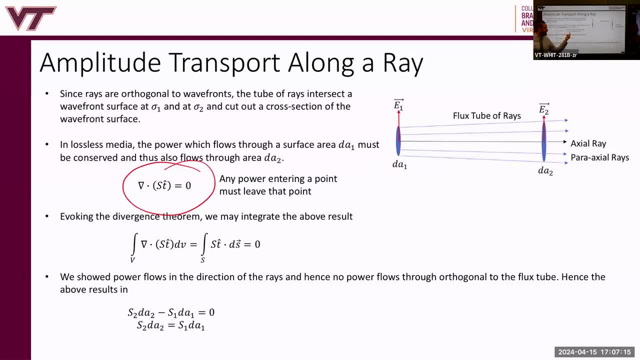 power flowing through some point. any power entering a point must leave that point right. if the, if the function has zero divergence and there's no source or sink of the power or the power density at any point. right, so the power density is what's carrying power. all right, this is the pointing flux, or the pointing 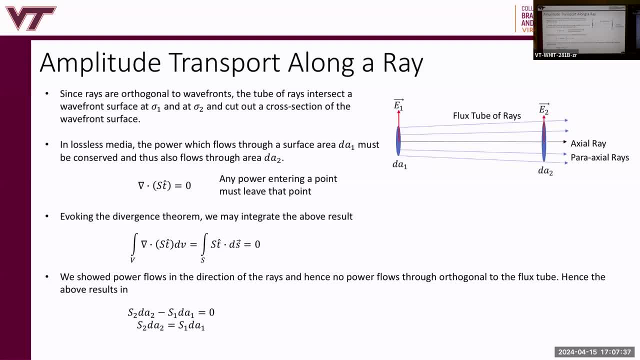 vector is carrying power. what's that? yeah, this is pointing. good, so let's invoke the divergence theorem. we're going to integrate over the surface area of the flux tube of rays. so first we're going to talk about integrating the power throughout a volume, the divergence of power throughout the. 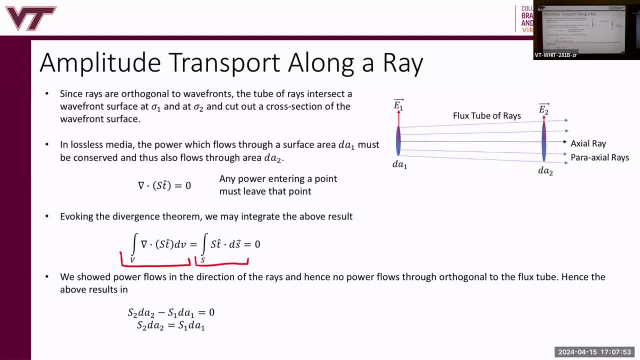 volume. we use divergence theorem to calculate the power density- uh, i guess the power here, in this case leaving the uh sides of the flux tube, right? okay, so we showed that the power flow is in the direction of the rays, right? that was one of our conclusions, and hence no power flow is orthogonal to the flux. 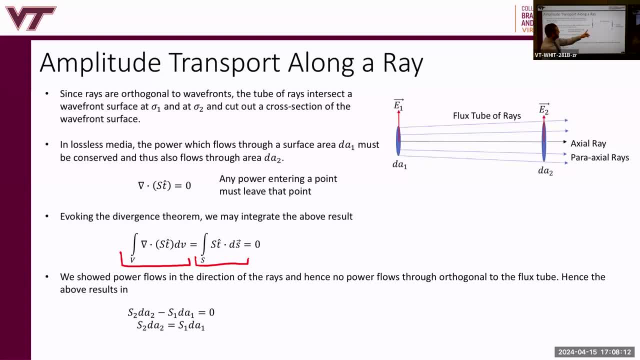 tube. hence the above results in the difference in the power leaving this surface area, da2, and power entering surface area da1- right, and that's the result of this integration being equal to zero. so we can say that s2 times da2 has to be equal to. 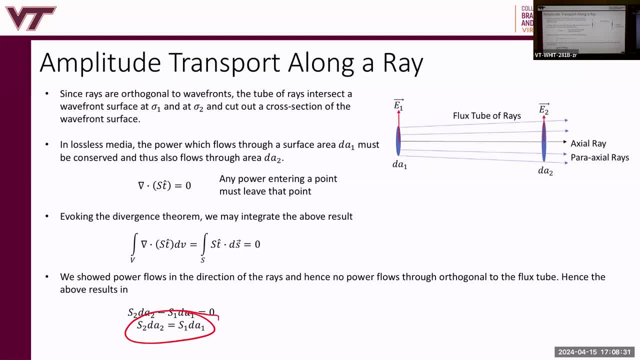 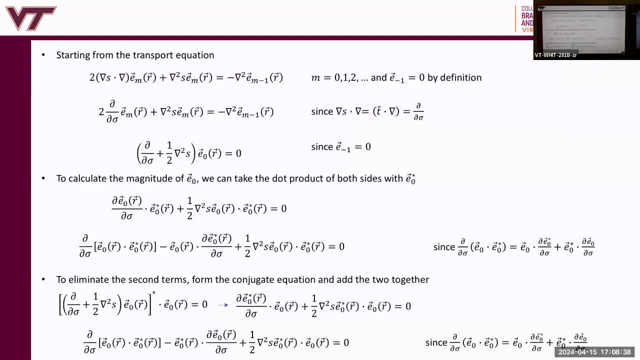 s1 times da1 conserved power in the flux tube of rays. right, very nice. so start with the transport equation. we derived that before. here's the transport equation i've repeated here from our derivation by substituting lunaberg-cline into the wave equation. and okay, so there's some. 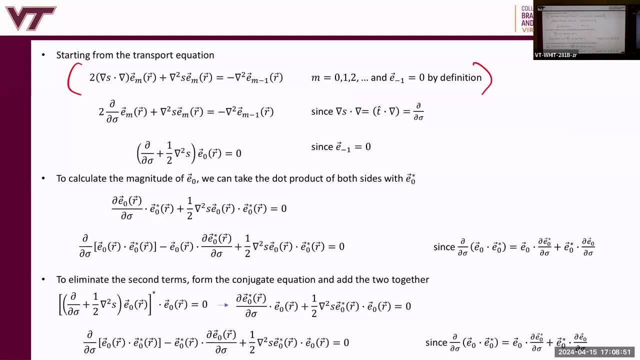 steps here and i've tried to explain them all. so here, gradients of s dot with gradients. we already said that that's equal to partial by partial sigma. so we replace that with partial by partial sigma. that's all we did in that line, all right? next, uh, we know that. e to the minus one we're going to talk. 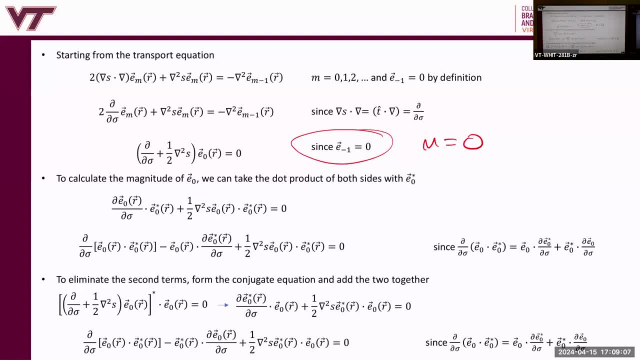 about m equal to zero here. all right, so e to minus one equals to zero. this side goes to zero and we replace these with zeros. we factor it out, so we got this line right. okay, to calculate the magnitude of e naught. we want the magnitude of e naught from this equation which governs. 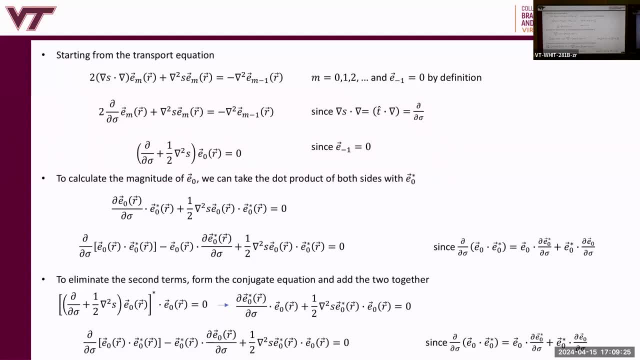 the change in amplitude along a ray. we multiply by e naught conjugate, because e naught conjugate gives us magnitude. e naught squared. that's what we're after, right? okay? so take the dot product: e naught conjugate, both sides. all right, now what we can say here is that partial. 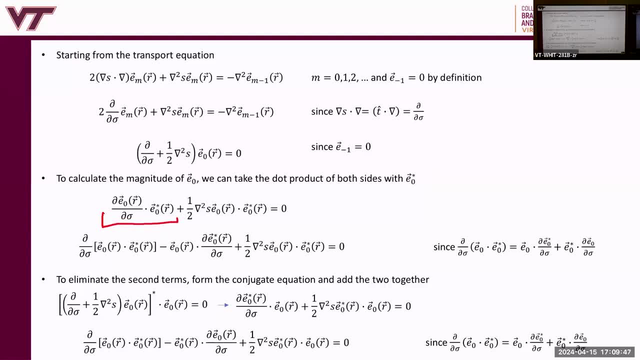 e naught partial sigma dotted with e naught conjugate is this, this term here. and if you differentiate e naught dotted with e naught conjugate with respect to sigma, use the product equation. so this term is equal to this one minus minus this one. all right, and that's what we've done. 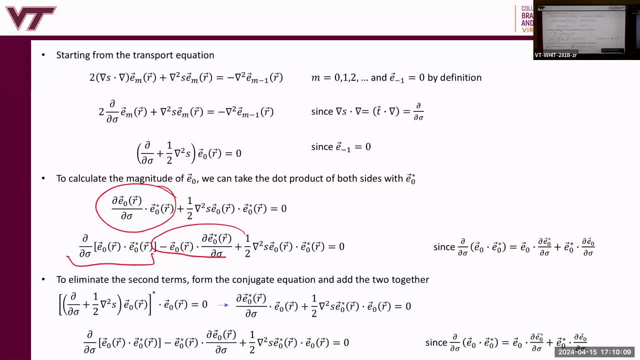 we've replaced this one with this term minus that term. all right, very good. the other term stays the same to eliminate the second term. so we want to get rid of this term, basically to eliminate the second term from form the conjugate equation. add the two together. all right, so let's do that. 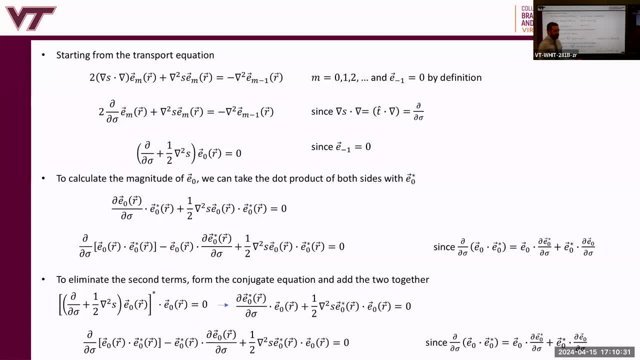 we. this reminds us of what we did the same thing when we calculated what theorem last semester, first lecture- i think that was probably related. yes, it was the conservation theorem, right, conservation of power. we did the same series of steps that we're doing here. so let's, let's conjugate this equation and dot it with e naught now. 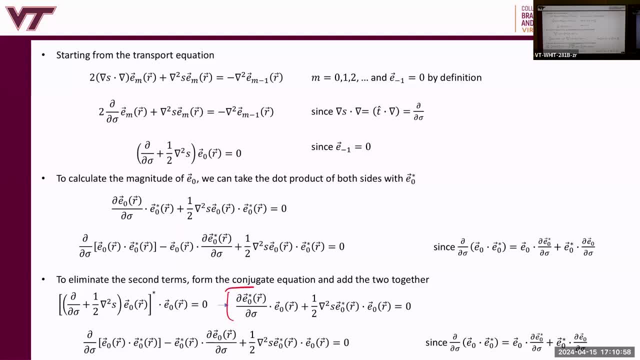 all right. so if you do that, you get the same thing. you get the same thing. you get the same expression, all right, all right, and then we can replace this derivative, which is now this one, with this one, minus this one. all right, so we get this here for that, okay. now we have to add the. 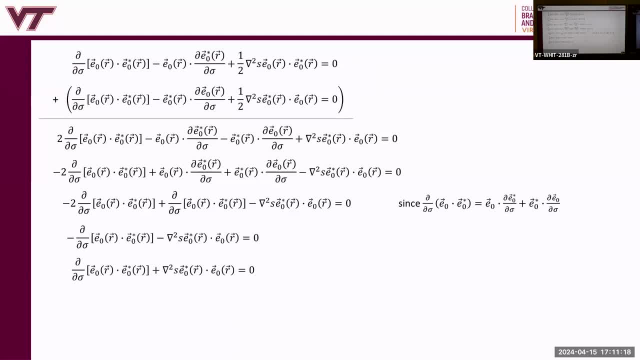 two together. so here's the first one. here's the second one. right, this is like equation one dotted with e- naught, conjugate, and this is the conjugate of equation one dotted with e- naught. right now, we're going to add the two together and we're going to add the two together and we're going to. 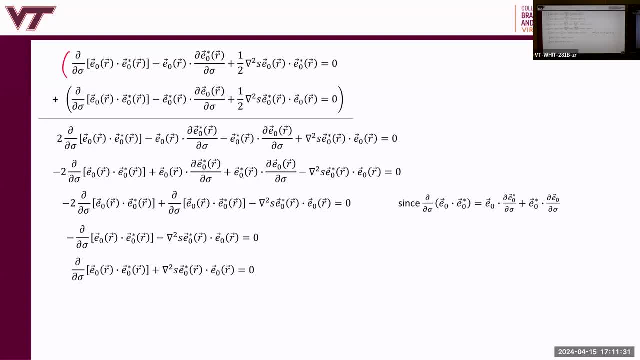 add these two together and what do we get? so this plus this, these are the same, so you get two of those. then you have, uh, this: this term comes from equation one, this term comes from equation two, and then you have two of these which are the same, so you just get this without the one half. 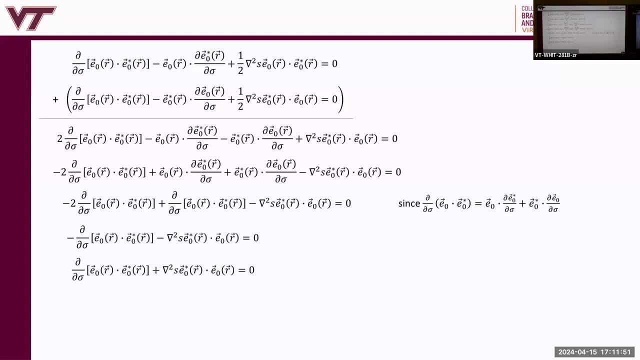 all right, okay, now. what are we going to do? um, the next thing we do is we negate everything, this line. all we did was multiply through by a minus sign. all right, now we'll notice that we have, uh, e naught times partial e naught conjugate, plus e naught conjugate dotted with partial e naught. 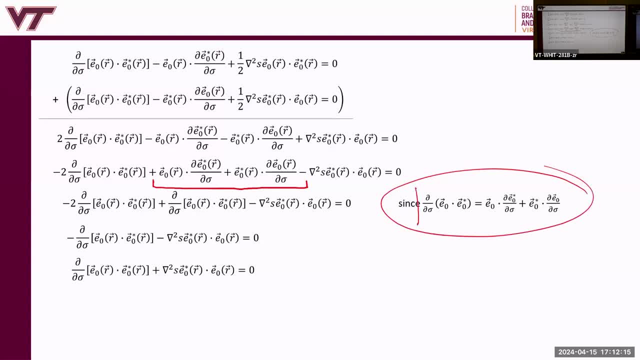 which is nothing but partial, by partial sigma e naught dotted with e naught, conjugate right, okay, so that means that we can replace all that with this. all right, now we have two of these and one of these, and we're going to add the two together, and we're going to add the two together. 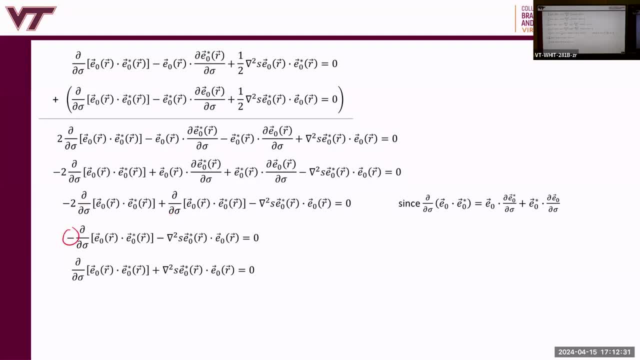 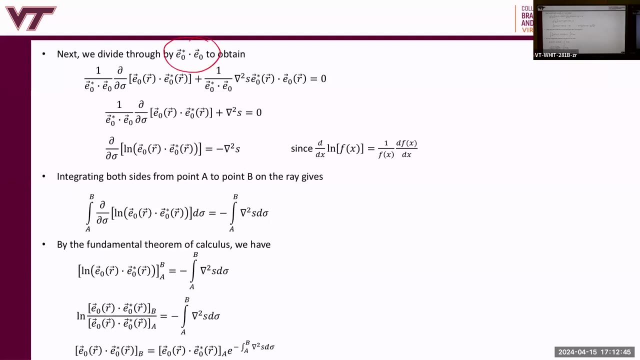 which are the same. so we just get minus one. now, right, and this term stays the same. and then, uh, we multiply through by a negative. again, we arrive here, all right. so this is how we're solving this differential equation, right? okay. next, we divide through by e naught, conjugate dot with e naught. 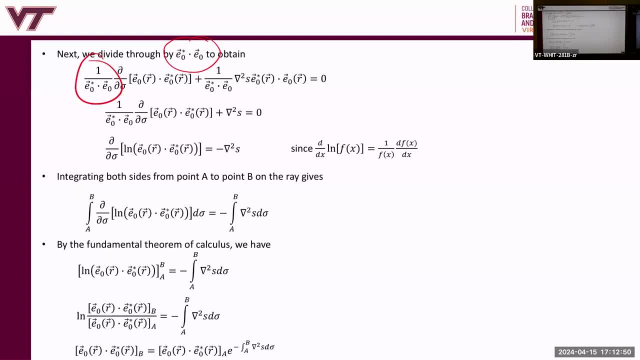 all right. so all i did was divide through by that there and there, right and okay. so this- remember- this term is multiplied by all of this, so these cancel with that. that was the whole point of multiplying by that one over e naught, conjugate dot e naught. all right, now, uh, the next. 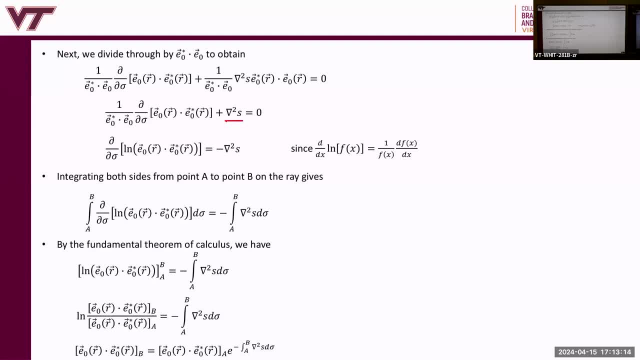 thing we do. so that means it gets rid of this. so now we just have that. on the second term. yeah, so if you differentiate d by dx, ln of f of x by the chain rule, you get one over f of x by the derivative of the natural logs multiplied by the derivative of the inside, which is partial. 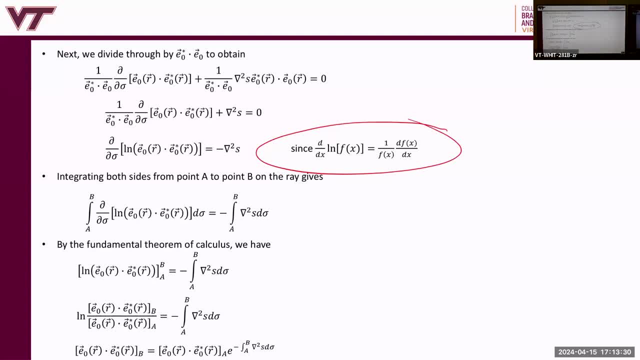 or df, dx, right, okay, so use that to convert this one over x, multiplied by partial of f of x, into the derivative of the natural log, and then throw this to the other side. all right, so we're at this point now. now what we need to do is we need to integrate both sides, from point a on array to point b. 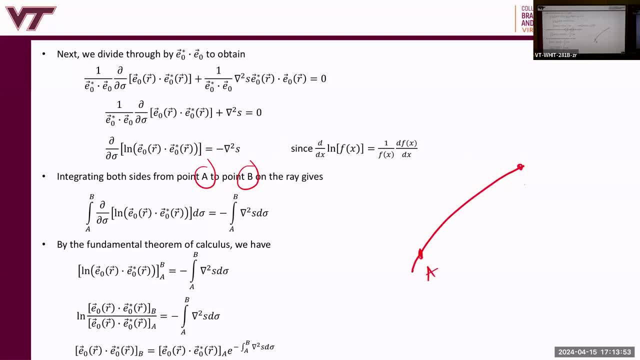 so there's some point here. a, another point b: we want to calculate e at a and you e at b. okay, i drew this curved, but it's not a curved line, it's a straight line. all right, okay, so integrate both sides, from a to b and uh, by the fundamental theorem of calculus. now the left. 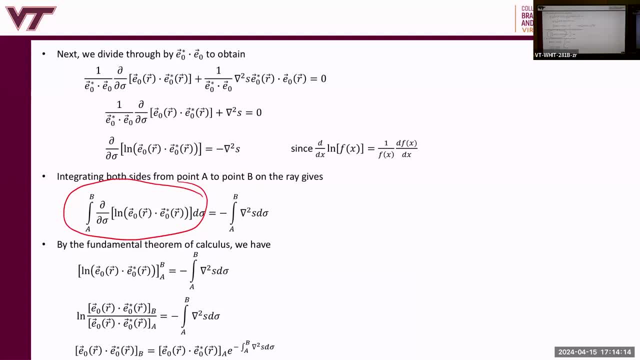 hand side becomes: uh, so this is just like f of x, right. and then we, we divide or we evaluate at b minus a, so both first and second fundamental theorem, i think all right. and then uh, so we get ln there right, so ln of f of x by the fundamental theorem of calculus. now the left hand side becomes: 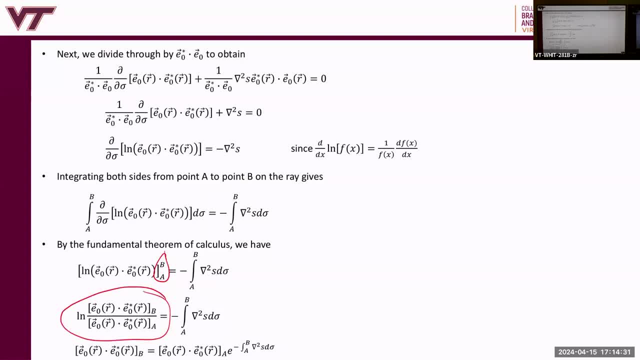 ln of b minus ln of a is nothing but ln of b divided by a. yeah, and then we raise e to both sides to get rid of this natural log. and now we have a product of the magnitude of the electric field at point b is equal to the magnitude of the electric field at point a, multiplied by e to the. 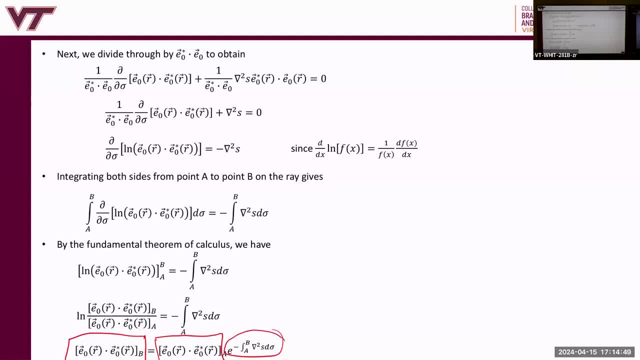 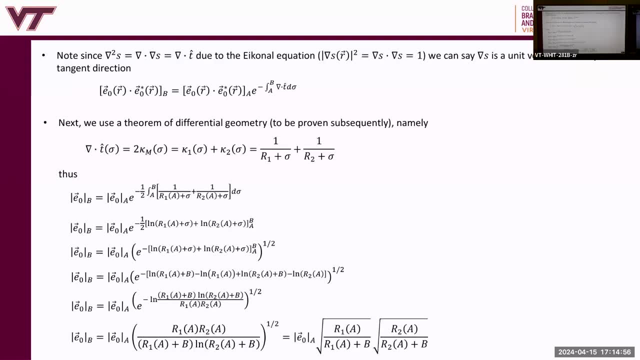 minus integral of from a to b of del squared, s d sigma. okay, all right, so the conclusion is coming very soon here, let's, let's, stop here. i don't want to, i don't want to rush it. all right, we're almost there, though. where we're going to get to is after this slide. we get to here, and we find that the 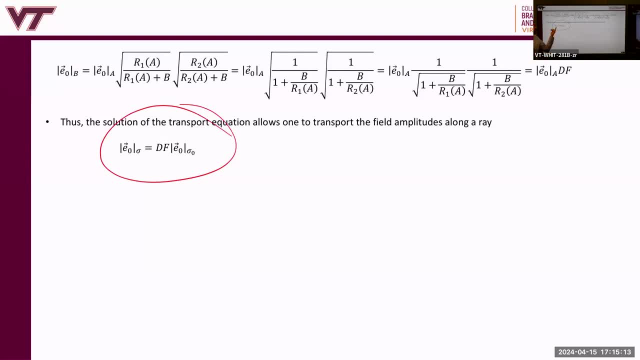 electric field at point sigma not is equal to, or the electric field at a point sigma on a ray is equal to the electric field magnitude, the electrical magnitude at a point sigma not on the ray, multiplied by this divergence factor, and we're going to derive this divergence factor. 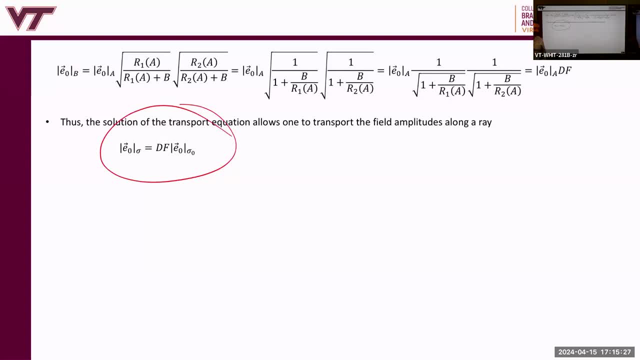 naturally, by solving that transport equation and calculating the integral of e to the minus, or e to the minus, integral from a to b of l squared of s times d sigma that's going to become this right, the divergence factor will pop out of there. we've already noticed that the divergence 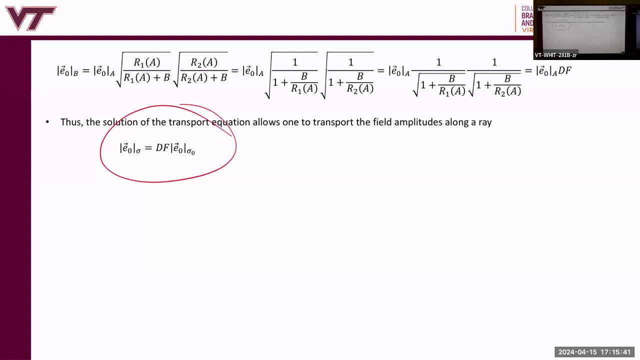 factor. uh, we derived it geometrically. here, we derive it from the differential equations, Maxwell's equations. all right, okay, very good. okay, so a lot of math, right. but we're gonna get to the fun stuff, where all we need is the final results of all these. we're solving differential equations. 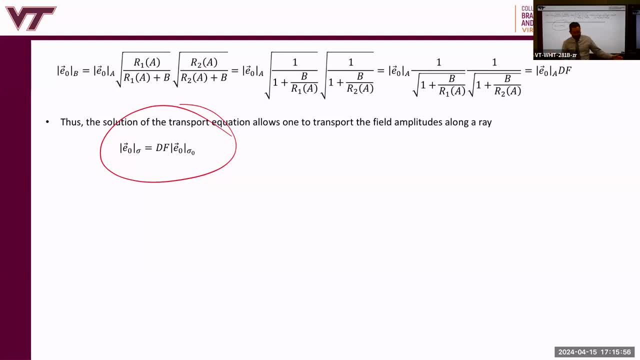 remember last semester we solved the wave equation and cylindrical coordinates, spherical coordinates and there was a bunch of steps, separation of variables- but we need to understand steps and we need to see them once in our lives, but we just use the final results. so we're going to do here. 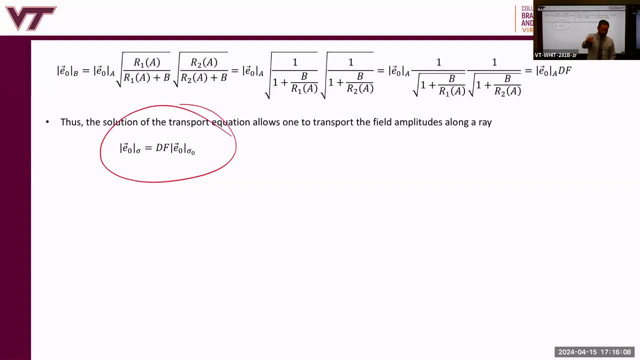 we're going to use this final result here and tracing the rays, uh, the phase along the ray, and you're basically done then right, you know how to calculate the amplitude along the ray and the phase. now we just have to learn how to calculate the reflected q matrix, and then we'll be done.